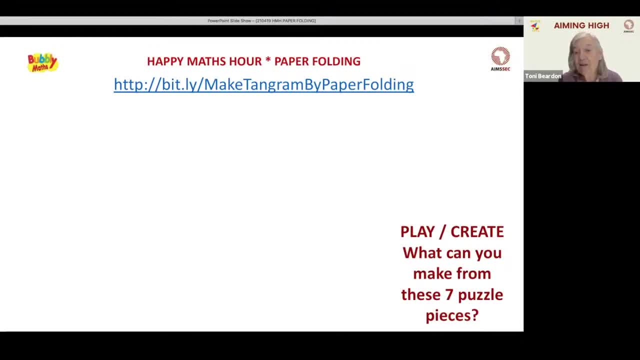 creative And this puzzle has seven pieces And Caroline's going to show you how to make the puzzle And we're going to talk about some of the many things you can do with this puzzle. There you have the puzzle used in our logo for Mass Toys to make that little sailing boat. 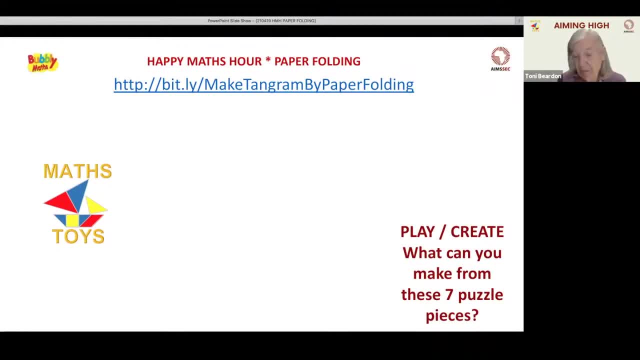 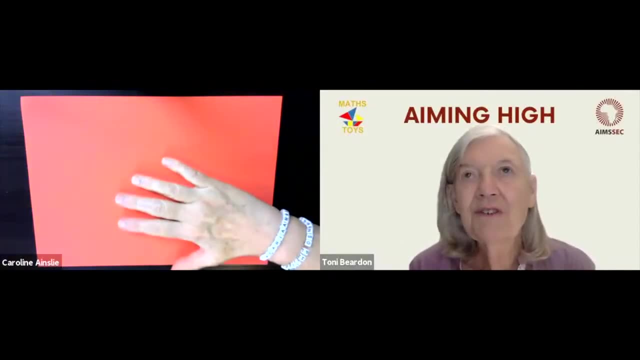 Mass Toys is the YouTube channel, And here you have the square with the time-gram puzzle in it and a symmetrical shape which we'll discuss later. So we have these. This is an ordinary piece of paper And she's going to do some folding. 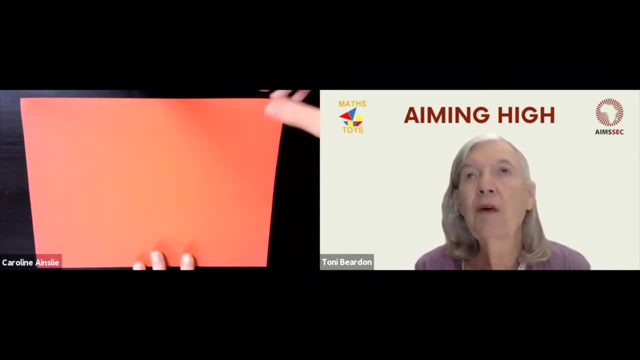 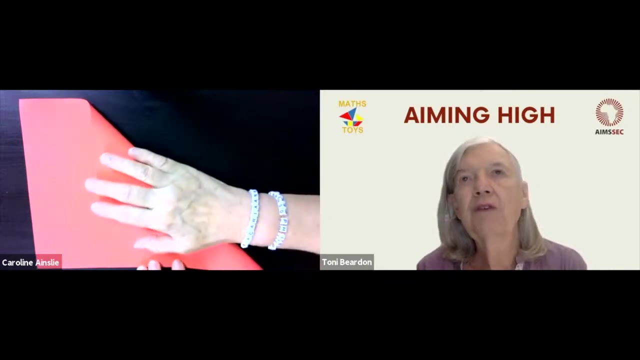 So you need to fold one corner to the fold it right back so that the two edges go together And you make that into an angle of 45 degrees. And there you go. Those two edges should go together. Fold should go through the corner. 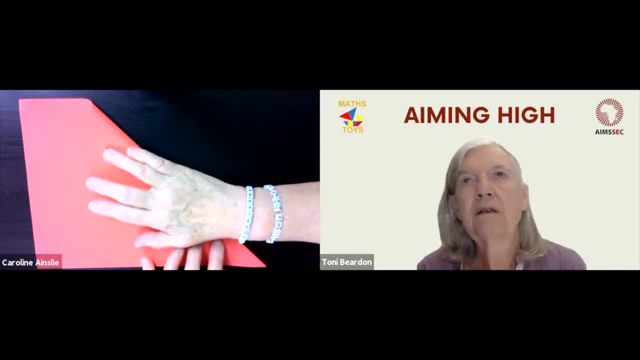 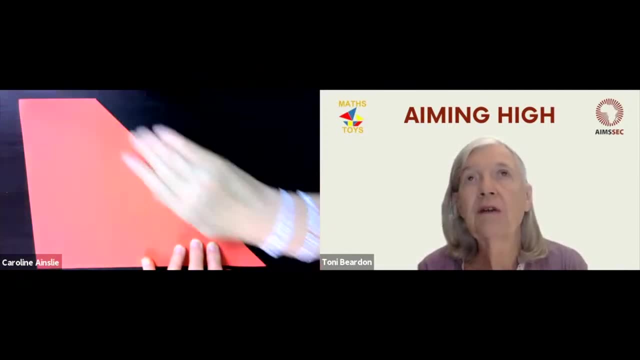 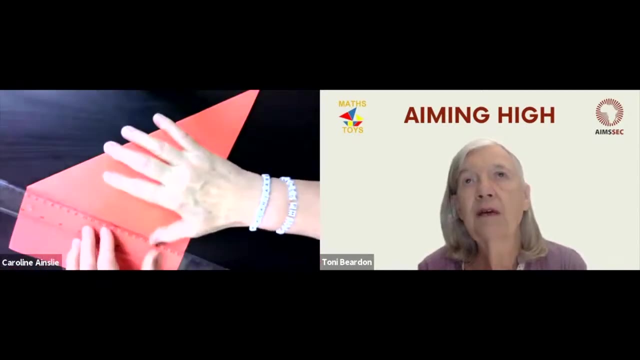 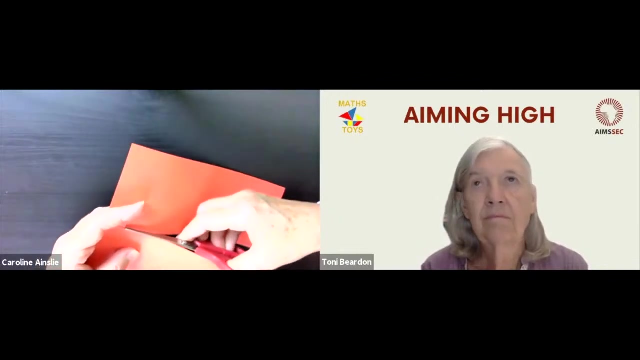 And crease it down Along the fold, And the reason that we're doing that is to get a square. So Caroline needs to cut off that edge of the paper and she'll be left with a square when she opens it out. I have found these days that not every child knows how to make a square from a piece of paper. 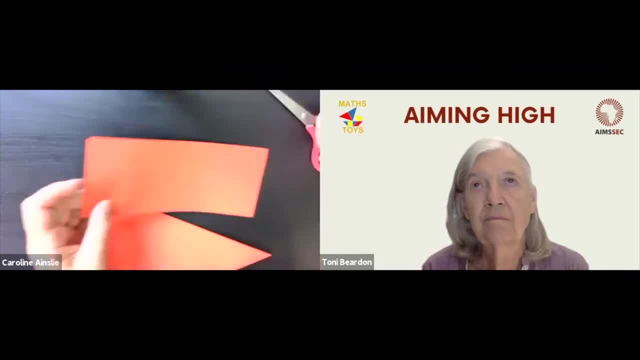 And it works with any piece of paper, Because all you have to do is then fold it over And that gives you a square. That's under there, And now Caroline's opened out her piece of paper and she's got one diagonal in that square. 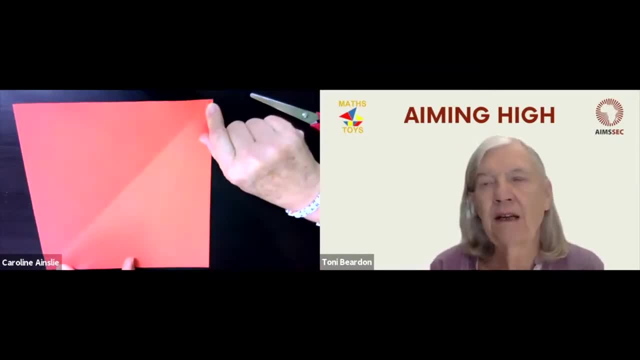 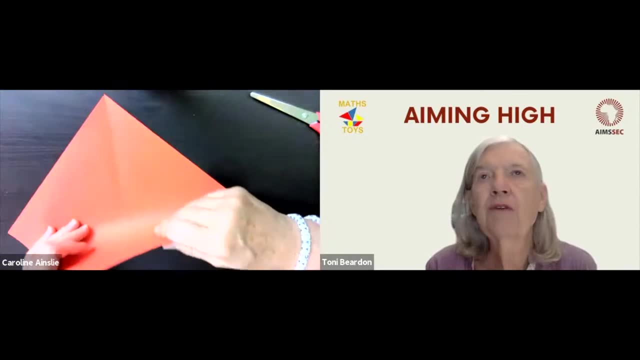 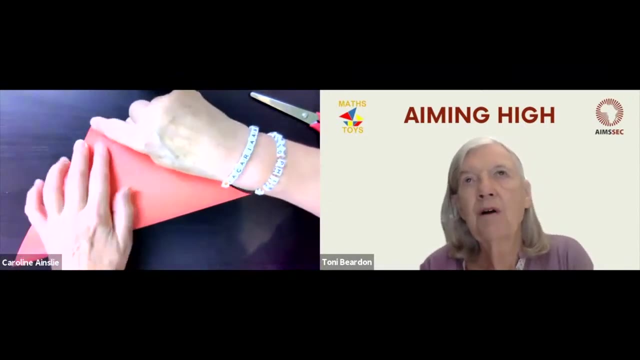 Now the next thing is to find the centre, But not to crease it down as right across, But just to put the other two corners together And just to flatten it slightly in the middle there So she can mark the centre. We need that centre point. 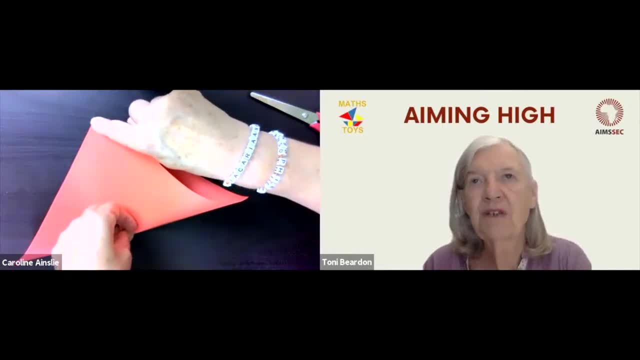 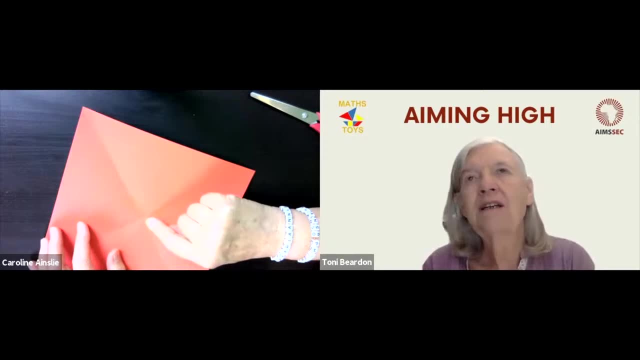 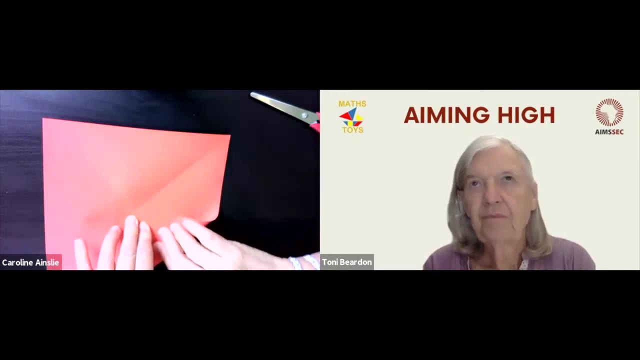 There we go. So she's making sure she knows exactly where the centre is there, Opening it out now. Now she's going to take the bottom right hand corner and fold it up to the centre And crease that. Now, that smaller triangle. there is one of the triangles of our seven pieces for the table. 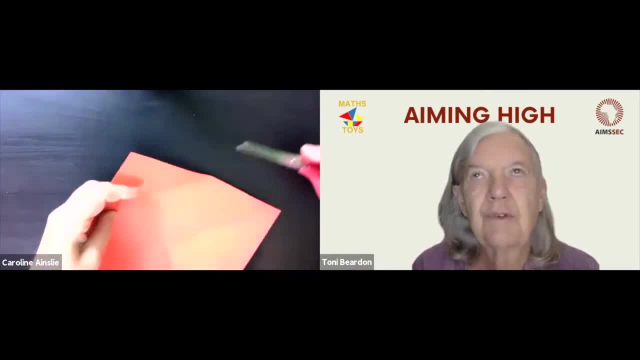 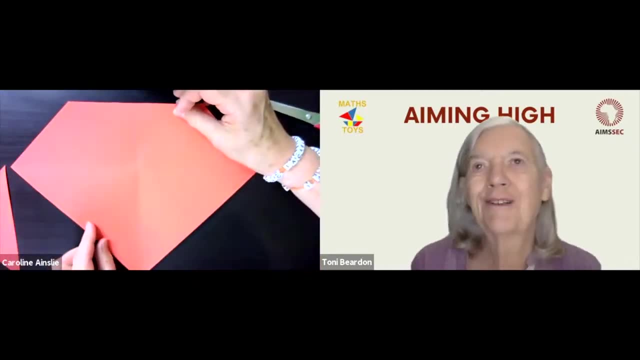 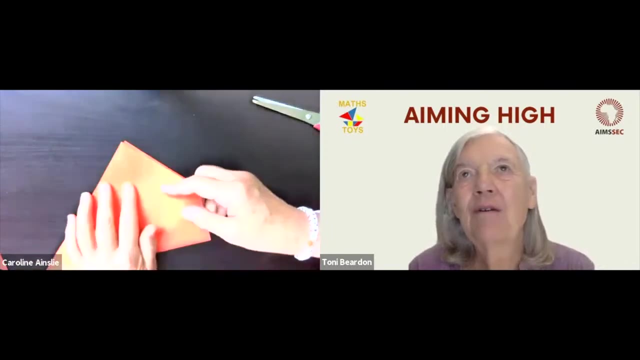 So Caroline's going to cut that off Now. the reason she didn't crease it across was she didn't want to crease the triangle that she's just taken off. So she's now going to go back and fold that, Because now that's not going to matter anymore. 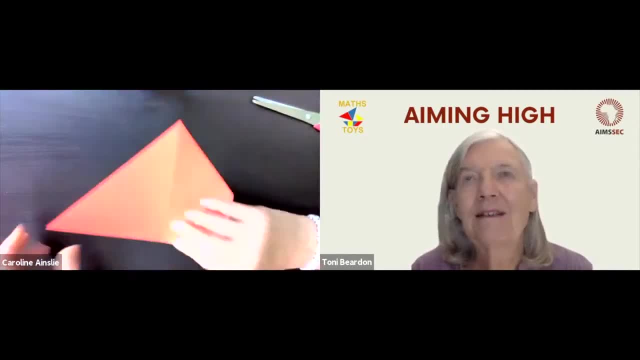 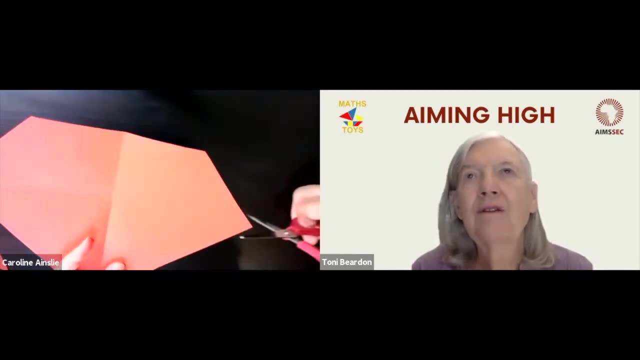 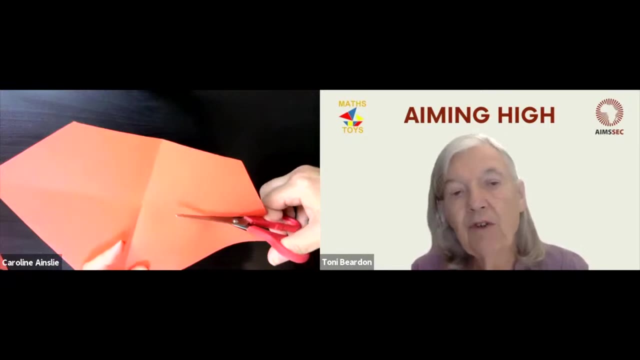 We actually want this fold. This fold will be cut by the time we're done. Yes, Now then she's going to cut that long diagonal now And those two pieces, those two triangles. There's going to be five triangles here. 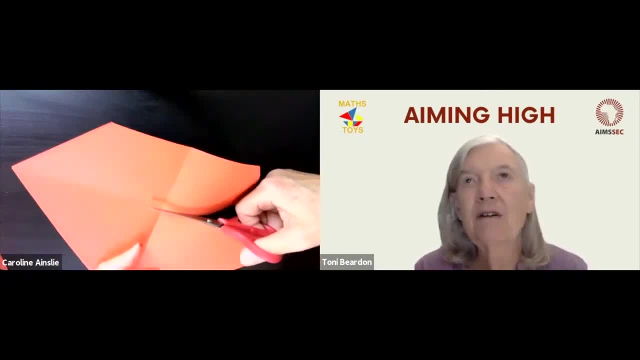 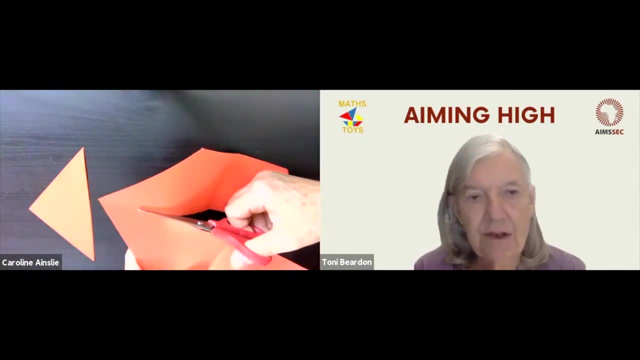 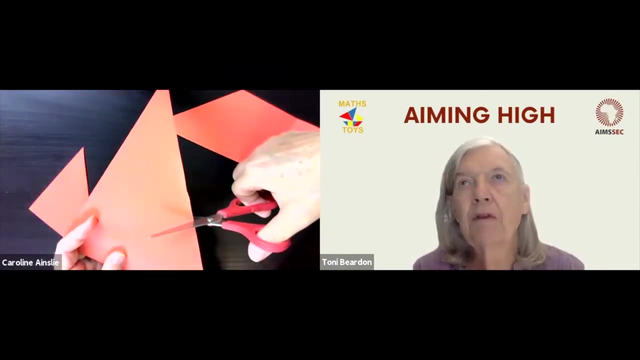 We've just taken off one of the middle sides. Caroline's now cutting the two larger triangles And she's cut them off. She's going to be left with a strip. I was so excited to discover you can actually make your own tangram. 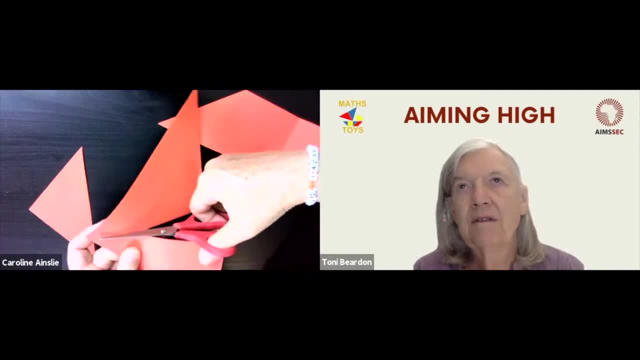 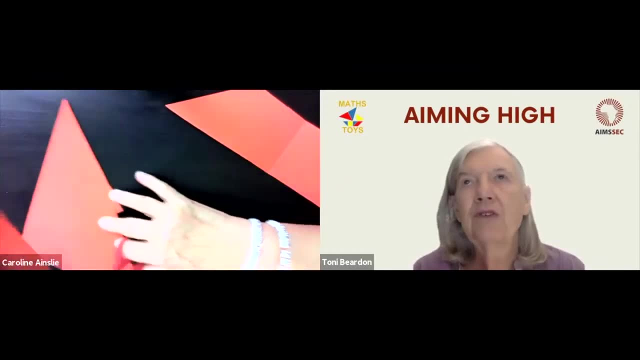 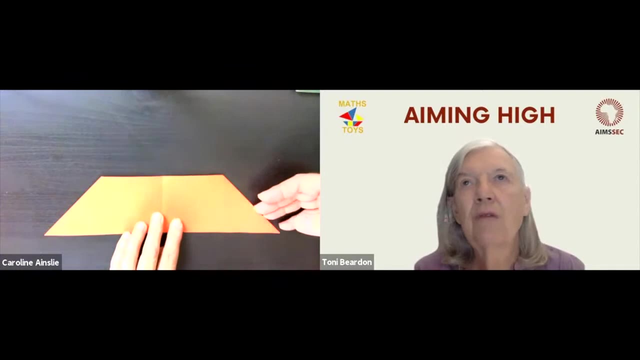 I couldn't believe it when Tony told me So simply and beautifully: There you go. Now then the strip. The first and obvious thing to do is to take the triangle, one of the triangles, fold the corner. Sorry, it's a trapezium, isn't it? 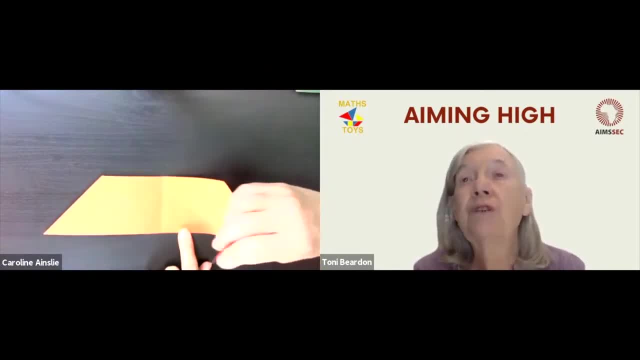 But the one with the corners there And fold it to the centre. So you've got a triangle and a square on that side of the centre And Caroline's going to cut off that smaller triangle now and the square. Now she's left with another trapezium. 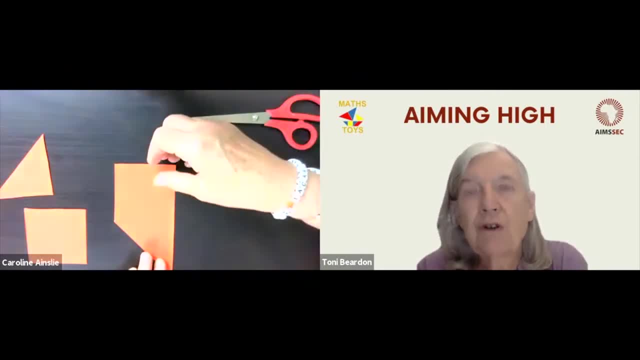 But this time she's going to fold it so that she's got a parallelogram and a triangle. So I'm actually going to fold through the square rather than make the square. Yes, So you see, she's now shaped. now It looks as a parallelogram. 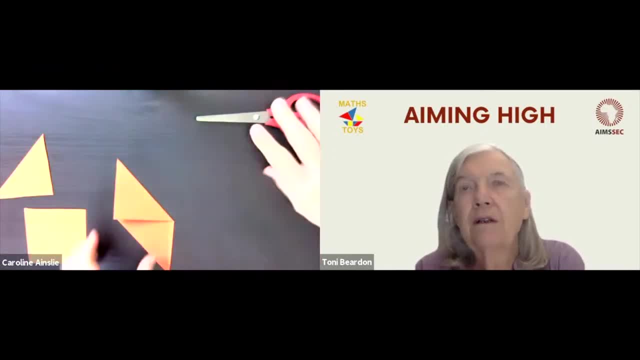 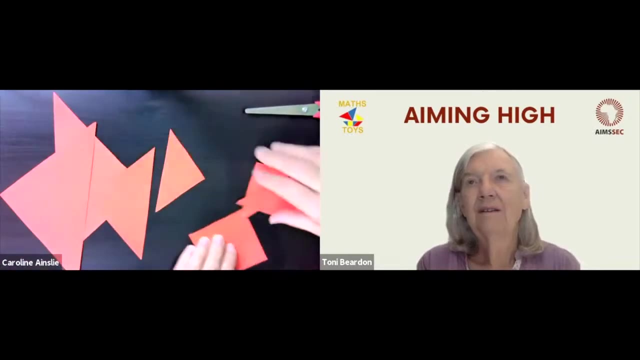 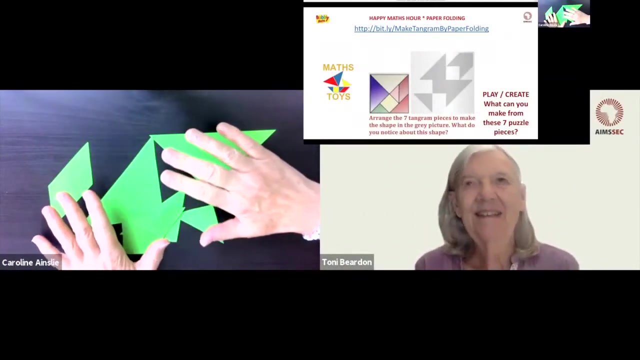 And she's going to cut off that triangle And she will have then the seven pieces. Here's my seven pieces: Two big triangles, One smaller one, Two small ones, A square and a parallelogram. I've now got to make that grey. 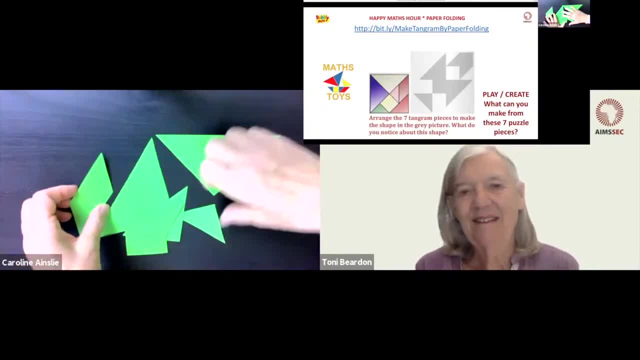 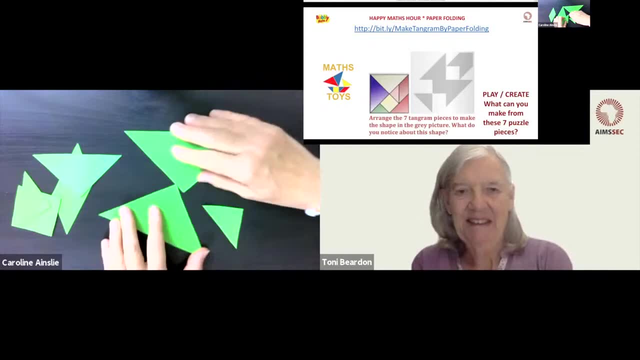 It could be a kind of a fancy rocket as well, couldn't it? Or a fancy airplane. Right, let's see I'm going to use. Yeah, I'm going to start off with what looks obvious to me. It's the two big wings. 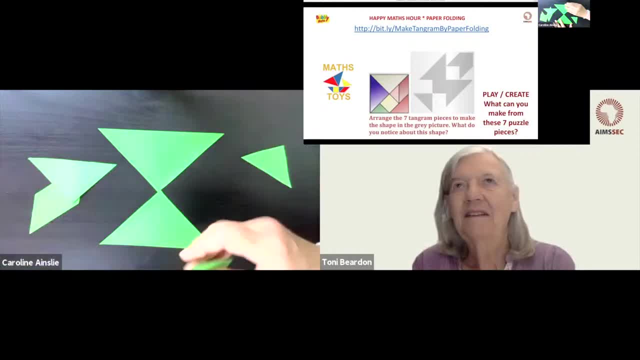 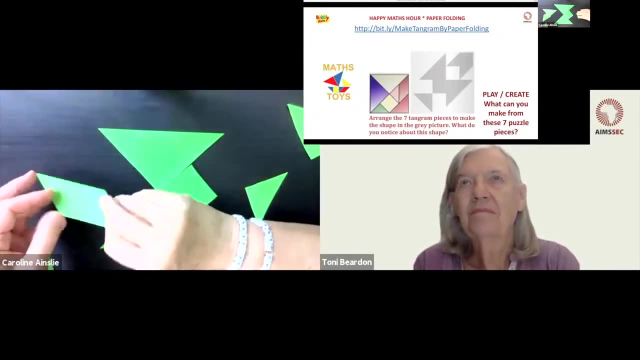 And then I think that I think that there is a square. We'll make that, Let's hope. And then perhaps Let's see, The parallelogram has to be making. Oh look there, That's going to make a square there, if I put that there. 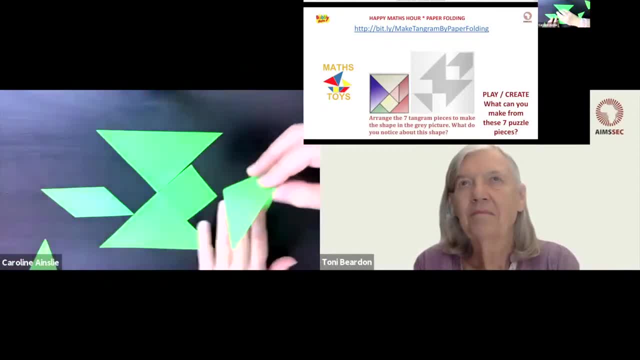 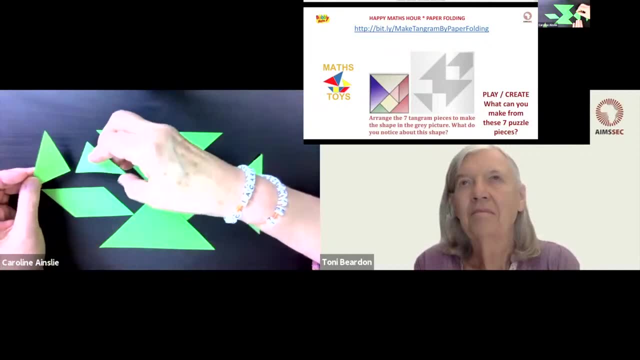 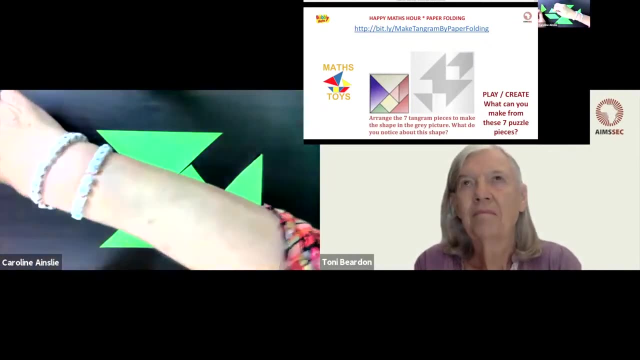 And will that? Oh, that triangle's too big, So that must be this one down here And now, with these two remaining triangles that I have to make, Is that going to work there? And then, how do I make this last one? 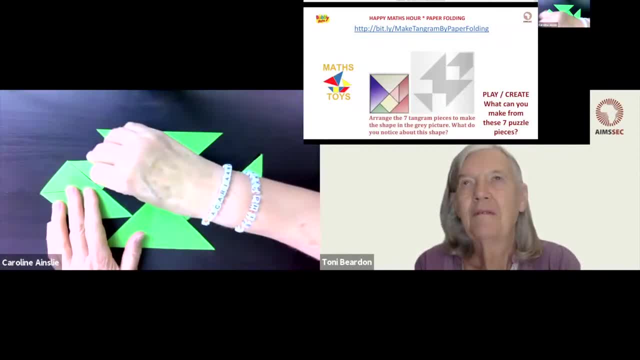 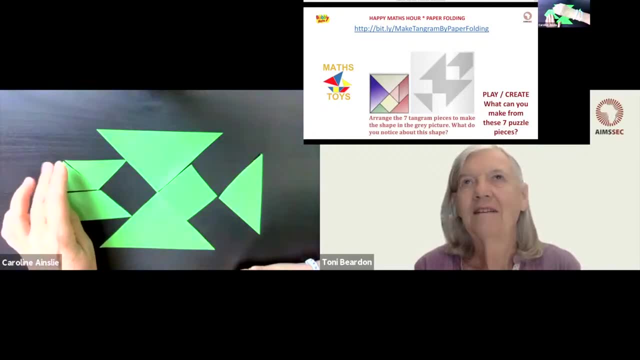 Is that? Oh, I did it this time. I've done this a few times and I've struggled to do this bit, But what I love to see here is that these two triangles, which we kind of know because of the way we cut it. 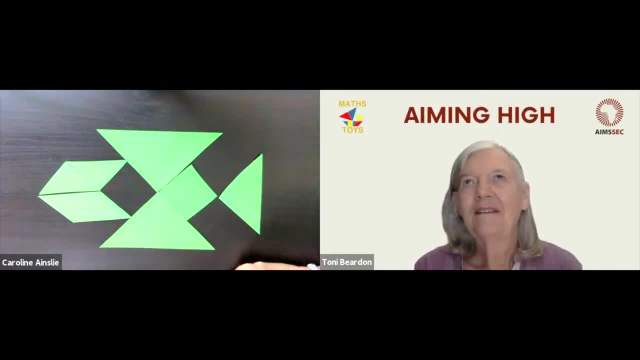 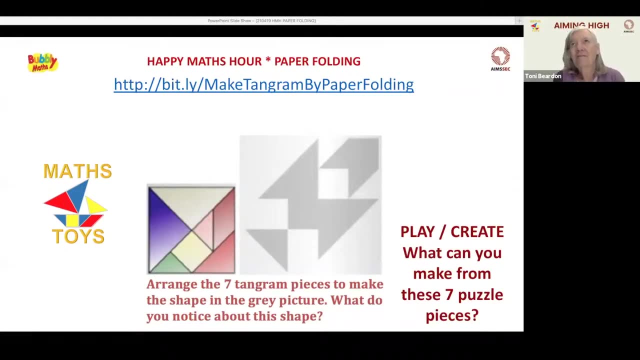 make a parallelogram, Which I really liked. So this is just one of hundreds, many hundreds of different forms that you can Creatures, if you like, that you can make with the tangram pieces. It's an old Chinese puzzle and there are many, many ways that you can play with it. 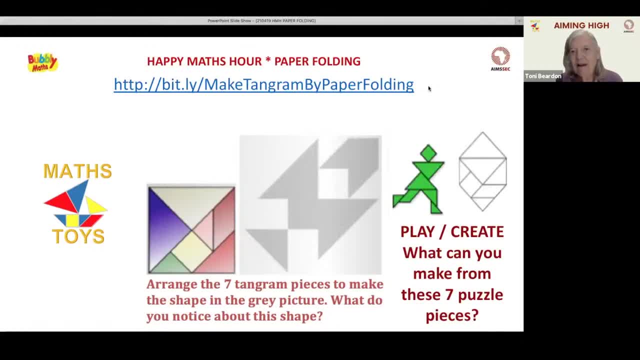 Here are a couple more. You can see- because we've not presented it here as a puzzle but actually drawn the pieces, so you can see where the seven pieces fit- the little green man who's running along. and Even so it is still quite taxing to even copy in the picture. 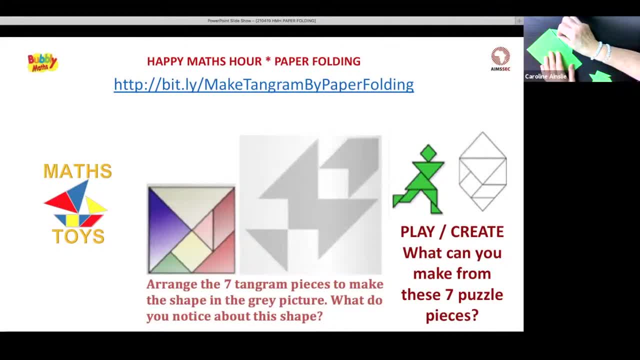 So it's a really good place to start by copying an existing picture, a picture with the outlines. It's a great place to start to get your head around it and see if it does actually work. Caroline's made the hexagon there and of course it isn't regular. 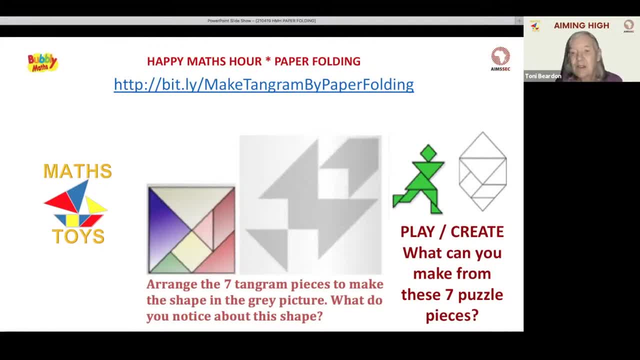 the angles are different, but you can see the hexagon shape. Now, to go back to our grey shape, which we had before, we might ask you: what do you notice? We've talked about, well, a bird or something that's flying anyway. 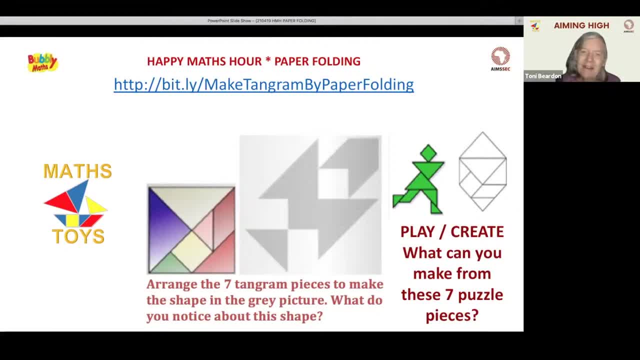 and we're both agreeing that those look like wings. but now let's get down to the mathematics. and what do we notice about the shapes? Now, if you're doing this with a group of children, a group of people, different people will notice different things. 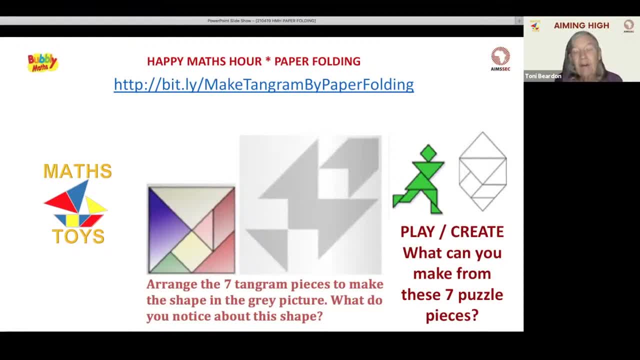 but what we use this one for very often is to talk about symmetry and, in particular, symmetry by reflection in a line. Now can you see there, the line of symmetry through the tip of the nose of this flying creature? Yeah, it's diagonal, isn't it? 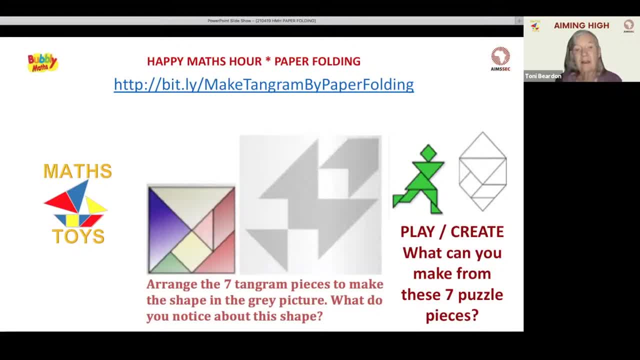 Yes, yes, yes. OK, so enjoy Tangrams. And you can see it even just from the basic, just taking two triangles like that. you can see it that way. and because it was different, top and bottom there wasn't. 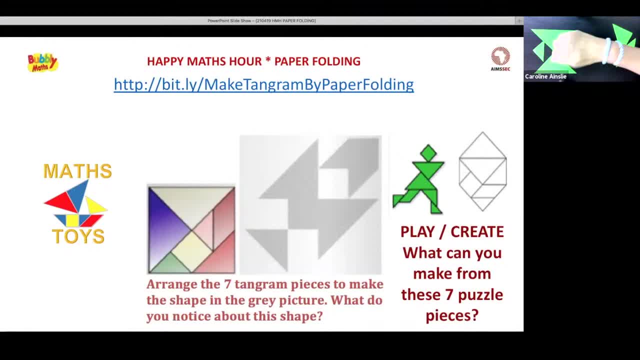 there's symmetry along that line, but there isn't symmetry. symmetry along there, There isn't symmetry. Symmetry is a very important idea in mathematics, but actually it's something that's very natural If we just look at our own hands. 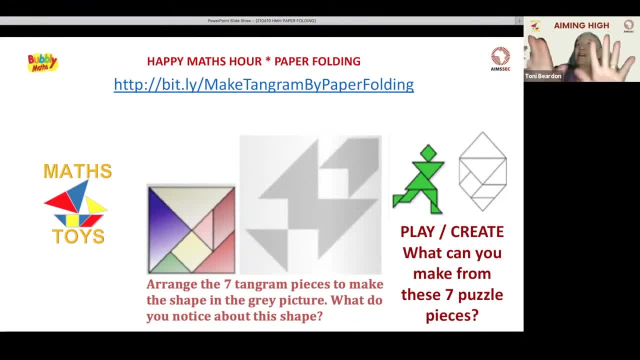 we're carrying around with us these symmetrical things, our feet too, and we've got two eyes and two ears. We're quite symmetrical- people and most creatures are, and we see symmetry in flowers. we see symmetry all around us. 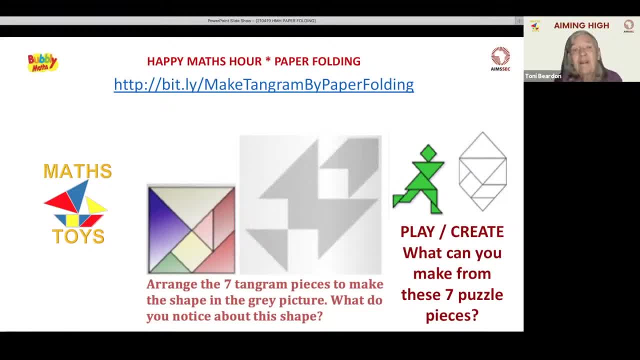 So small children understand symmetry by experience, by just looking around. But it's a very important idea in mathematics and it goes well beyond mathematics. It's used in crystallography, in physics, in particle physics, So It's very much used in real life. 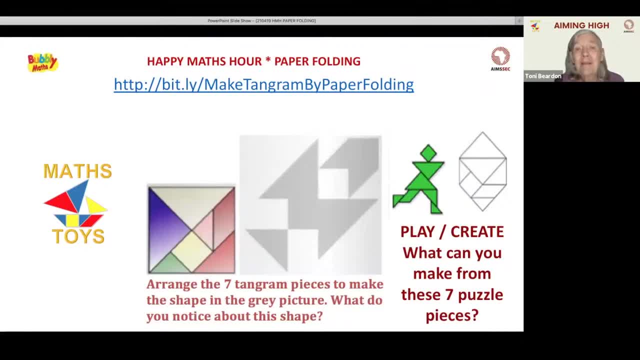 Yes, And artists use symmetry. Oh, absolutely. I mean very many gardens and many buildings are designed to be symmetrical because that's sort of pleasing to people looking at it. It's a pleasing, It gives a pleasing appearance. OK, so we're going to move on now to something else. 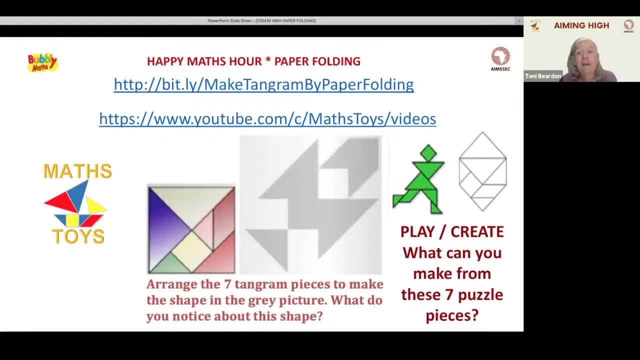 but I've just shown you the link there. There's quite a few videos on our YouTube channel and on the Aiming High website you'll find a lot of activities using all about puzzles, getting maths out of puzzles, tangram puzzles. 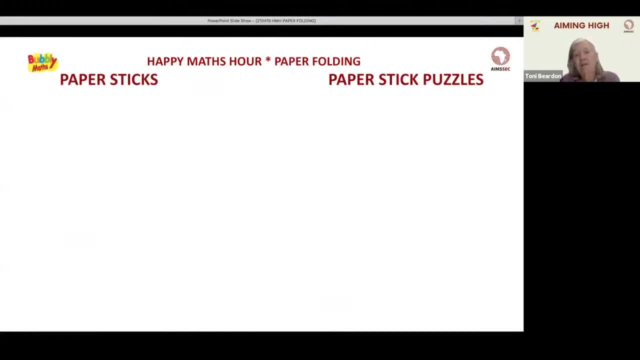 So the next thing we're talking about is paper sticks. Now, paper sticks came about. We invented the idea, I think, and nobody else came up with it first, Because Caroline's a showman, aren't you, Caroline? And Caroline does the most wonderful maths shows. 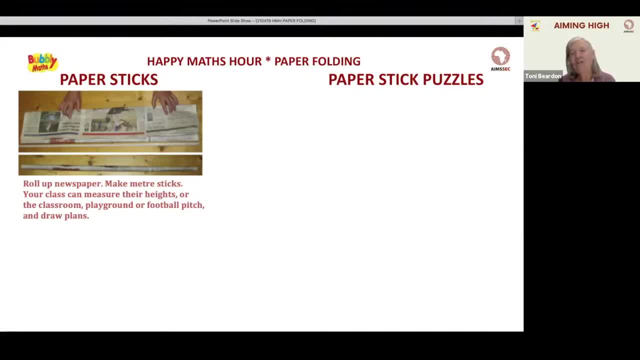 and she can entertain a whole hall of hundreds of people with maths, and that's quite an unusual thing to do. Most people don't think personally, think about when they think about maths is it's? Oh, it's not a show, It's not for entertainment. 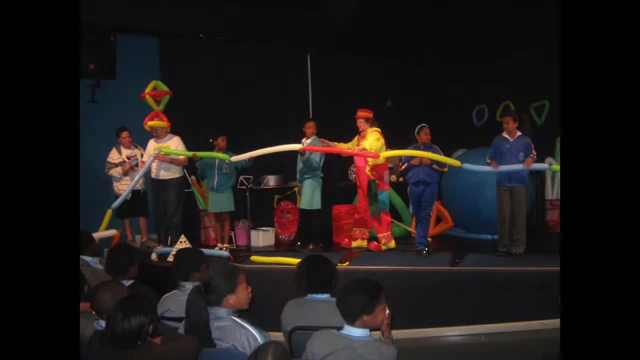 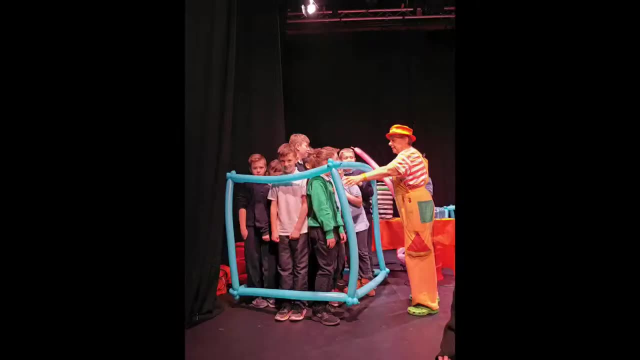 But Caroline uses metre-long balloons and then she shortens them sometimes and she does a lot of. I say Caroline does, but she has children up on the stage with her and they do wonderful things with balloons And it's sort of mathematical. 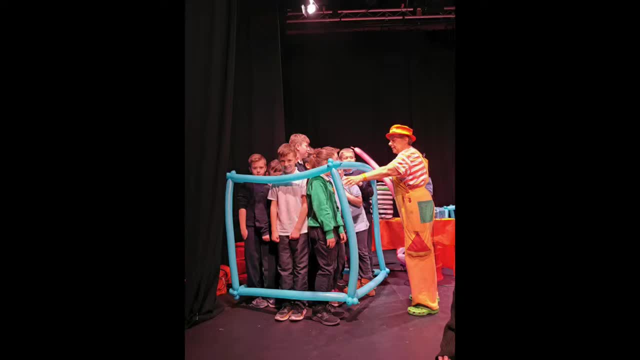 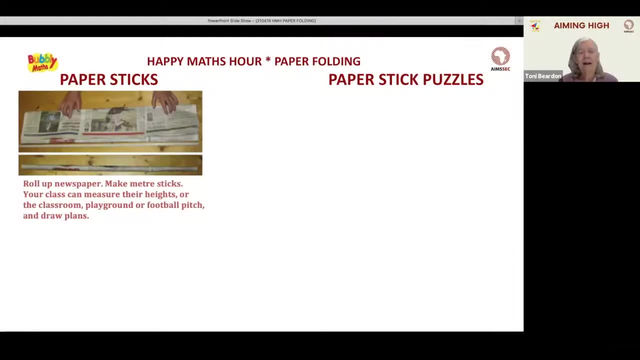 but the children don't feel it's maths, They feel it's, It's just a lot of fun. So what we wanted to do was to have follow-up activities that teachers could do in lessons after Caroline's show, that they could then relate. 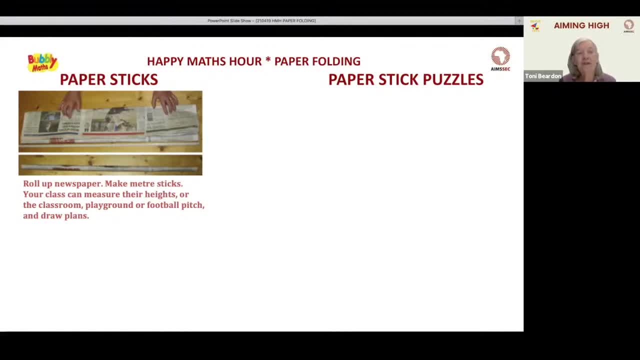 the maths that she'd been doing. the children had enjoyed to a curriculum that they had to learn at school, And we wanted them to be able to do something with long, thin. Well, in Caroline's case, she's using balloons. 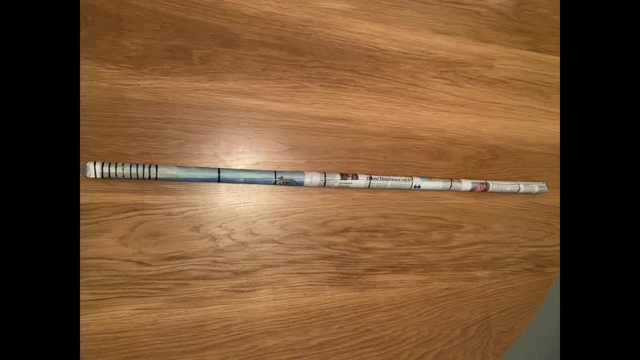 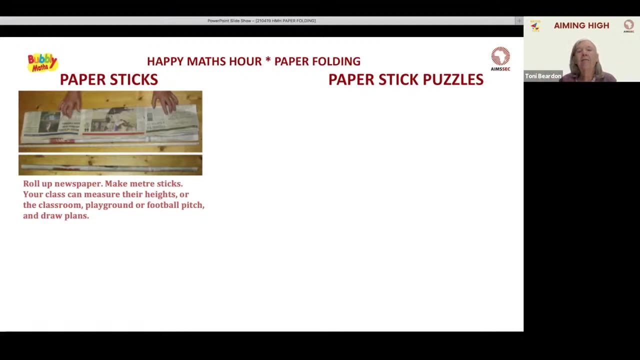 So we got this idea that you just take some old paper- it could be any newspaper or some scrap paper- you roll it very, very tightly into a stick and then you've got a stick which is very versatile and can be used for a lot of different things. 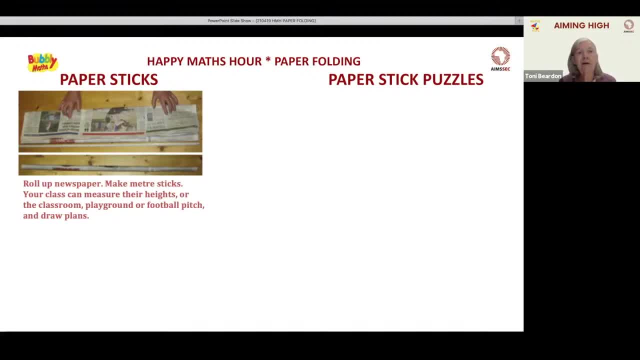 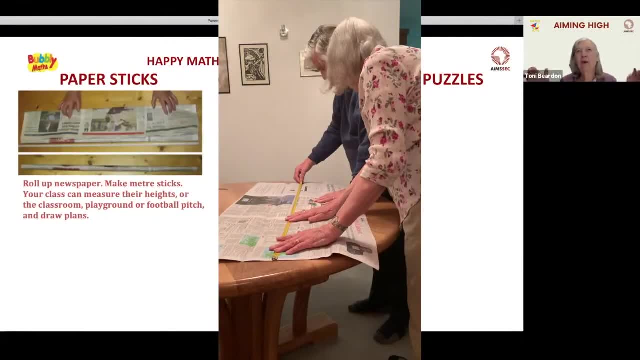 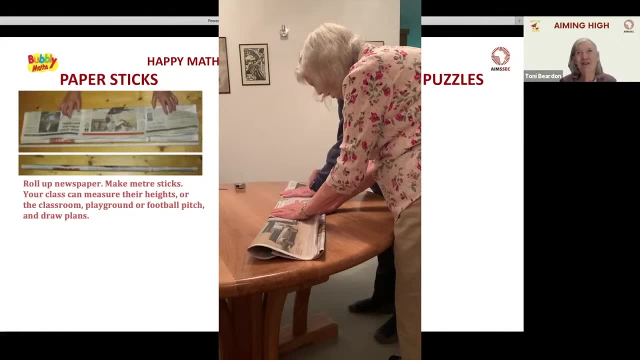 Now the one you see on the screen there is to make a metre stick to do measuring with Before you start. you want to make your newspaper probably a bit longer than a metre. You really need two people to do it. It's very hard to do it tightly with one person. 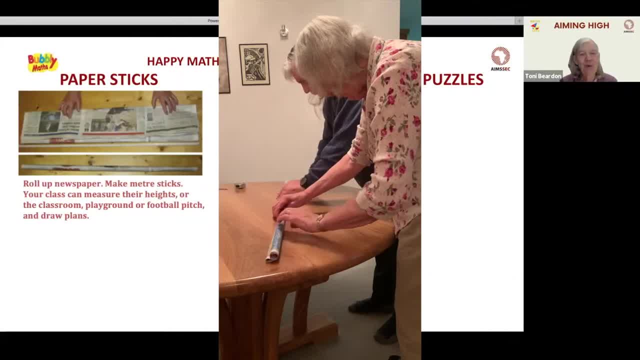 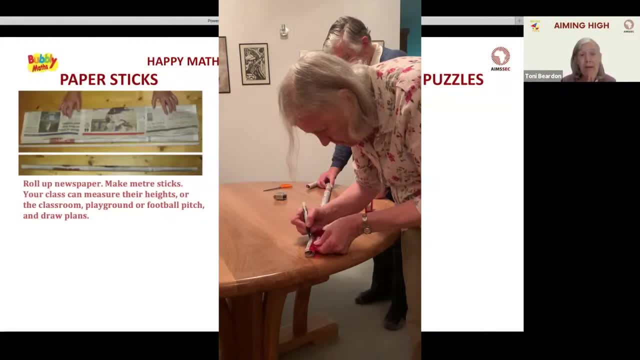 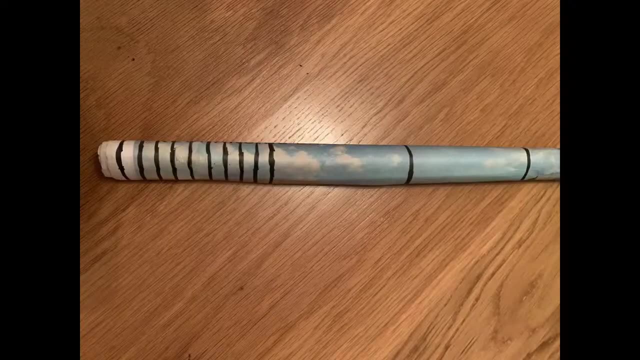 And four hands are better than two. You roll it very tightly, use some sticky tape to secure it in your long, thin stick, and then you take a short ruler and you mark ten centimetre lengths along the metre stick and then at one end, 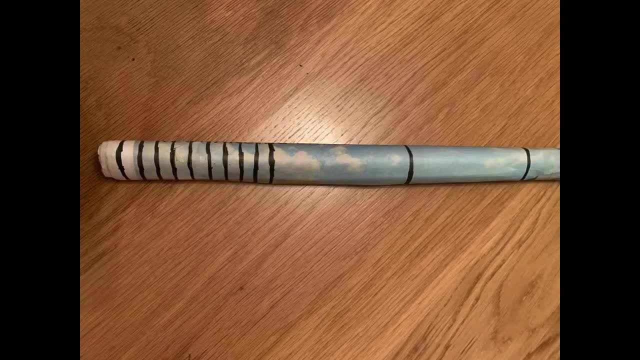 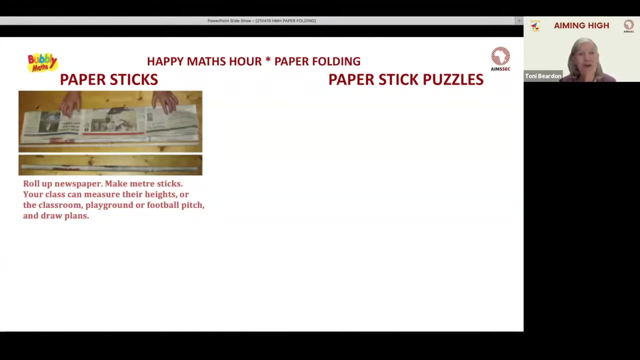 you mark into one centimetre length, so you're ready for measurement. In a classroom. children can make their own metre sticks, so one between two, and then they're ready to measure and can measure their heights, and they can then draw graphs for the class. 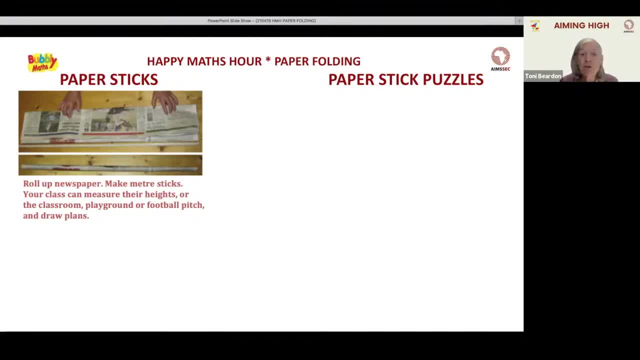 and the different heights. They can measure the classroom to draw plans or some different parts of the building and the playground or the football pitch and draw scale plans. Now, scale drawing is so important in life, isn't it? And to be able to read scale drawings. 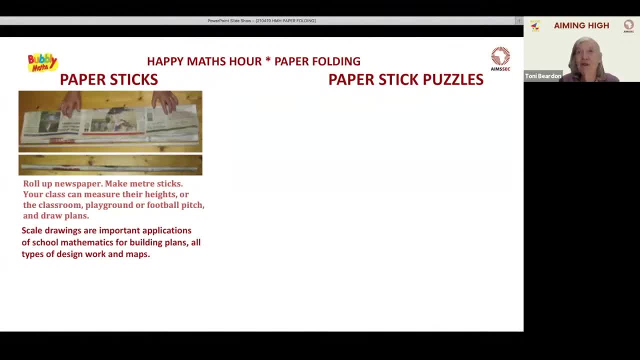 is a really important skill: Reading maps and building plans and using scale drawings in all sorts of design work- Kitchens, decorating a home, planning a bedroom. There's just so many things, And even if you're making a big project, you need to be able to make a small version of it. 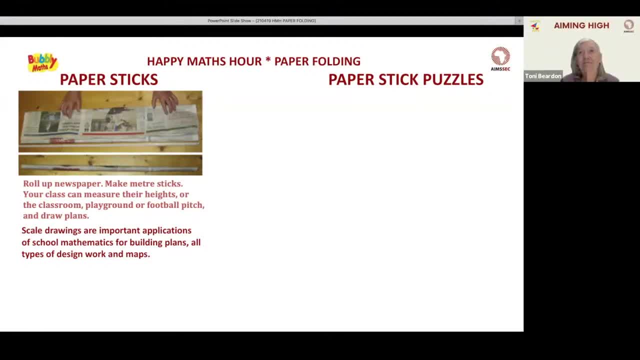 Architects, of course, are the ultimate small scale drawing people. But yeah, as you say, roadmaps, there's so many. Write in the comments what things you can think of that need scale drawings. Yes, I mean, the thing is: 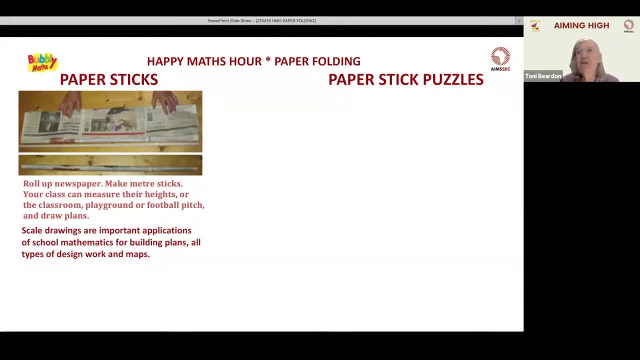 when you're maybe going to buy a new piece of furniture, will it fit in? You know, make a little scale drawing of your bedroom or wherever you're going to put this furniture and move the furniture around and see if it will fit. Not just if the furniture will fit. 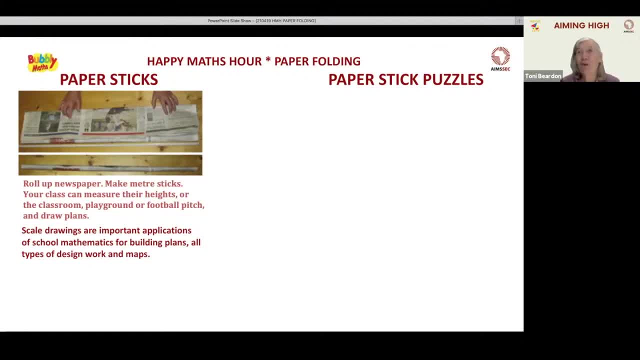 but will you be able to open the cupboard, drawers and doors? That's a very serious question. Is it actually going to be convenient to open the cupboard, the drawers and the doors and then get into it? It's all very practical. Yes. 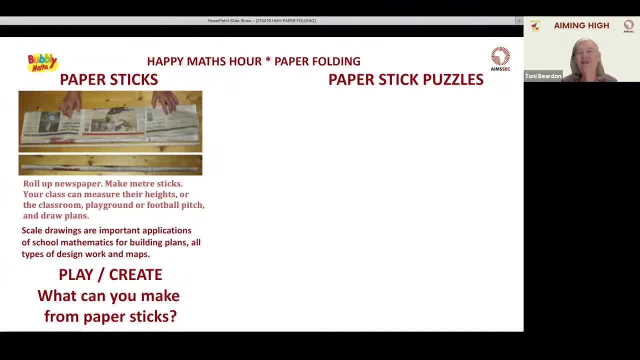 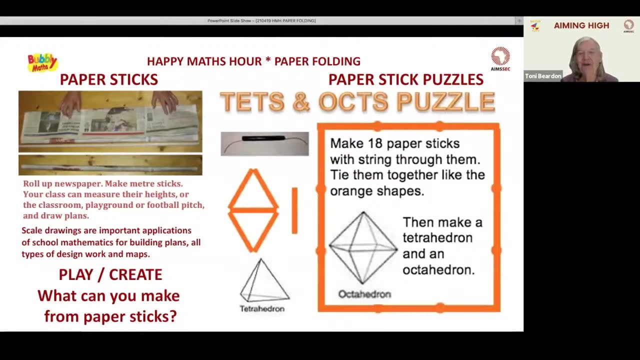 Yes, a lot of ways to use scale drawings, And so that is a very good use for paper sticks. Now we're going to go on to think about some puzzles, And Caroline's going to. Actually, there's two shown there. 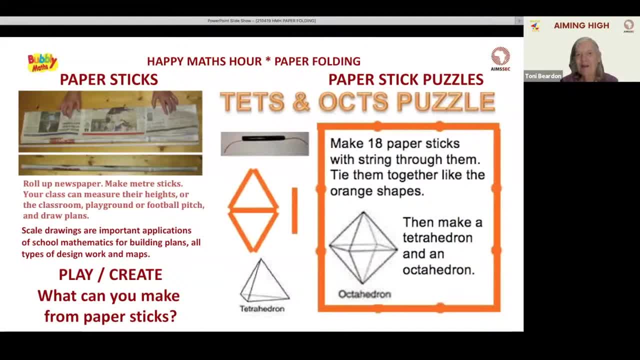 but we're going to show you three puzzles. Now we're going to move from two dimensions to three. No, we're not. No, we're not. We're going to look at two dimensions, All right, OK. well, we'll see why Caroline says that. 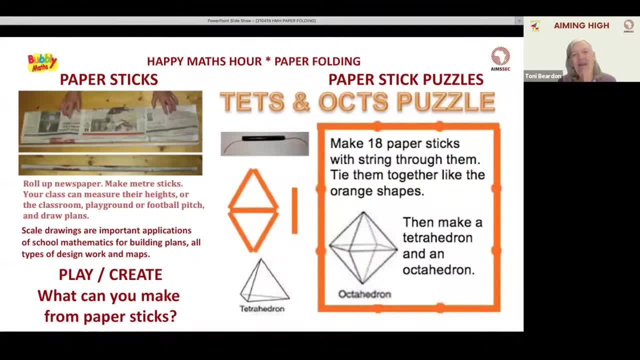 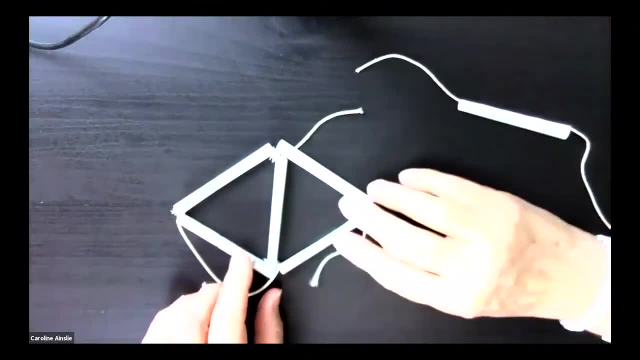 in a minute, And we're going to show you a way of learning some more mathematics using our paper sticks. OK, so over to you, Caroline, If you could stop sharing for a moment. Lovely, thank you. So what we have here is two triangles. 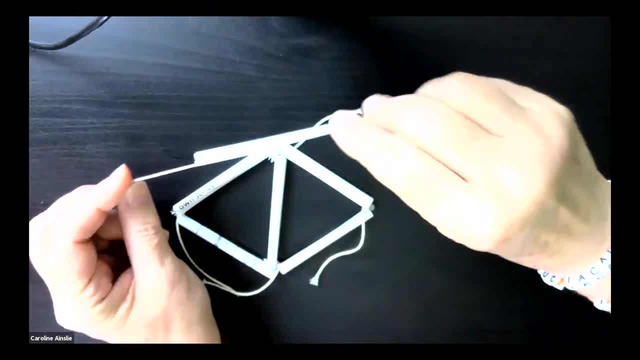 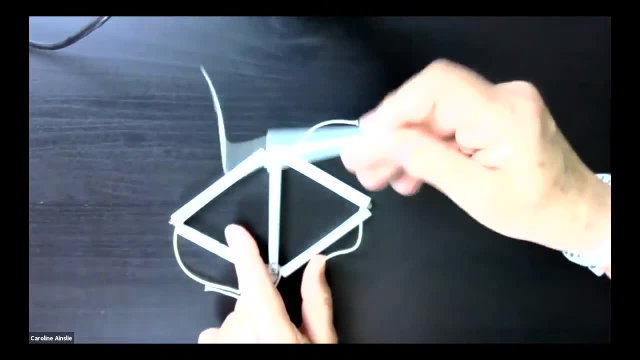 and one stick. So, yes, they've got the string on them so that we can tie them together. The objective here is: we've got two equilateral triangles and we've got one stick and we need to make four equilateral triangles. 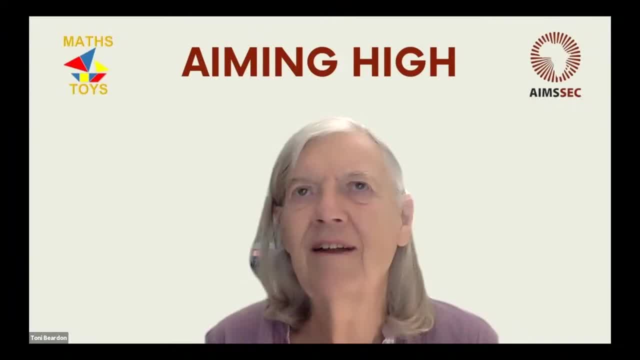 So how are we going to do it? Let me see, It's impossible, Caroline. Well, I don't know. I'm going to give it a go. I'm going to give it a go, Let's see, We can put it there. 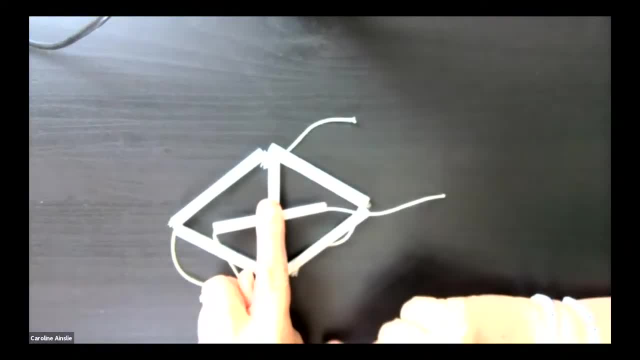 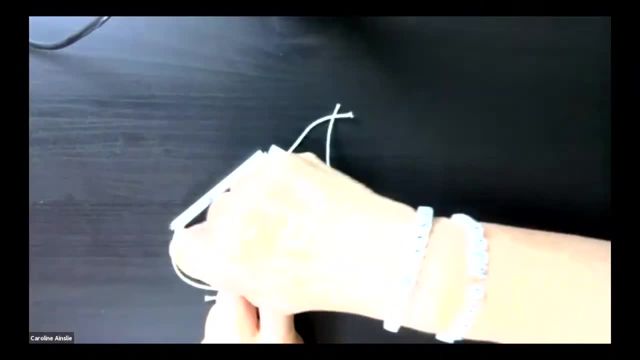 Hmm, OK, we've got a slight problem here, because a triangle is a polygon which, by definition, is a closed 2D shape with straight edges, And these triangles don't close, They're open at the end. So OK, so that won't work. 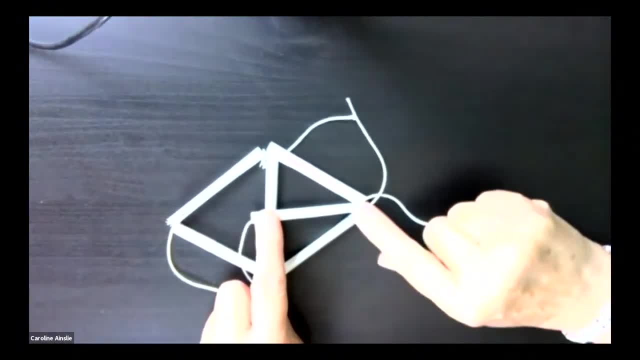 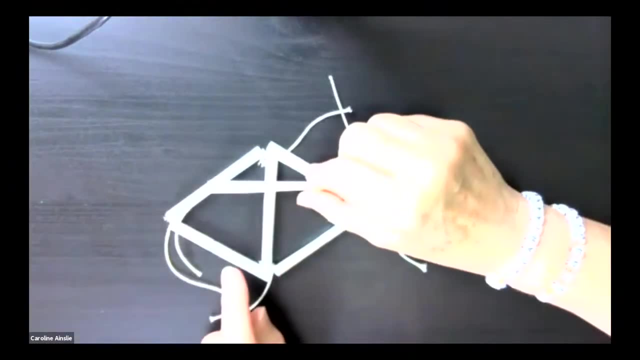 What about bringing it there? OK, now I've got three triangles, but they're not equilateral and also they're not all the same size. Hmm, What about going there? Well, I've got two triangles, but these shapes here. 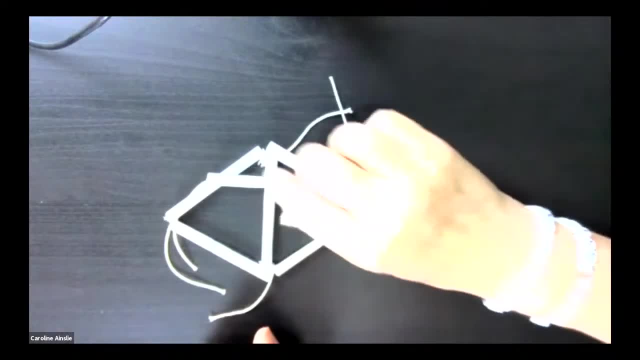 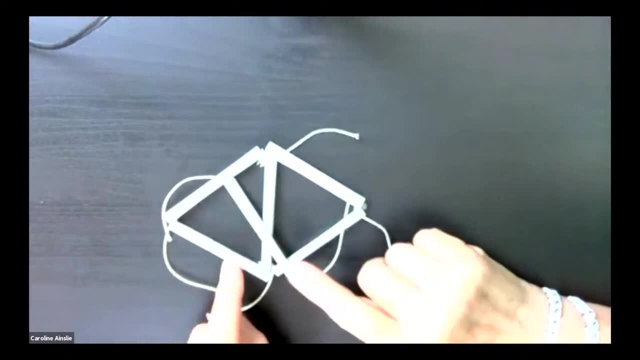 they're not even triangular. They've got four edges. They're quadrilaterals. OK, what about going that way? Will that work? OK, again, we've got the same problem. We've got two triangles and two quadrilaterals. 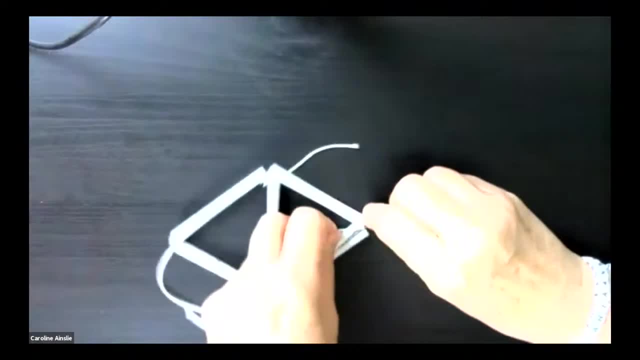 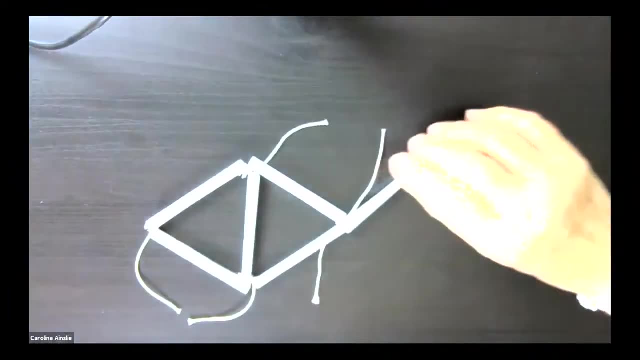 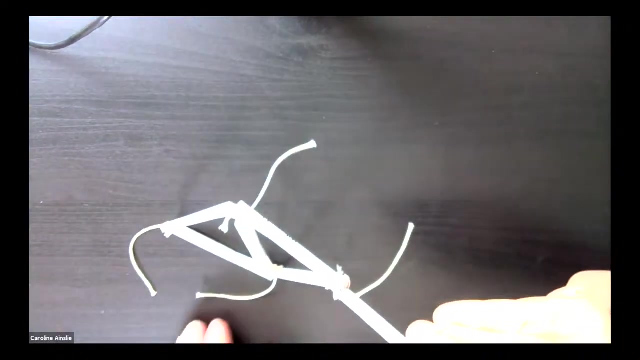 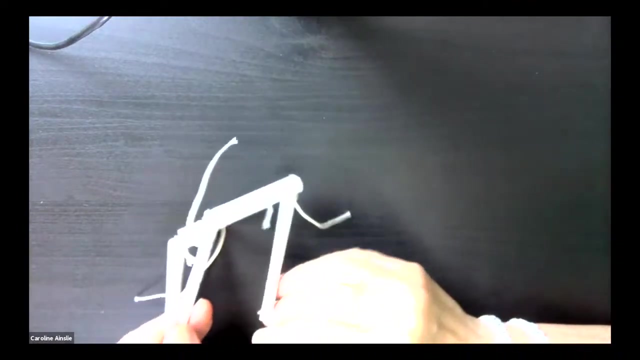 Hmm. Well, what if I? We're going to have to. I'm going to give you a little bit of a helping hand here. What about now? Can you see a way, if we now move into the third dimension, Can we actually make this magic happen? 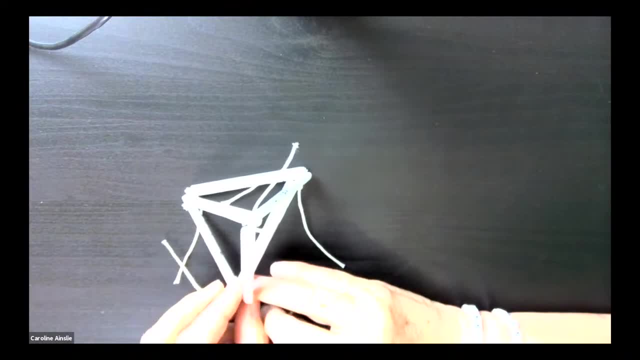 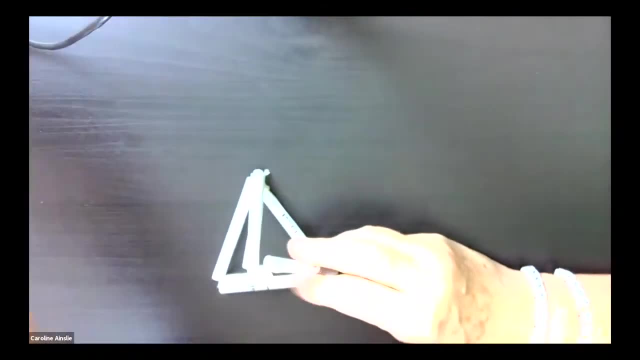 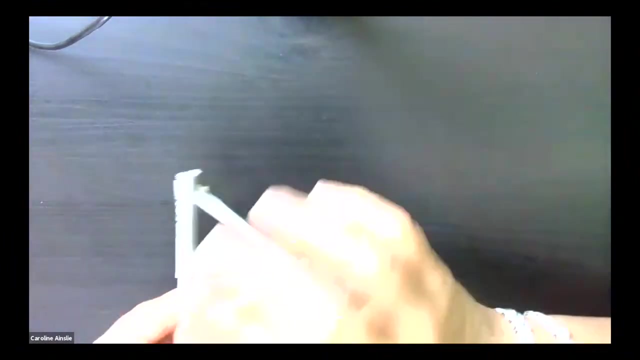 by using the third dimension. And now let's see: how many triangles do we have? I'm going to use one I made earlier so that I can move it around more easily. We have one, two, three, So that's those three. 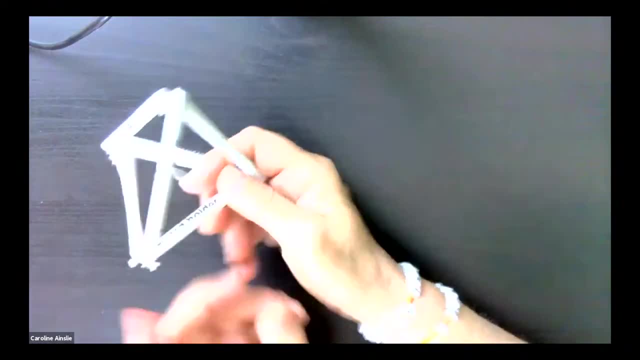 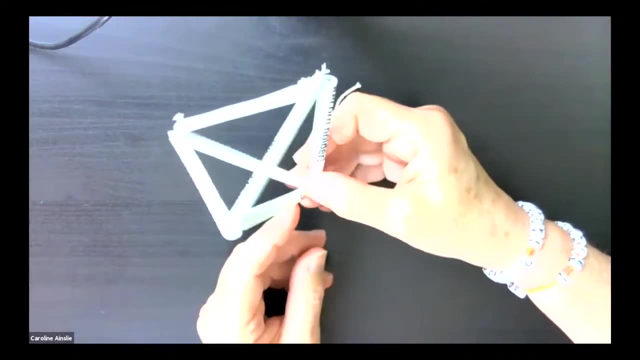 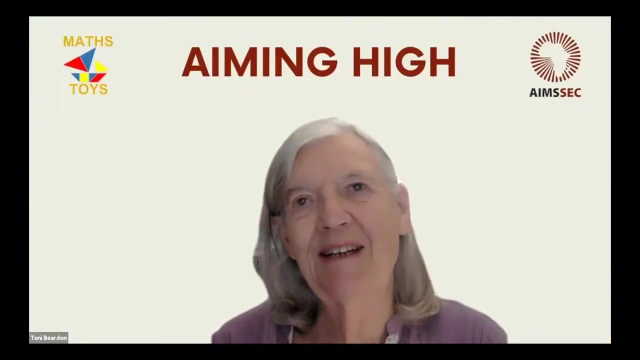 One, two, three And underneath we have another one, And they are all the same length because I've used identical paper sticks And I have four equilateral triangles making. Well, Caroline was trying to put you off the scent because I said we were going to be working. 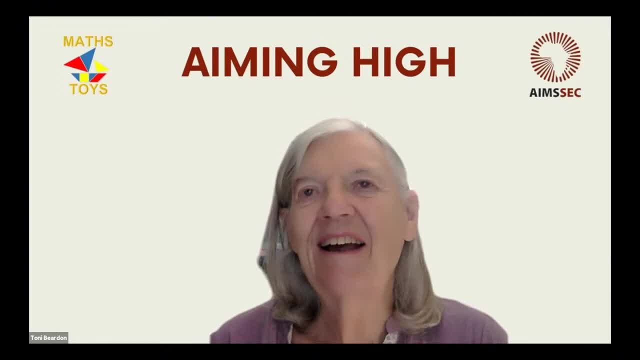 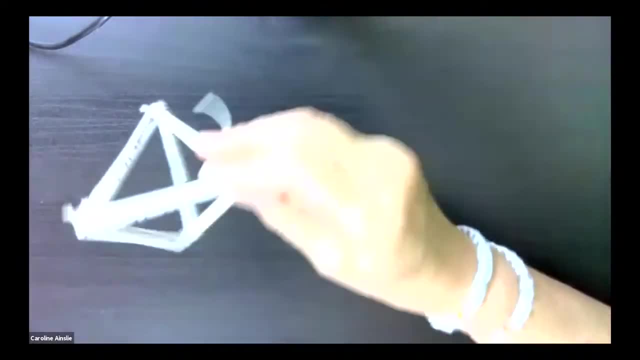 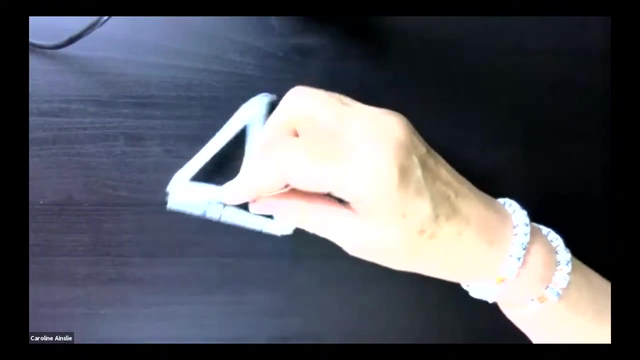 in two and three dimensions. And we are, aren't we Caroline? Well, we are. The solution is by going into three dimensions, But if you let the cat out of the bag too soon, the surprise is gone and the realisation of the power. 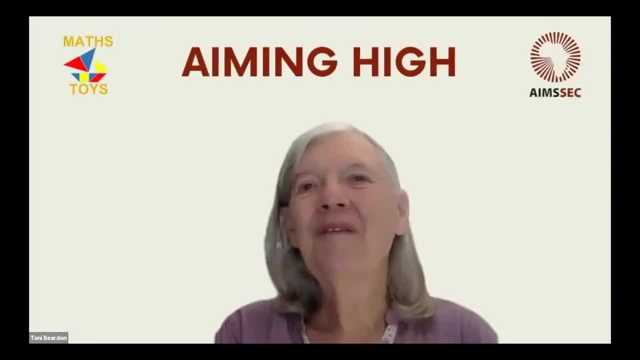 of going into the third dimension, And we want- We want the Whoever is doing this to be surprised by this. If they haven't seen it before, we want them to play an experiment with it and find out for themselves. So, actually, Caroline's demonstrated it for you. 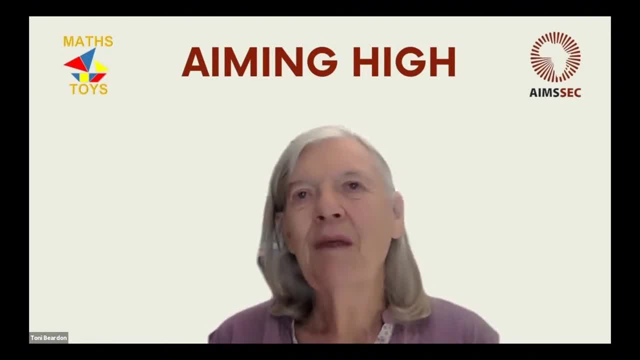 You know, if she's got a live audience there, she gets people up on the stage to assist her And she doesn't really care to do it herself. She doesn't show them. She gives them the balloons and they join them together and they have these balloons. 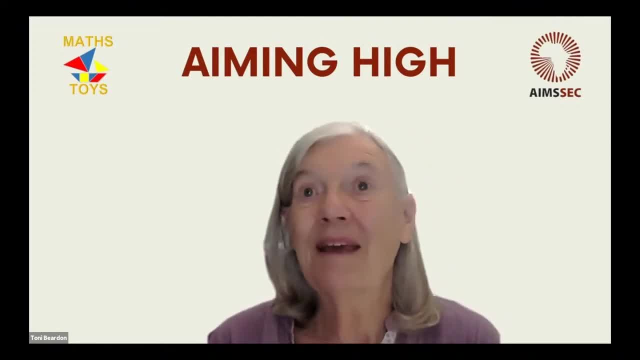 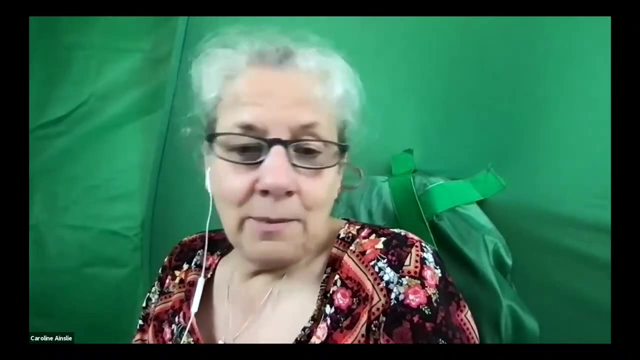 How many is it? Six balloons, And they make this tetrahedron, And they're often very surprised that they're able to do it. Surprise is a very powerful tool when learning mathematics. It's. It is something that you constantly experience. 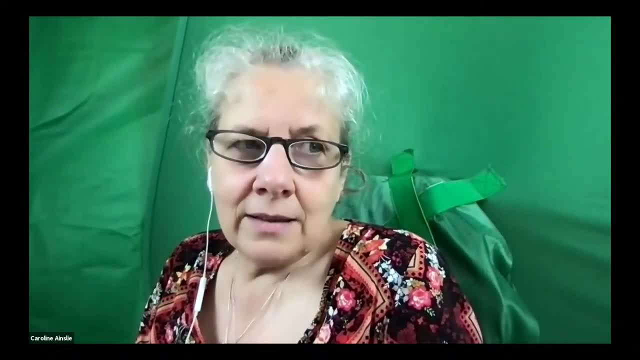 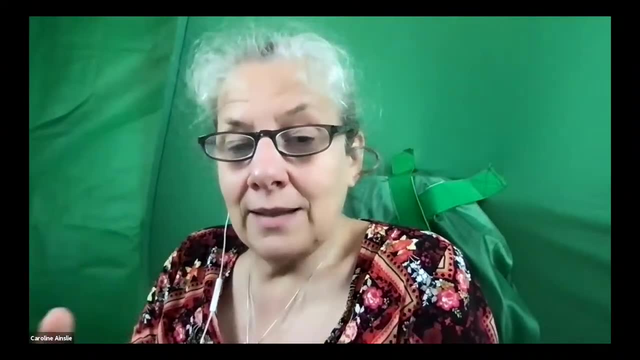 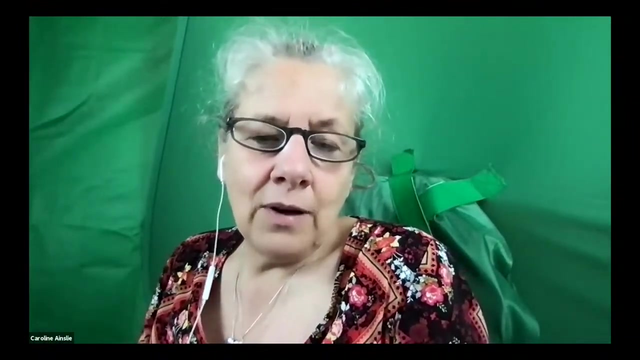 when you're learning And it's. That is an important tool in getting a learner engaged in maths and knowing that every time they do an activity there is going to be a surprise and this really exciting moment where they work things out, not just once. 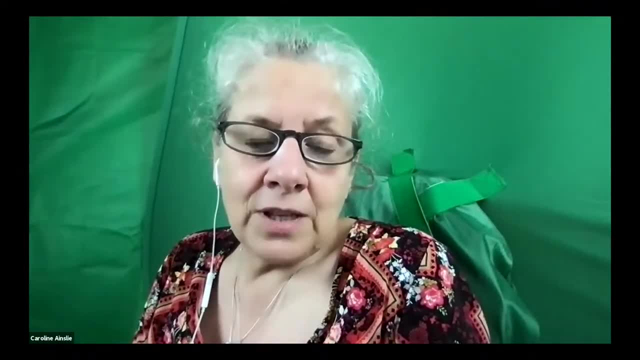 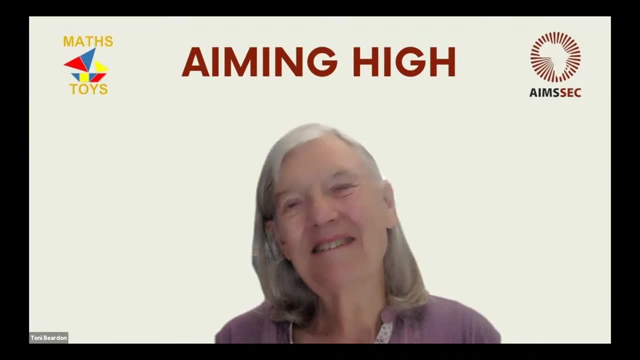 multiple times, And so, yeah, use surprise. Surprise is important. Don't let the cat out of the bag. Let the child experience their own surprise. The other thing about these spatial puzzles is that visualisation is a great help, being able to imagine something. 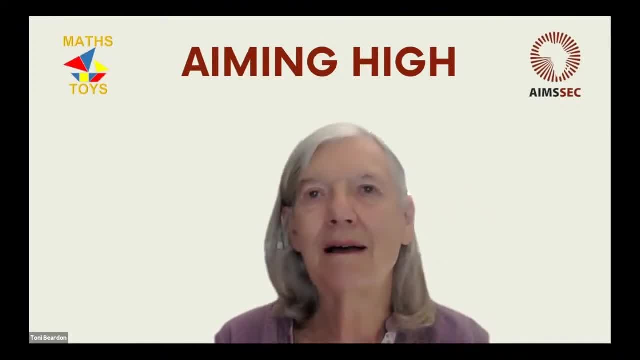 and see it with the, as they say, the mind's eye, And practice is helps to develop those visualisation skills. So we're suggesting some really fun activities here with a serious intention behind them, And the next puzzle is: We're just going to go straight for it. 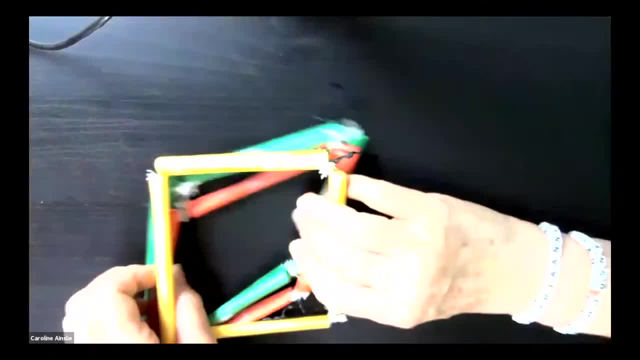 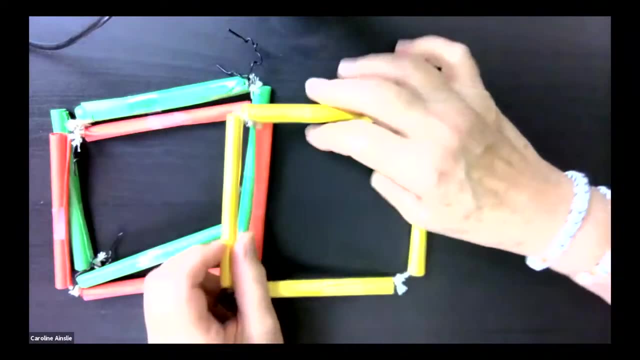 We're not going to give you any clues, And what we have here is three squares. Now they are made out of paper sticks, so they're not rigid squares. They have flexibility, But we are going to make a 3D shape. 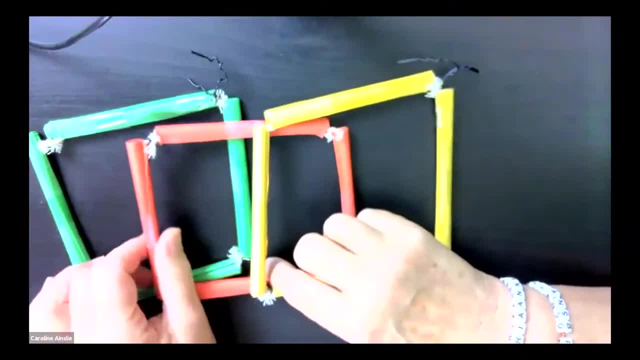 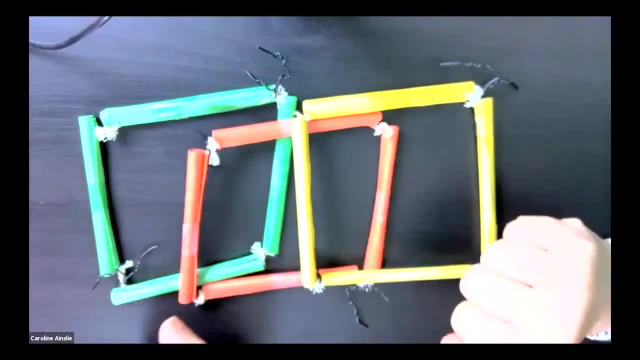 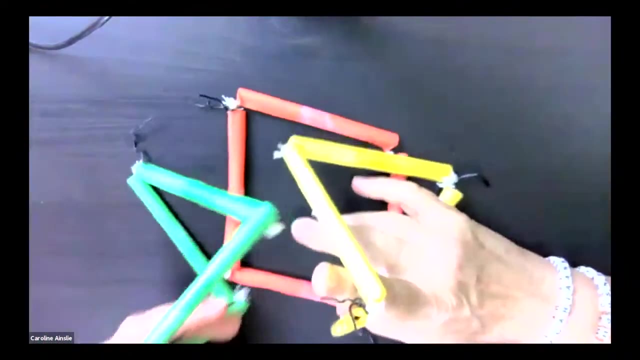 using the three squares, And they still will be squares at the end of it. So what shape can you imagine, can you visualise making with three squares? Well, the usual, The most common, I should say- shape that people say is what's known as a triangular prism. 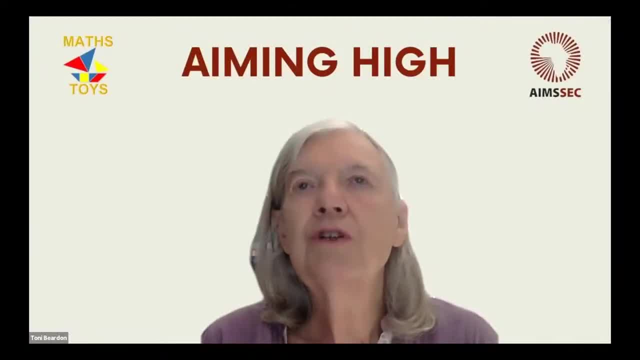 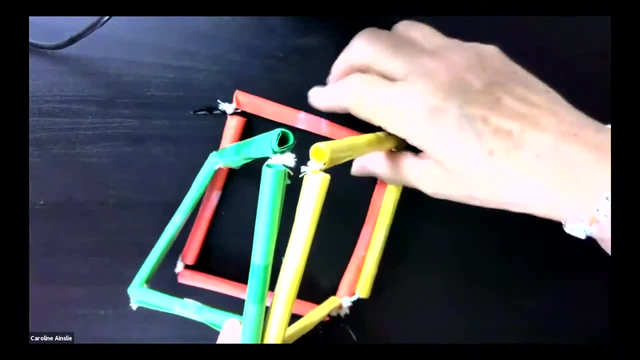 like a Toblerone bar, But you're not allowed to put two sticks together. Each edge should be just one stick. Yeah, well, I didn't say that, I just said a 3D shape. So that's fine. So, yes, that. 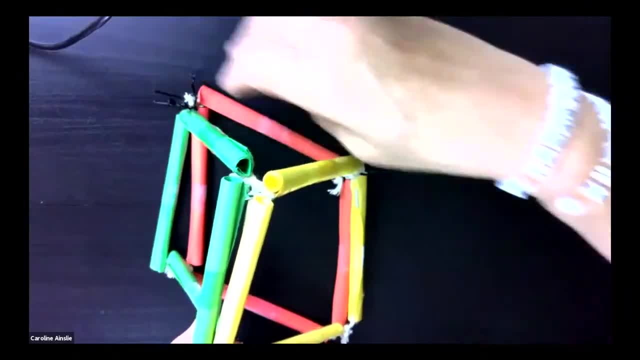 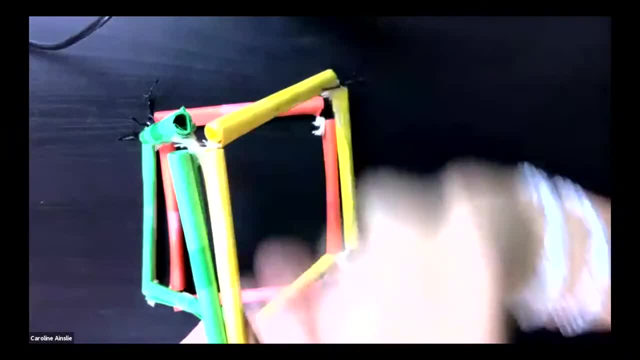 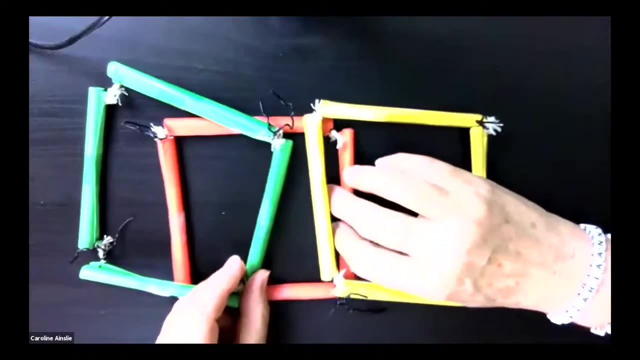 I didn't mention that yet, But that is the rule. Every edge cannot be two sticks, Every edge must be just one stick, And you've got to use all three squares, and all three squares will still be shaped like a square. Well, you can let people have a go. 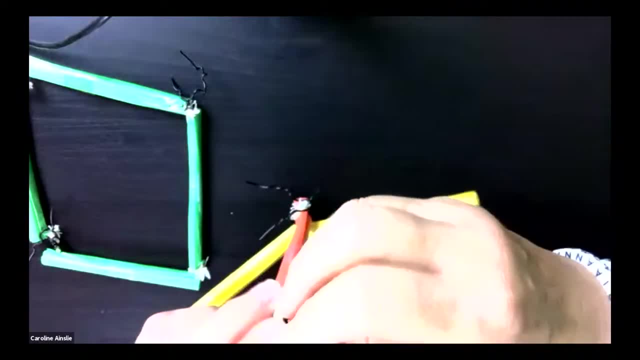 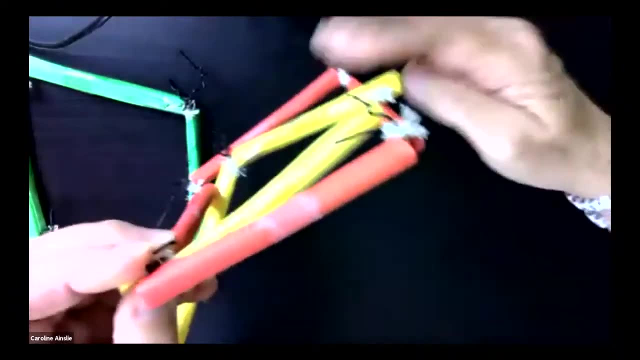 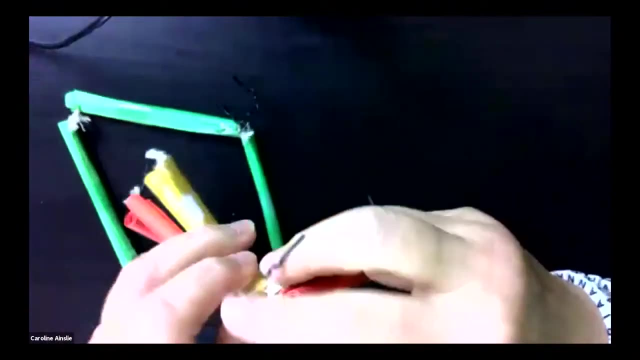 have a nice go and depending. But I'm going to just go straight to an aid for the solution, So I'm just going to use these. These are just cable ties, the kind that you get when you buy equipment, the one that curl round like that. 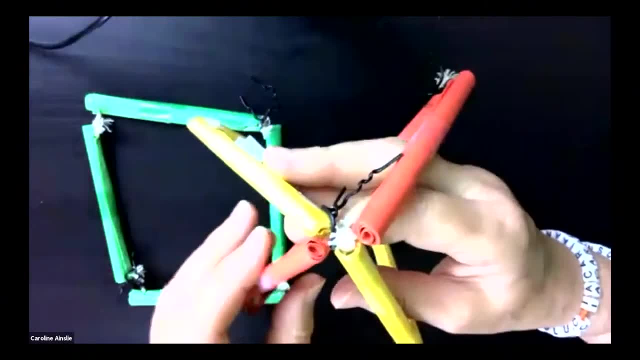 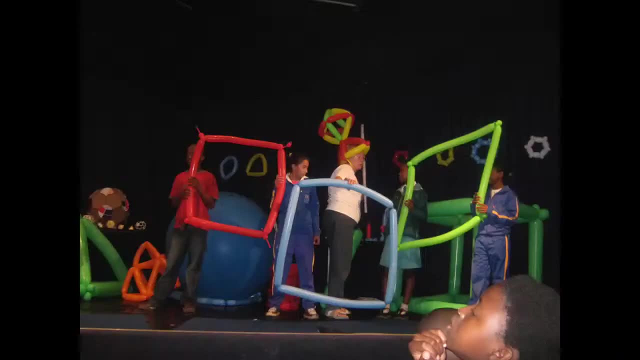 So I'm going to give you a little bit of a clue here so I can demonstrate this. You can see it in different angles. Mine will have some children up on the stage, each one holding a square, or maybe two people for each square. 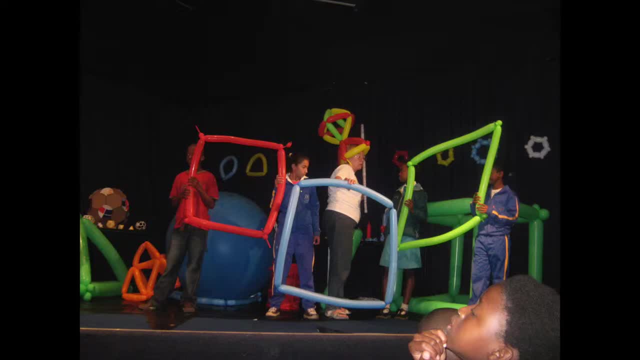 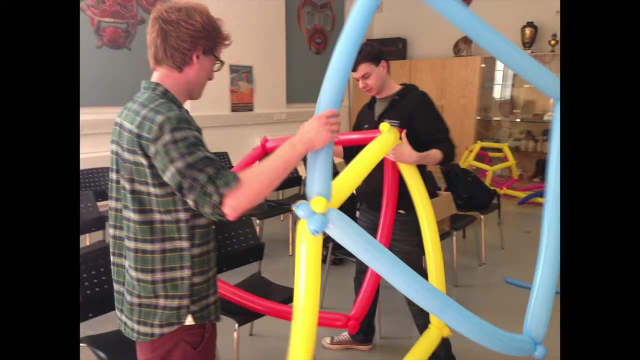 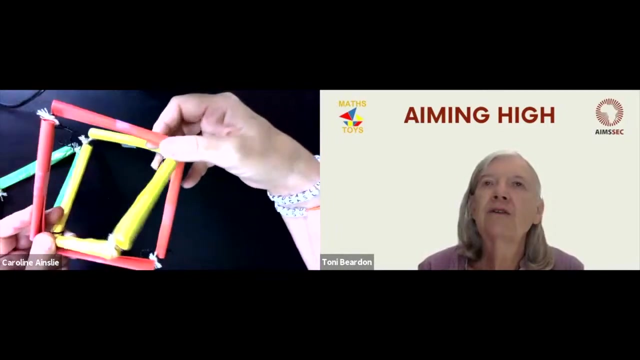 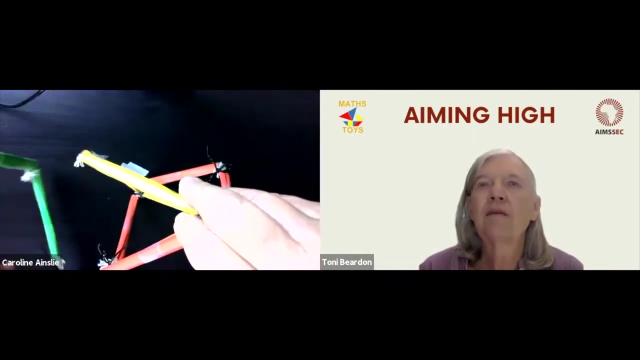 huge, huge squares, And she will get them to try to make this shape. At this point they will be holding it up, with those two squares linked together at two opposite vertices there, And the idea is now to use the green one the other one. 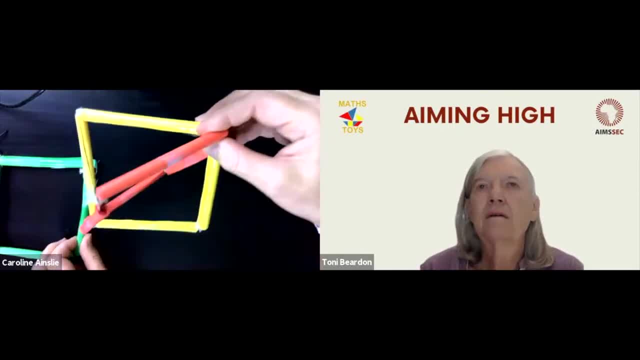 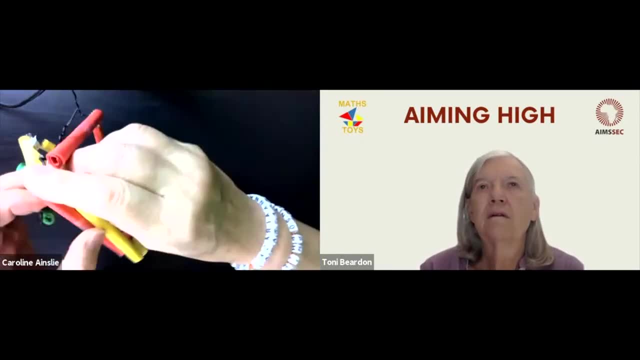 What do you do with it? Where does it go? And I can hear some of you screaming: put it through the middle. Well, when I'm doing the show, I actually then go do this, put it through the middle. So language is also important. 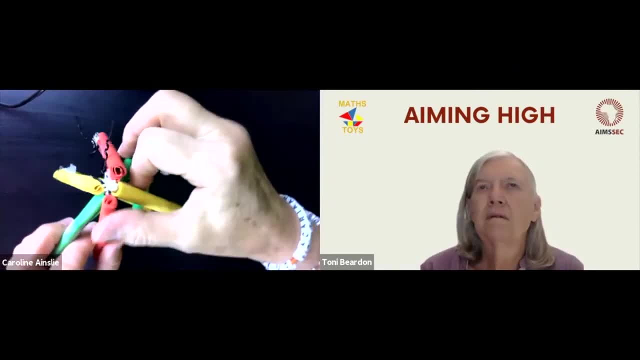 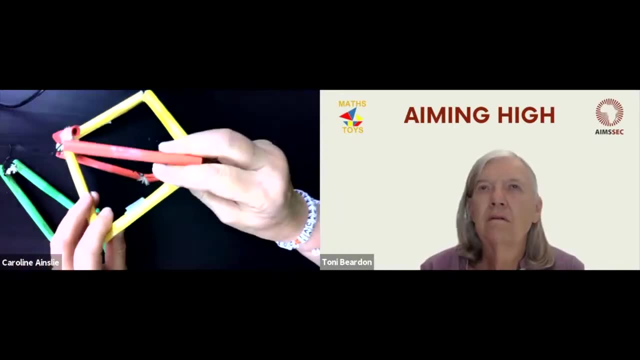 That's to demonstrate how important language is. And yes, that is a 3D shape, but it's not a 3D shape made up of squares- The faces- well, the faces are not polygons. In fact, there are no polygonal faces at all on there. 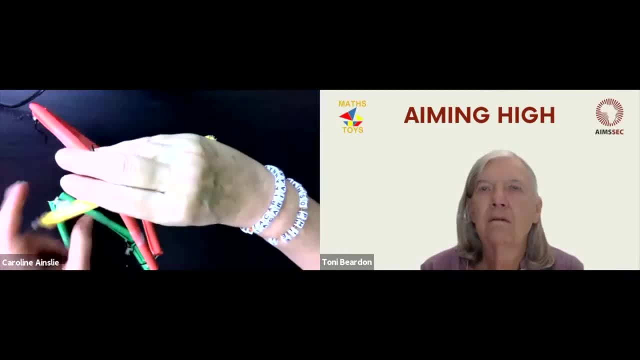 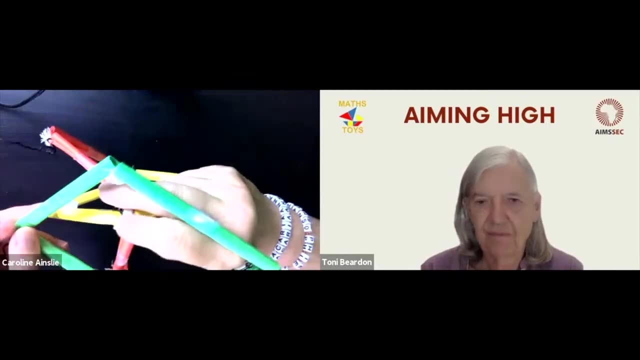 So we actually need to make a shape, And I'll give you a clue. We need to make a shape made up of triangles. They will all be equilateral triangles And the way that you do it, we can do it through the middle. 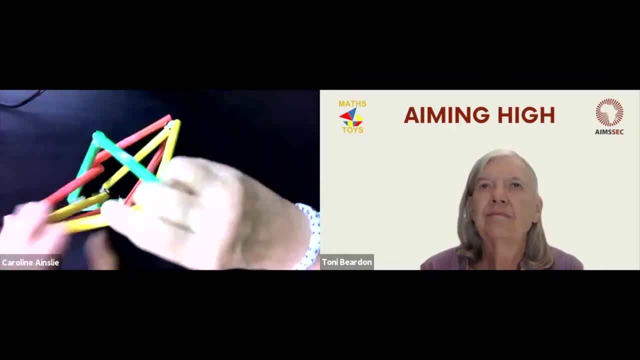 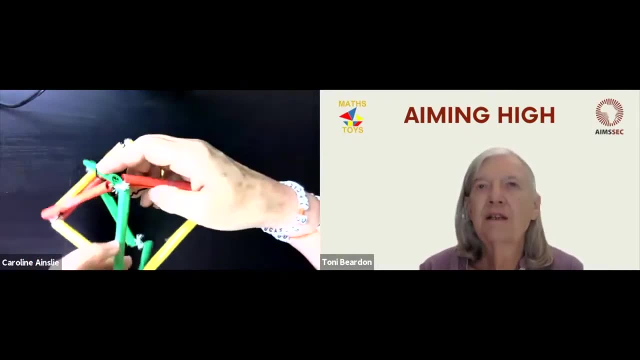 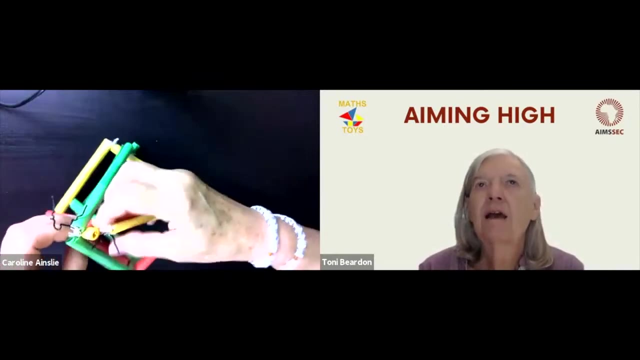 I'll do it over the top. I use my little ties here- Tony, would you like to talk about it- while I just tie them up? Absolutely yes. So what we're going to do is we're going to end up is a shape with triangular faces. 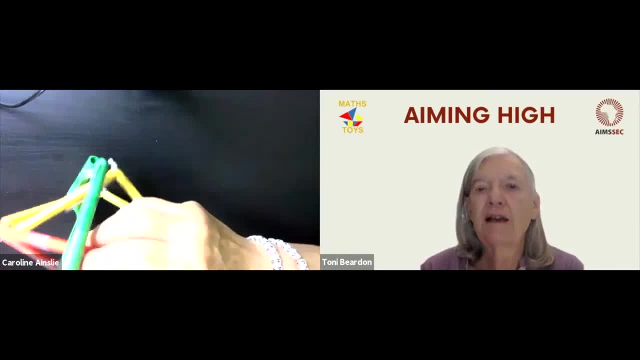 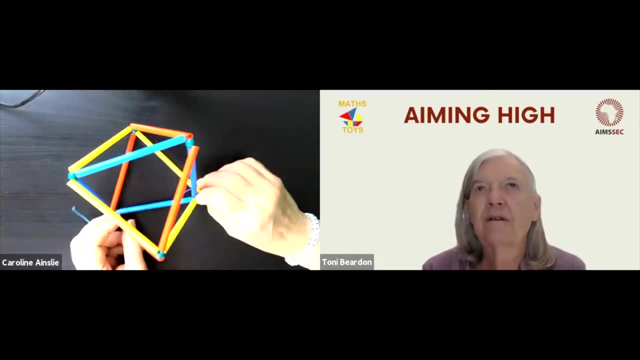 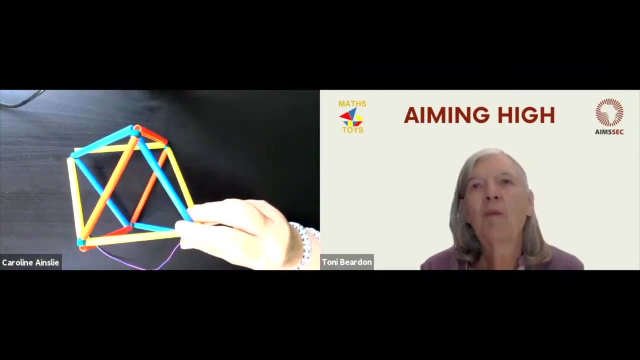 At each vertex. we're going to have four edges And I'm going to cheat. We've got 12 edges. Here's one I prepared earlier. Yes, there you are, And now you can also see, I think, why we chose. 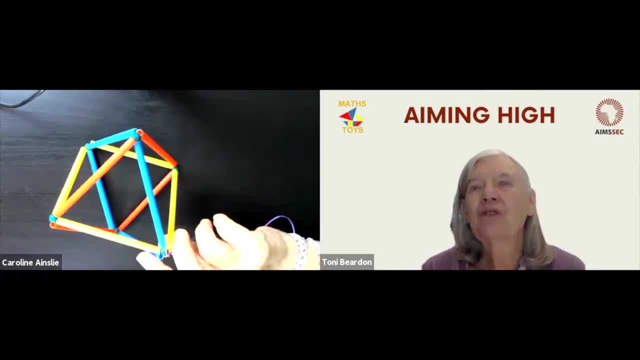 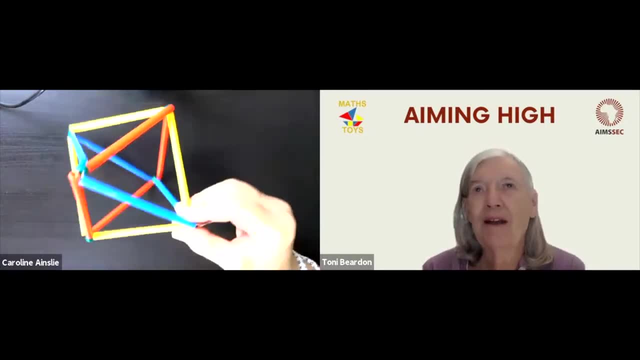 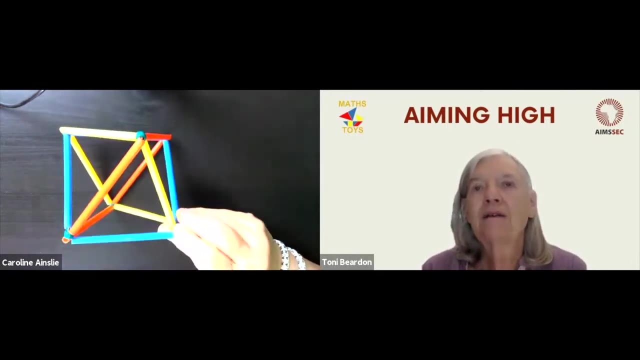 well, I hope you can. You can see why we chose to make the squares, each square, a different colour. So you see a yellow square there, a red square and a blue square, turquoise coloured blue square, And we're back to symmetry. 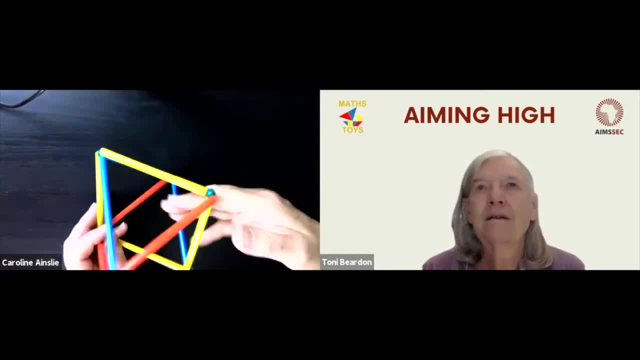 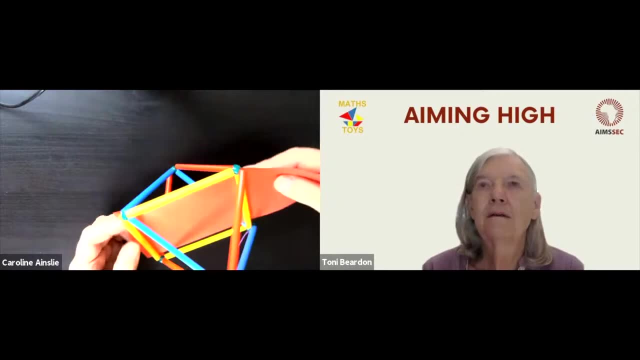 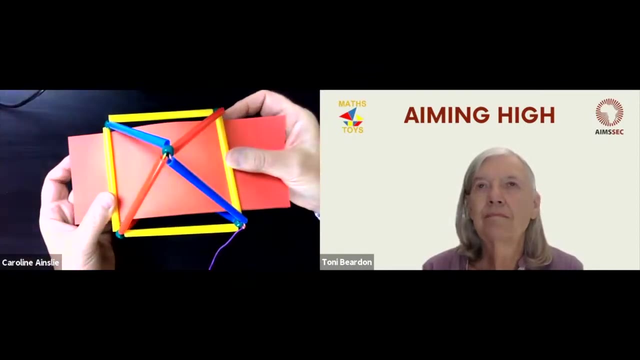 aren't we, Caroline? We certainly are, If I stick my hand through there, if I maybe use a card so you can see it. But this is your mirror. Look at it from this face or from that face, assuming that the card goes. 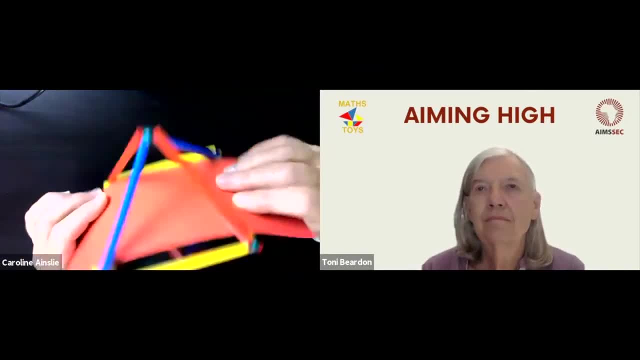 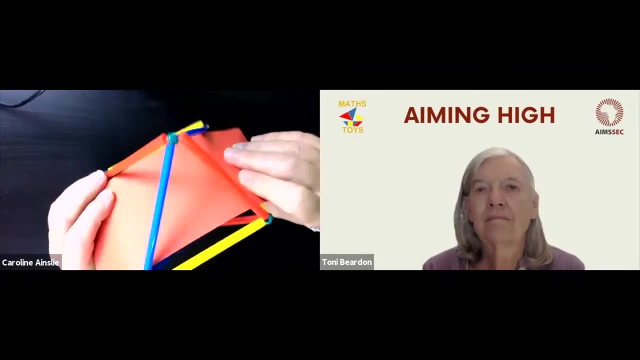 right through that middle square. The amount of triangles are identical on both faces. So when I ask people to tell me how many faces this shape has, if you start counting- one, two, three, four, five, six- Wait a minute. 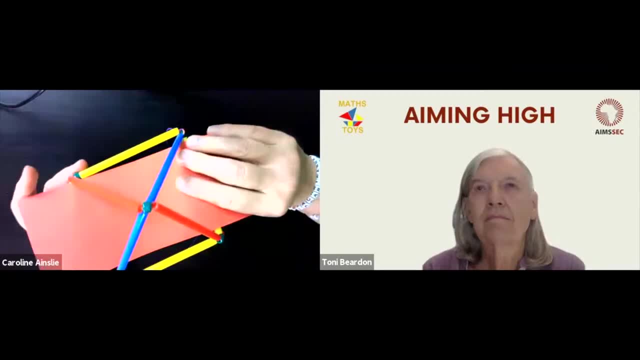 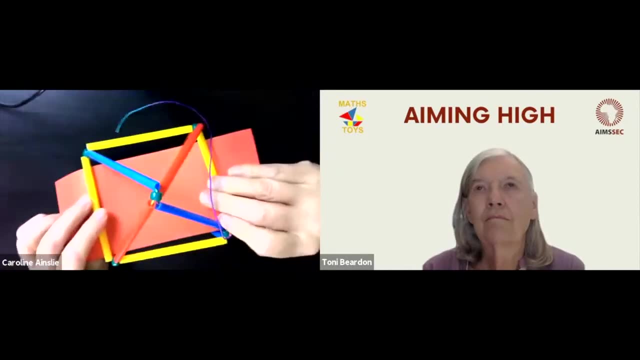 Have I counted that? one, Nine, ten? I don't know how many faces there are, But if you just count on this face from this way around- one, two, three, four- you can see that the opposite end has the same amount. 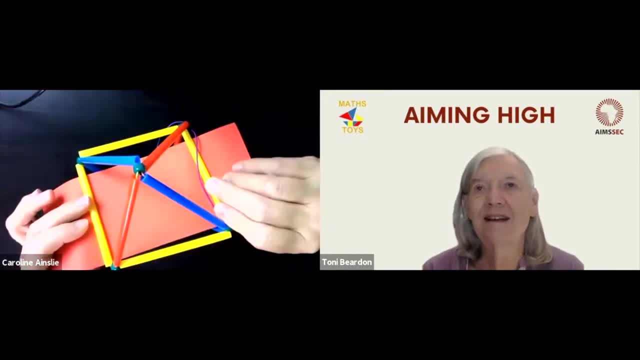 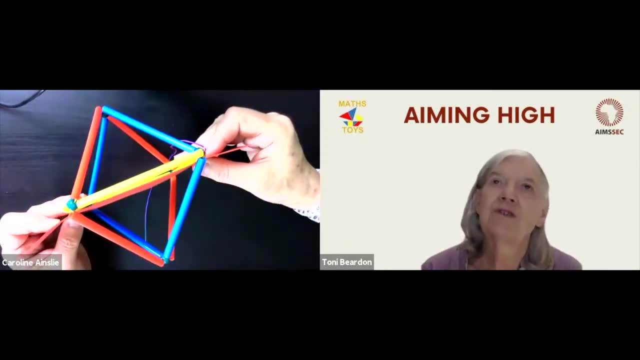 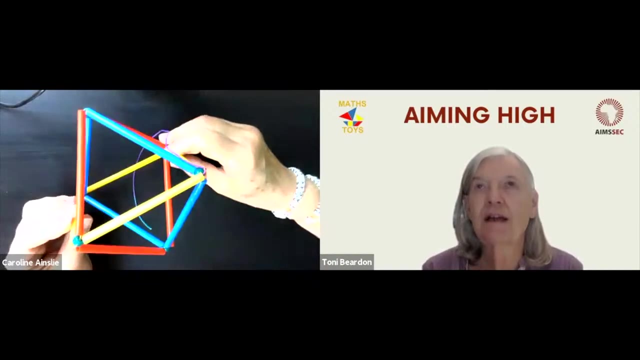 So there are no more. That's all there is, And what you can see is the card that Caroline's showing you. In fact, she's really just trying to indicate that yellow square is what we call a plane of symmetry. It's like a mirror. 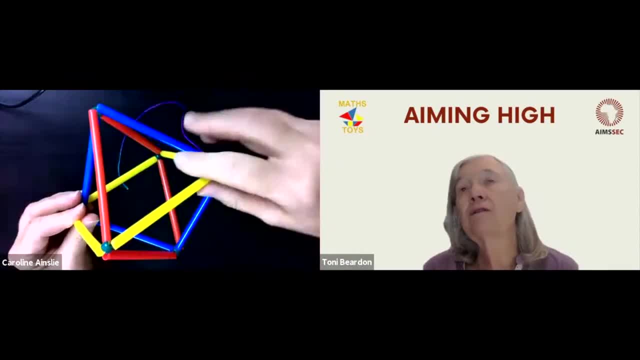 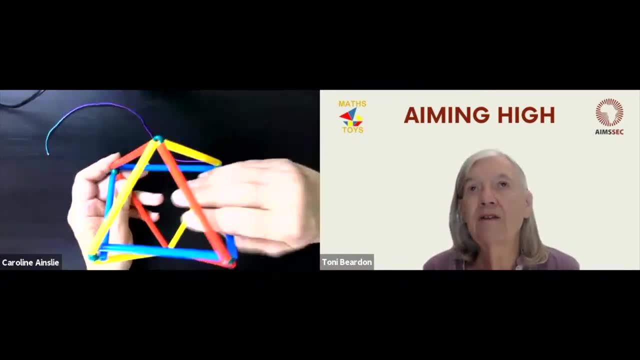 a flat mirror And the other one, the other two planes. so the red plane, equally, is a plane of symmetry And the blue plane, again, that's also a plane of symmetry. So we talked about with the grey tangram shape. 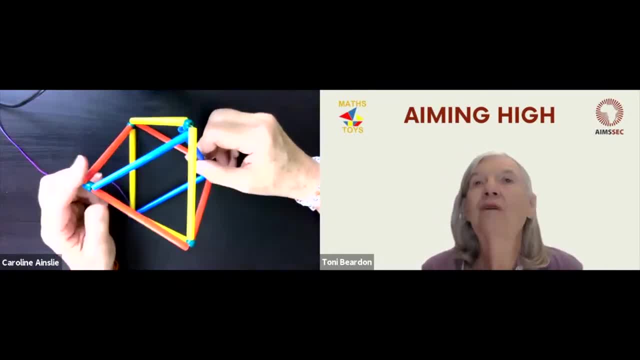 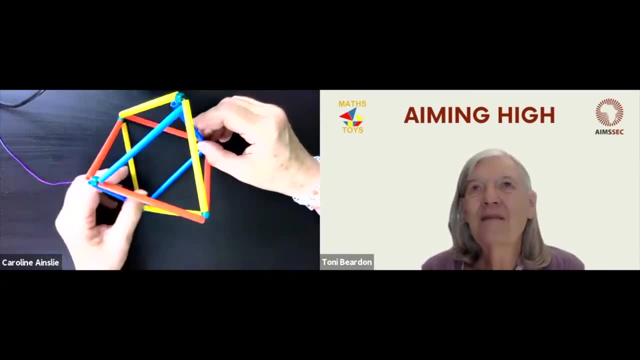 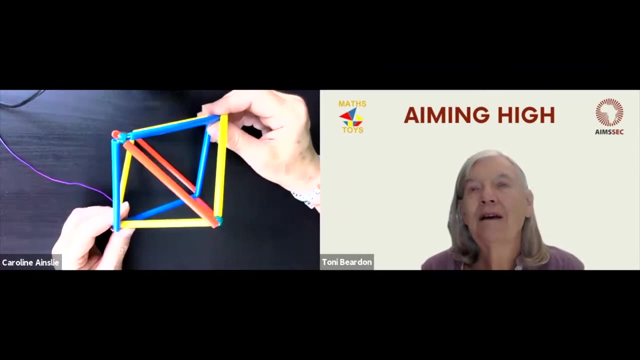 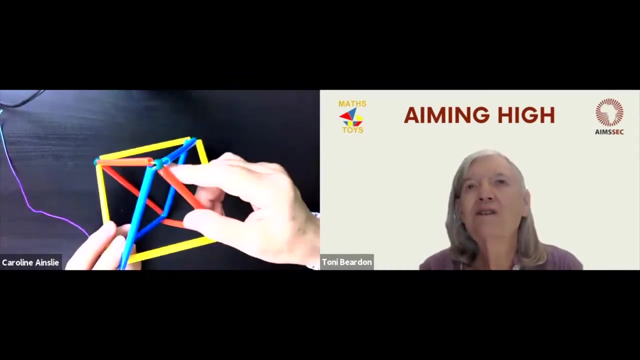 that was all in the 2D, And now we're looking at symmetry in three dimensions. Also, we've got here what we call a regular shape, And what we mean by regular is: everything's the same. All the faces are the same shape. 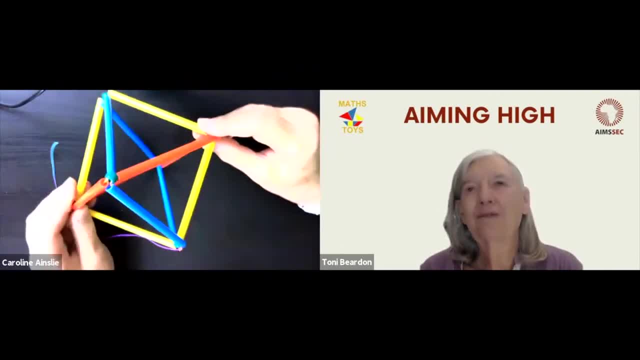 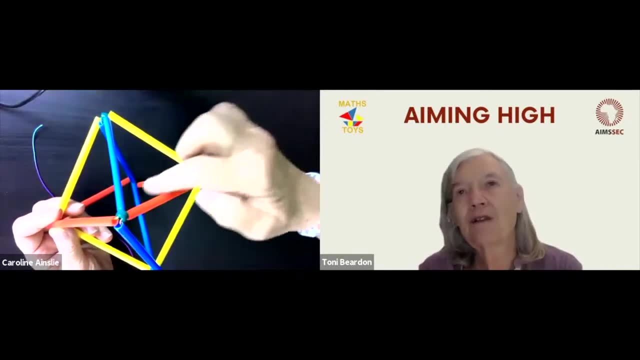 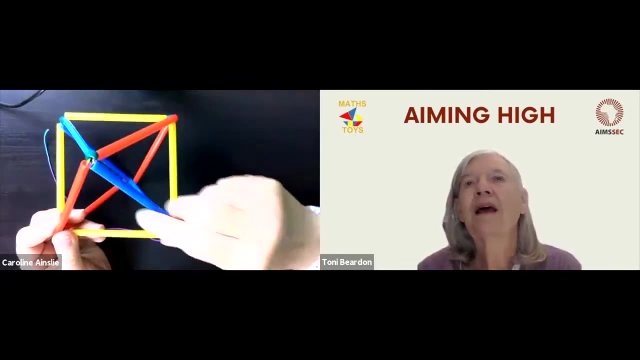 They're all equilateral triangles, All the angles are the same. They're all 60 degrees. Well, the angles in the faces are 60 degrees And all the lengths of the edges are the same. And that is one of the famous 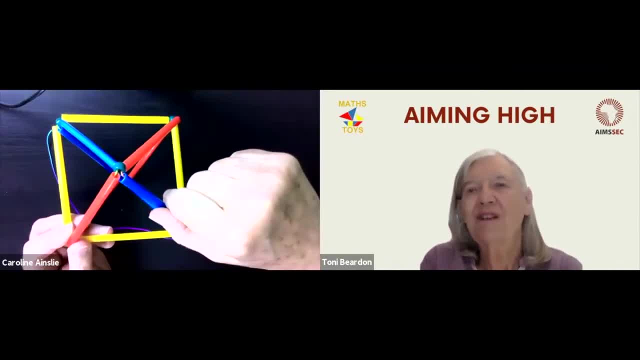 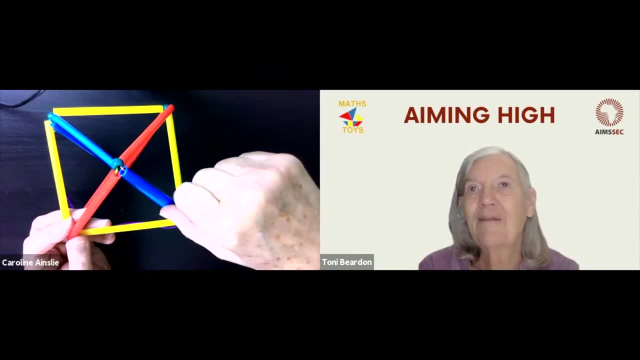 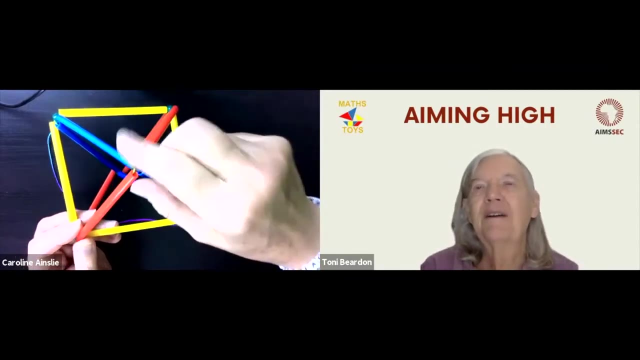 platonic solids described by Plato, who actually established that there were only five of these. They're all common shapes or pretty well-known shapes, And this is the one, the octahedron, And the other thing is that every vertex has the same number. 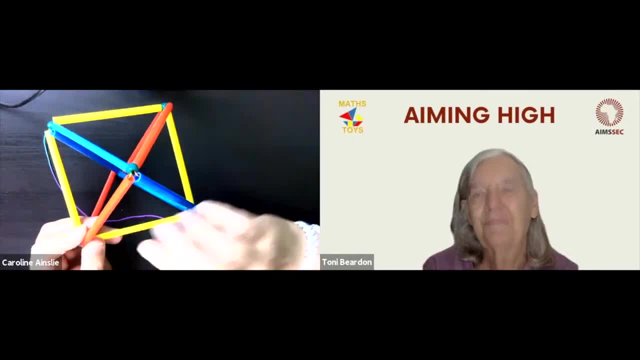 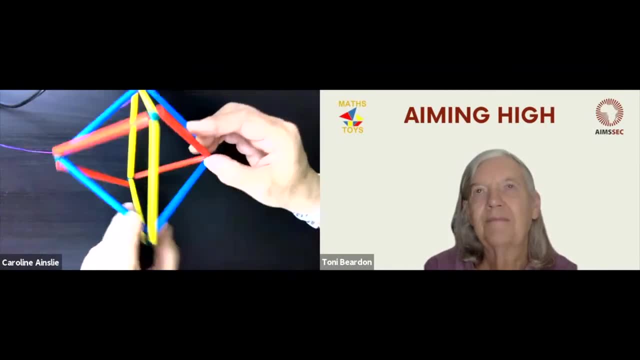 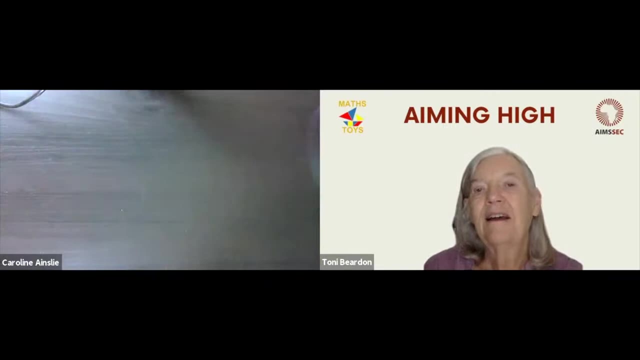 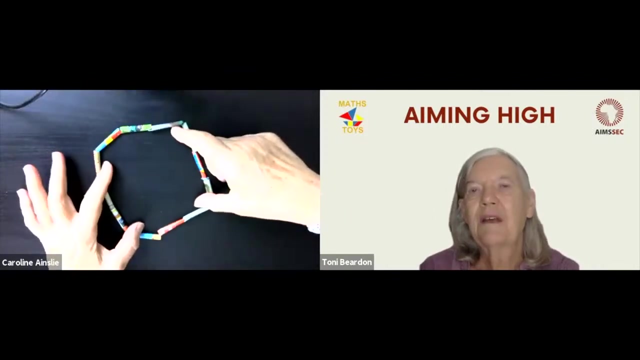 of identical faces coming off it. So every single vertex has four triangles And only four triangles, no more, no less. So Caroline's going to show us another puzzle here, And here she's starting with 12 edges. Again, 12 little sticks. 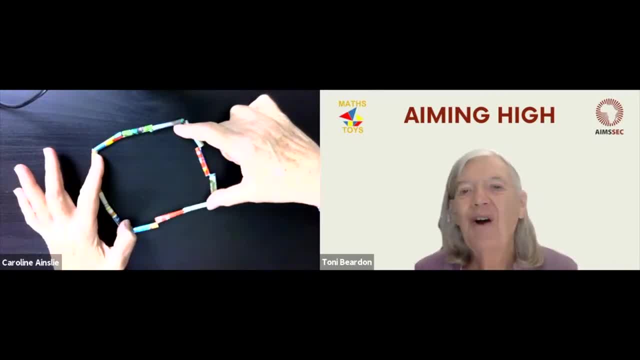 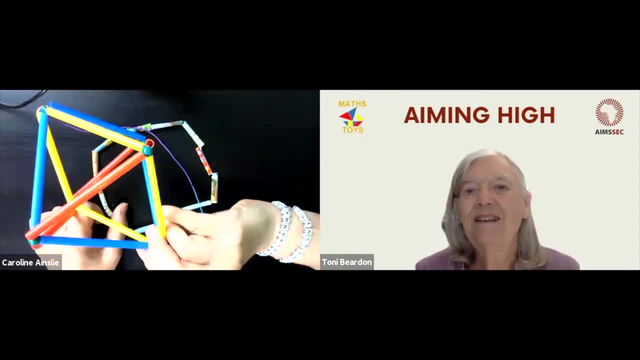 each of which is going to form the edge of her shape. But it's going to be another octagon, Yeah, another octahedron. We're making this shape, So this time I'm not revealing. It's fine Octagon for anybody that's forgotten. 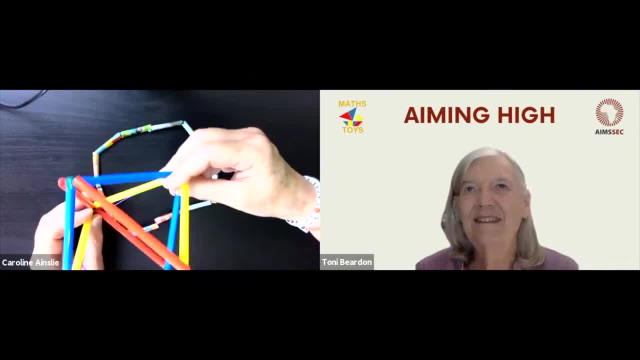 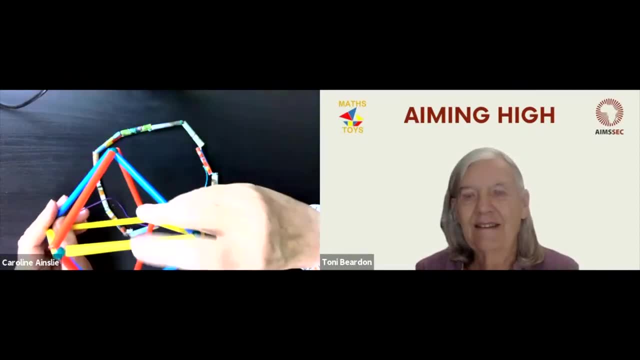 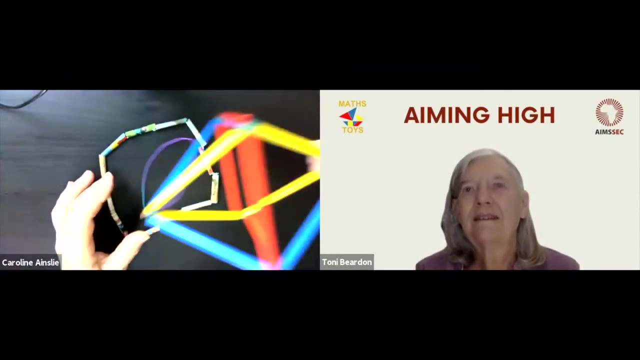 from when you went to school. octagon is a 2D polygon And octahedron- which I never learned- is the 3D way of referring to a 3D shape that's made up of polygons. So the thing with this. 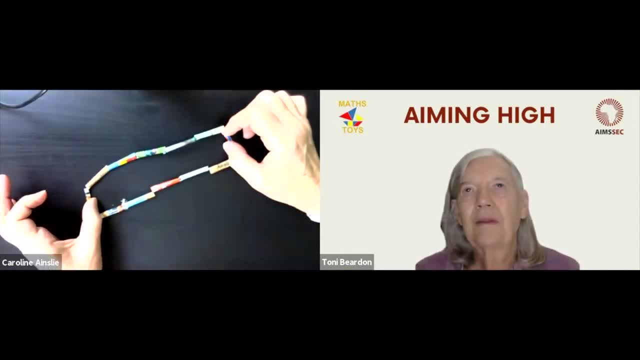 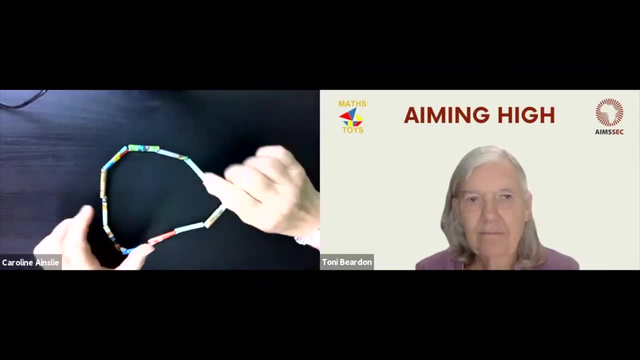 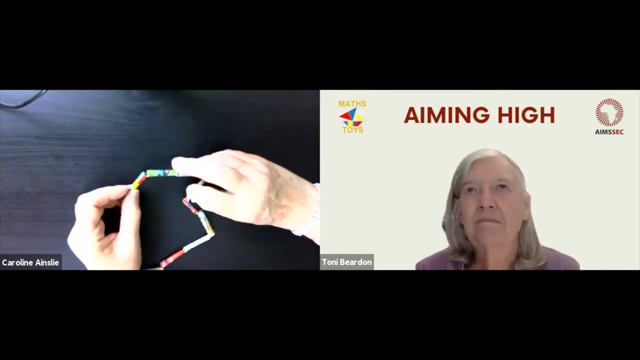 is that this is a closed loop. There is no opening And you can't. This puzzle must be made by using a closed loop. Now you can use elastic if you want. It might make it a little bit easier, But I'm using just recycled materials. 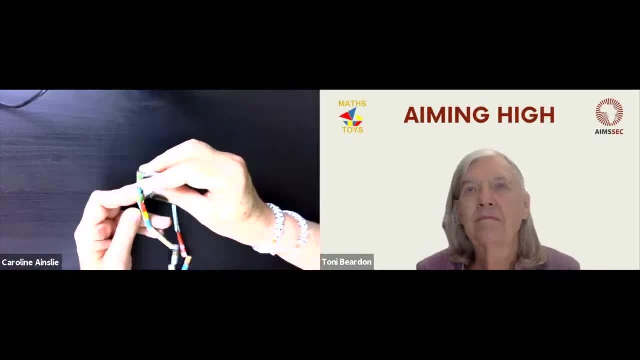 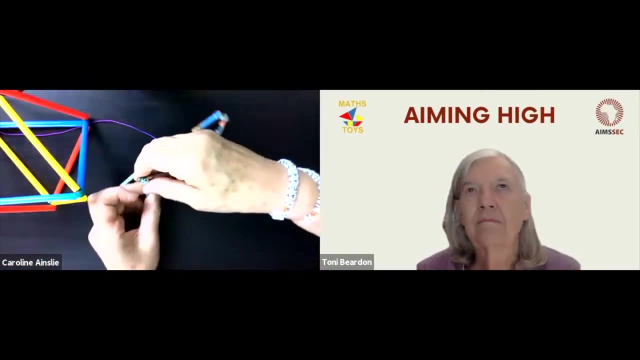 so string, sticky tape and an Aldi magazine. So what I'm going to do is I'm going to start with: This is the shape we want to make. I'm going to start by making triangles. That makes sense, doesn't it? 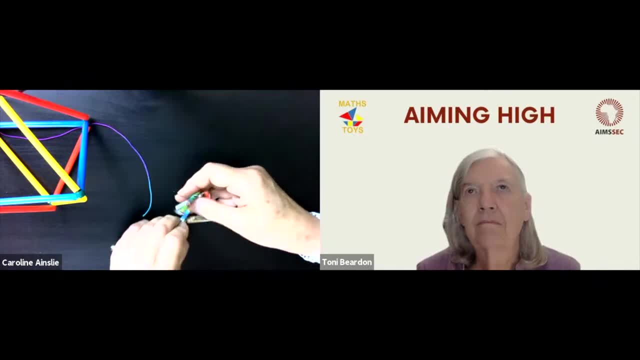 So I've got one triangle, two triangles. Oh, if I loop, If I didn't loop that quite enough times, Here we go. This is much easier with balloons, by the way. believe it or not, It's a lot easier with balloons. 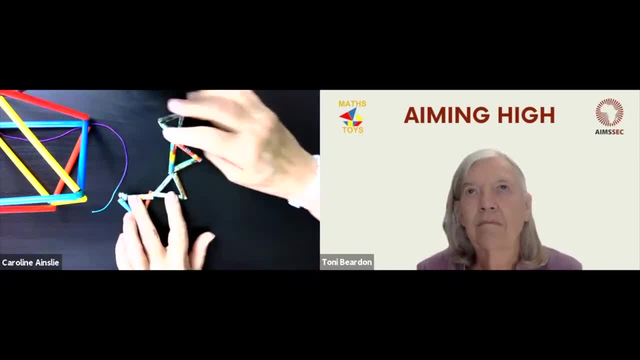 Three triangles And I've got four triangles. Oh well, I've got four triangles, But again we're in two dimensions. This is flat on the table. I've got four triangles. Well, can we go from having four triangles? 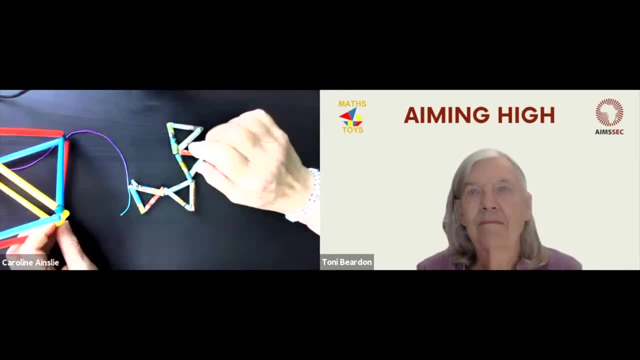 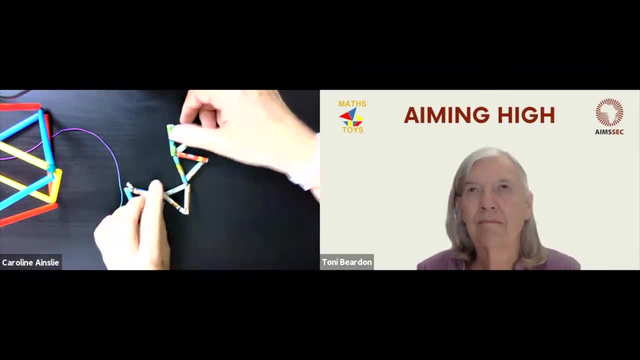 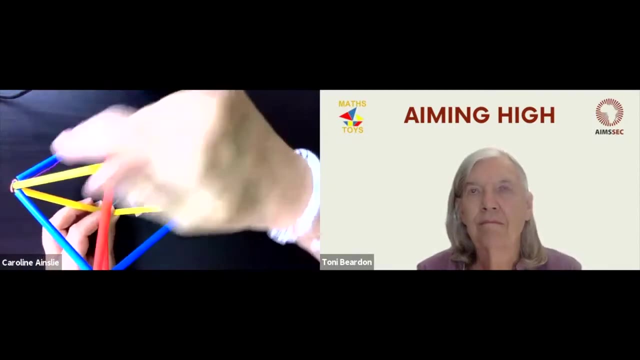 to having eight triangles without adding any more sticks, without Without adding anything. Well, you might have to add some string to hold the vertices together, But what do we know? We need to make sure that every vertex has four edges or four triangles on it. 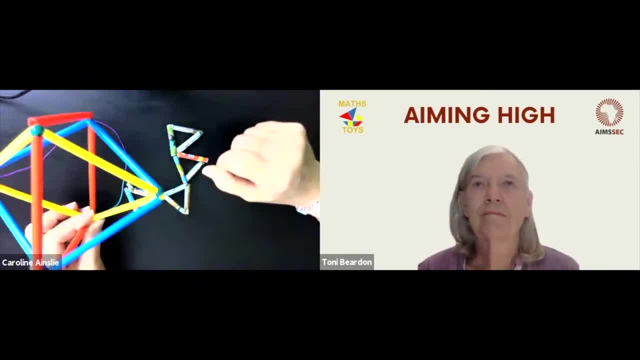 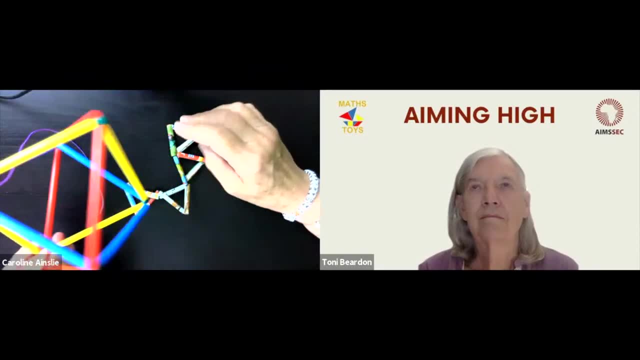 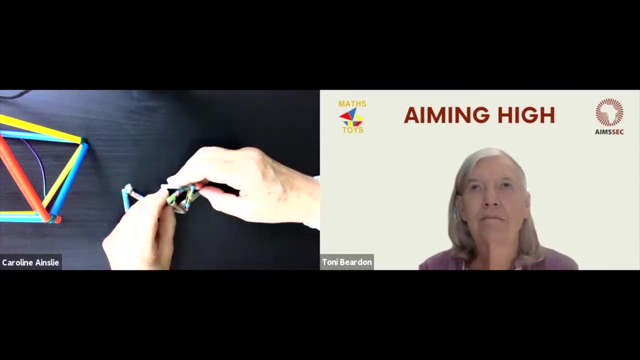 and not more and not less. And we need to only have, We need to have- the four squares, the three squares- I should say We know it's three because we made it this way. So you can- I was, You can- start putting them together like this: 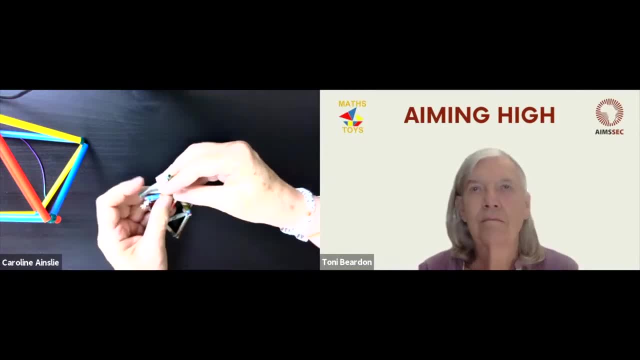 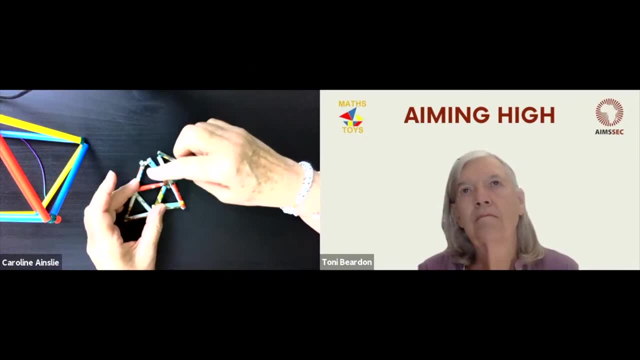 We're going to make a triangle there and a triangle, Oh dear. Ah, wait a minute. We can't join those together because we don't have four edges or four triangles. We've got six edges. Well, that's a clue for us. 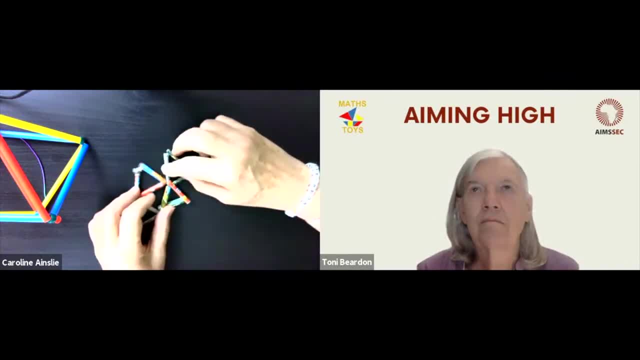 We don't. We have one, two, three, four triangles, But we've also got gaps here And we've definitely got six edges. So we know we're not on the right track there. So that's not it. Well, we had a clue here. 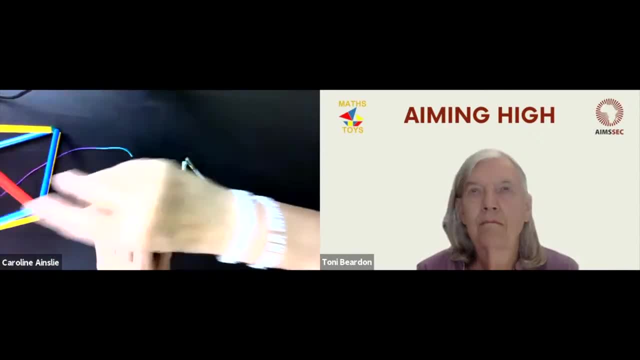 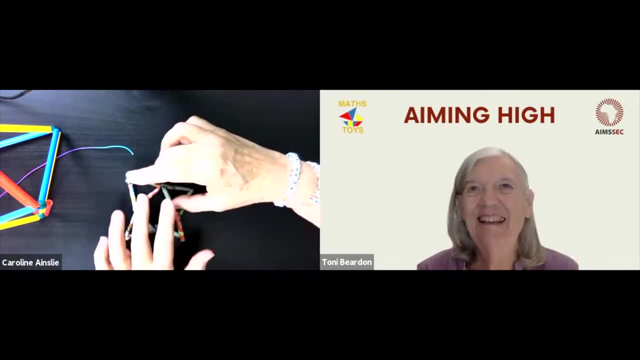 We made this up as squares, So let's see what happens if we make squares. Oh, that's interesting. This is looking hopeful, Definitely. Oops, Let's see if you can see the whole thing. It's definitely looking hopeful, Hmm. 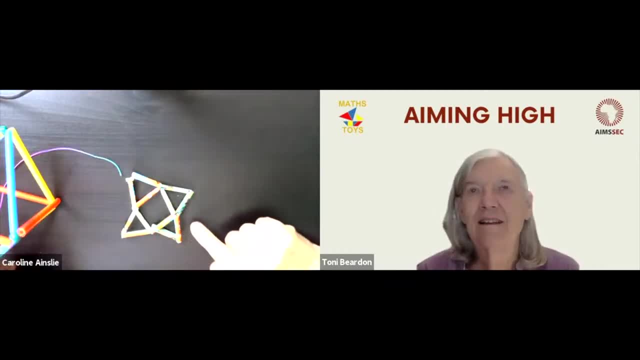 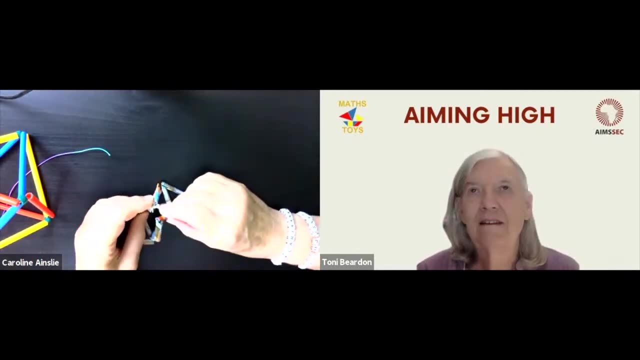 Now, how are we going to go from? We're going to visualise how to go from this to this. Well, let me bring two of them together. I'll bring two of them together. Ooh, we're halfway there, Caroline. 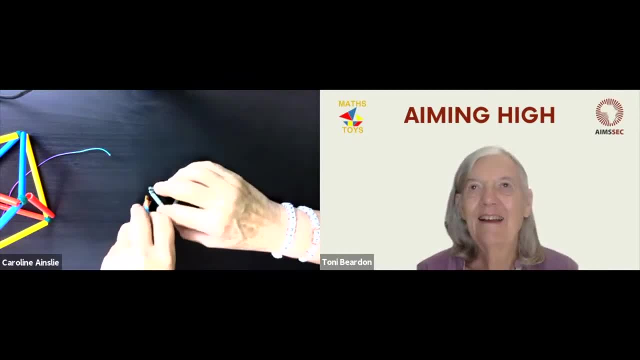 I think so. I think we are. If only my fingers were invisible. that would be so helpful, Actually, if we use a green screen to make my fingers invisible. And now, if I bring the top two together and the bottom two together, 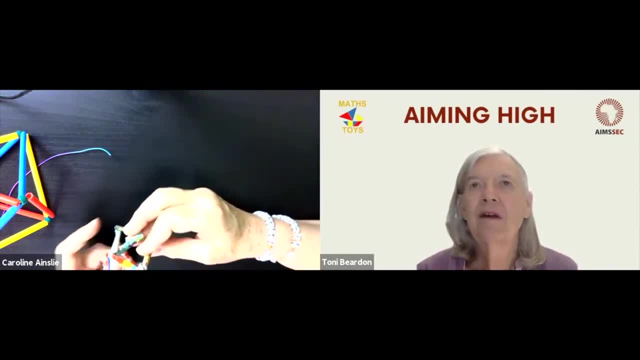 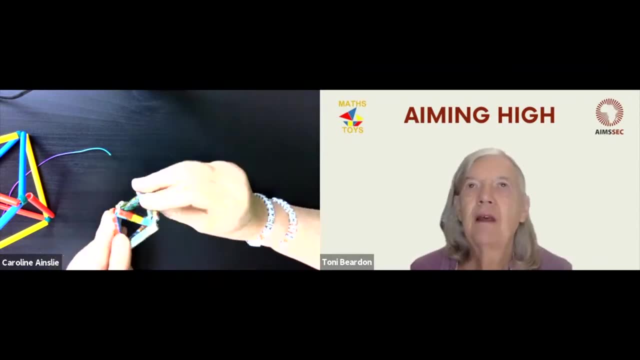 I just need. All I need now is some extra hands, Exactly Extra hands and invisible hands, so that you can see That's so pretty. Yes, And of course you can do it with longer sticks and if you've got two people together. 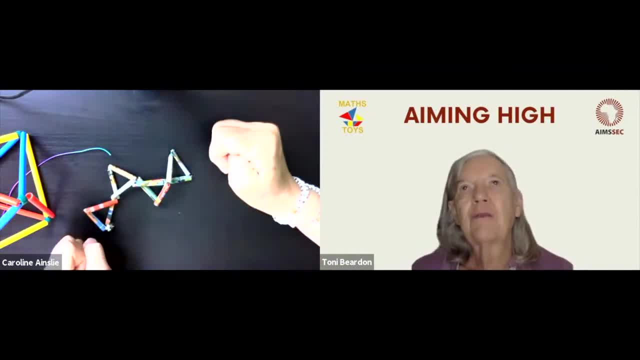 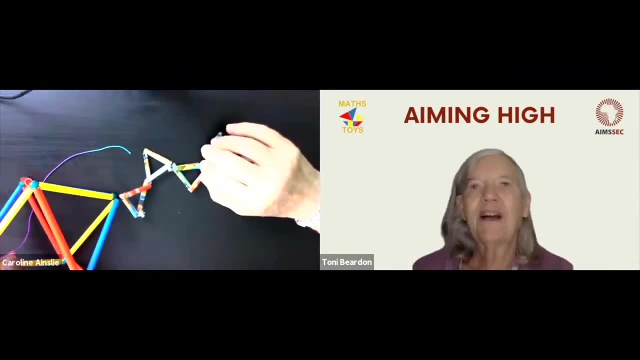 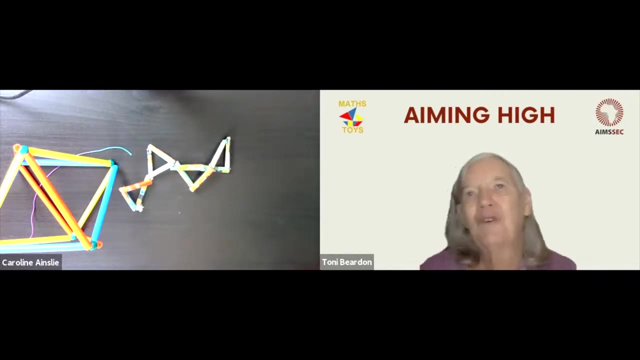 it is easier. But the four triangles around the square is your, is your clue. And then two triangles going up from the square and two triangles going down from the square and you've got your octahedron. The reason why I made it so small. 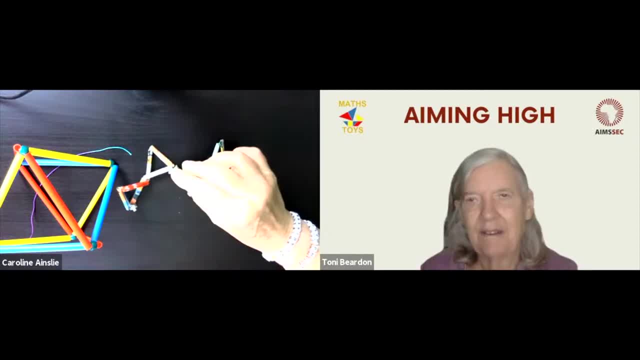 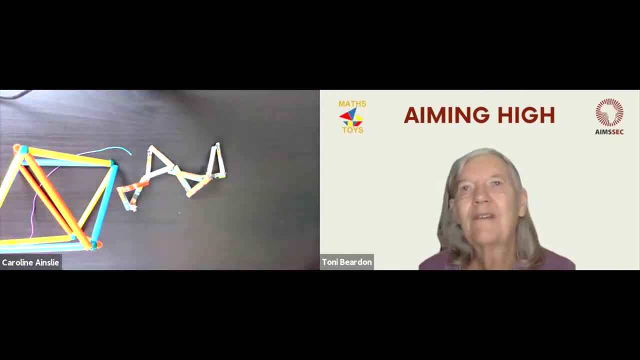 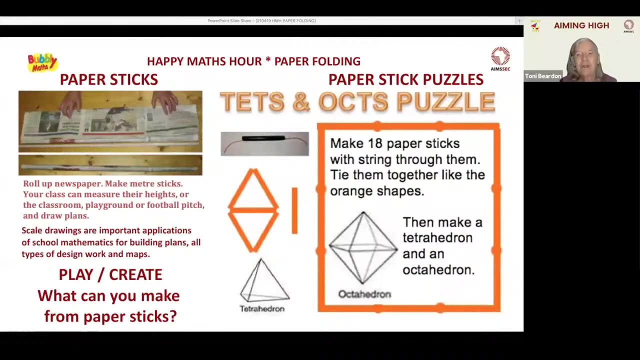 is so that you can see it on the visualiser is definitely easier to do if you're using larger, longer sticks. That's. that's a great puzzle. I really like that one, Caroline, And there's a lot of mathematics there to. 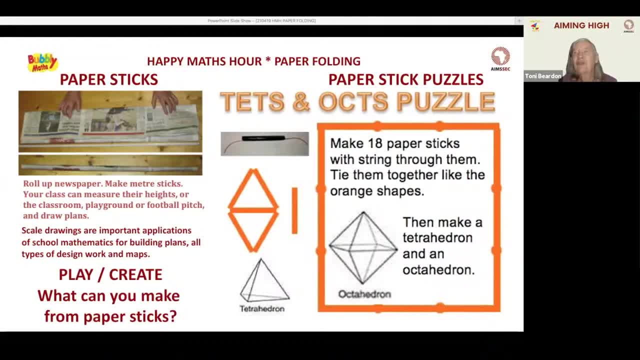 to talk about, to learn for the children- actually Not for the teacher to tell the children about, but for the children to discover for themselves And have lots of surprises and lots of victory moments where they're working things out and making discoveries. 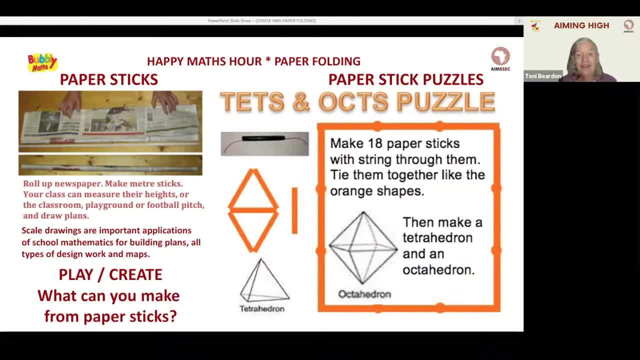 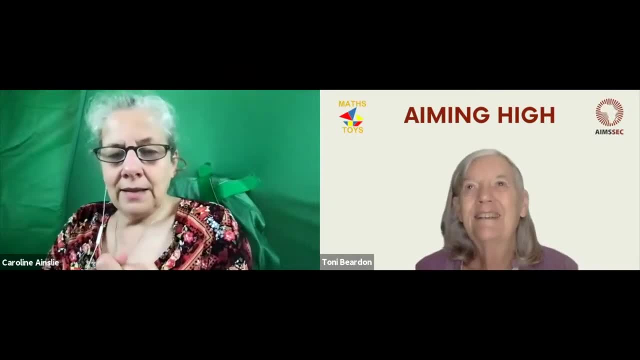 And we've got the tetrahedron- tetra being four and hedron being faces that we made, and the octahedron- octa- being eight and hedron being word for again, word for face, The way I present that. 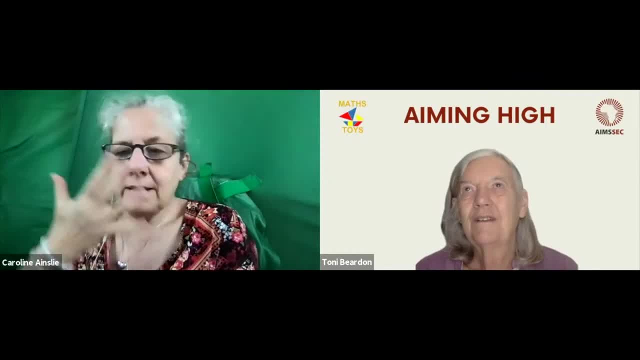 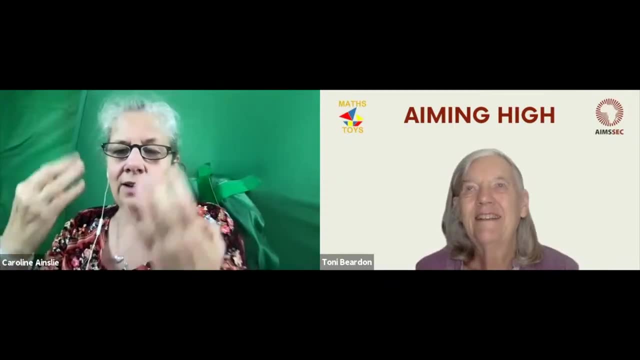 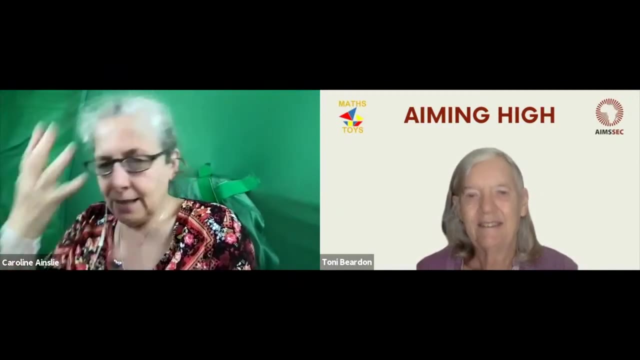 is tetra, meaning four faces. so tetrahedron for faces- and you're learning ancient Greek here- and octahedron, and it's a reminder that octa means eight, hedron means faces. OK so, And there's many more ideas. 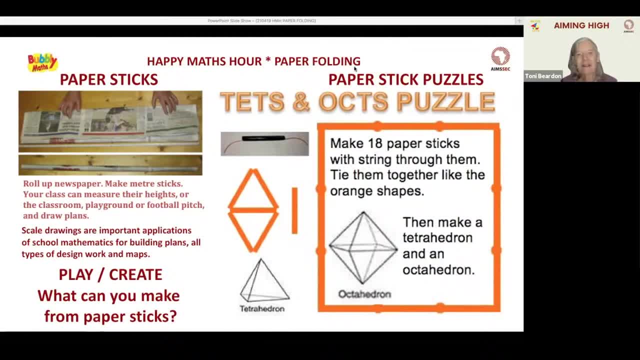 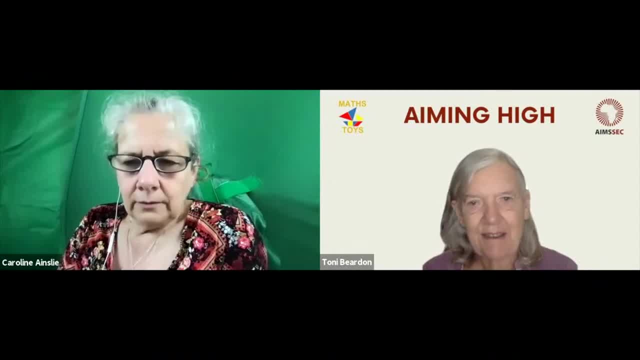 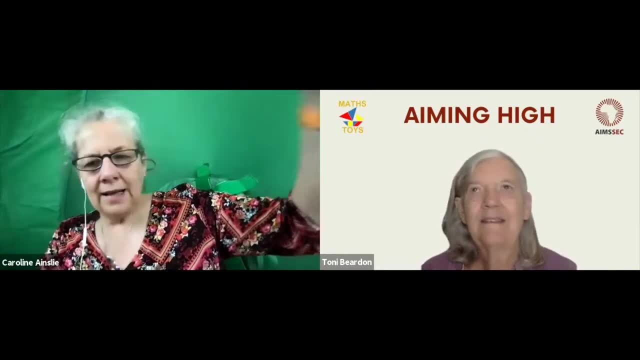 There's many more ideas on the Aiming High website for activities with paper sticks. Wonderful, versatile paper sticks. I'm just going to mention the the bendy quad. It's a fantastic activity. You make a cube out of sticks and there's so much you can do with it. 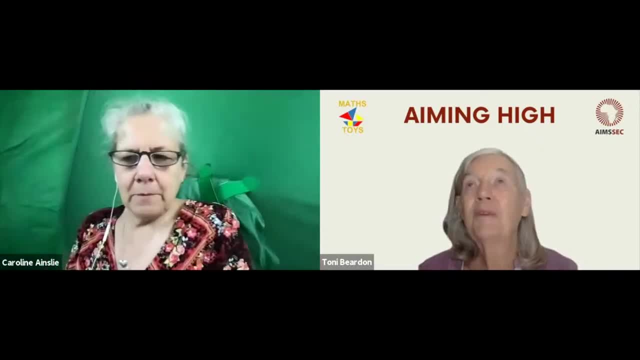 So definitely look up the bendy quads: one Bendy cube, and there's a bendy quad as well. Oh sorry, There's a bendy quad. That's right, And this is the bendy cube. Thank you. 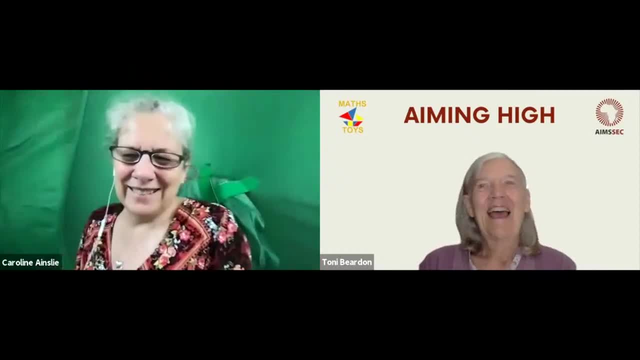 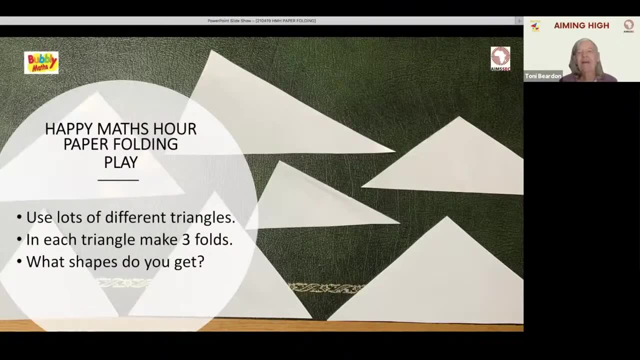 It's a bendy, hex And OK. so paper folding- We're going to get into some paper folding now, folding triangles, But Caroline really is quite a lot involved with early years. This is preschool activities for children to play with shapes. 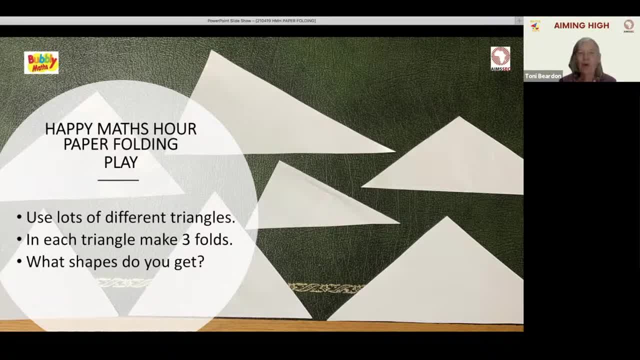 Not a serious, not seriously being taught mathematics in any way, but just playing with shapes, talking about the, what they see, what they're doing, having fun and building the basis for later mathematical learning. So So, yeah, so they literally. 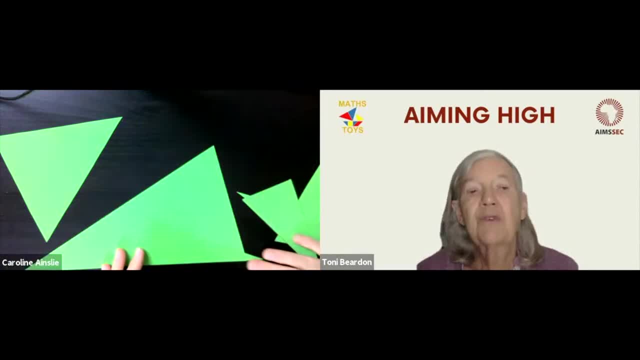 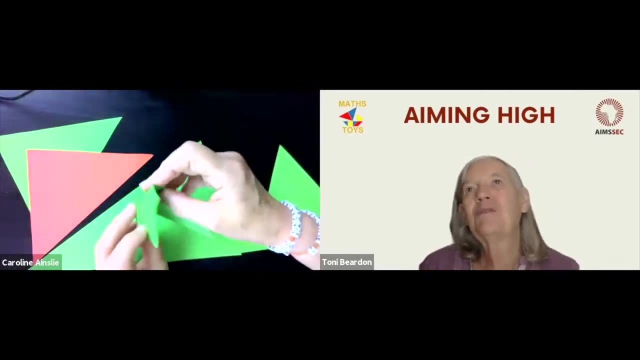 for early years, just get lots of triangles. So you say to the children: fold the triangles, see what you can make. And then, as they make different shapes, you don't necessarily tell them anything, You just don't ask questions. You say: 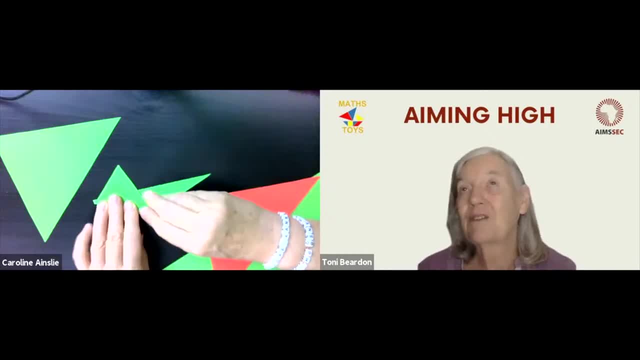 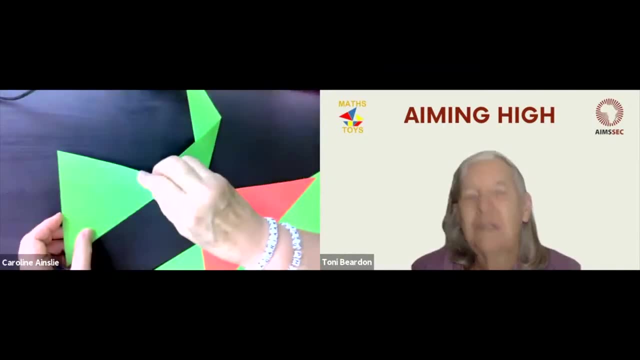 oh, you've made a triangle, You've made two triangles there. You've made What's that shape? Oh, my goodness, Isn't that an interesting shape. And talk about the different, the different things the children's actually doing. 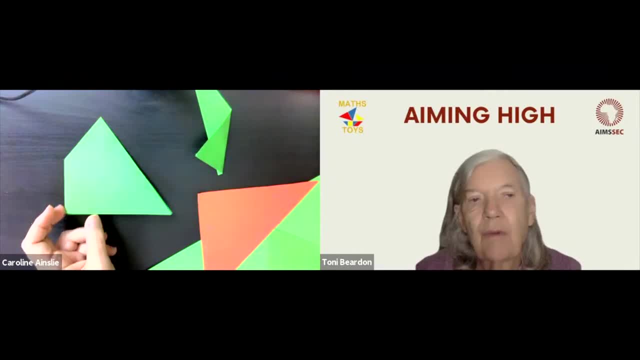 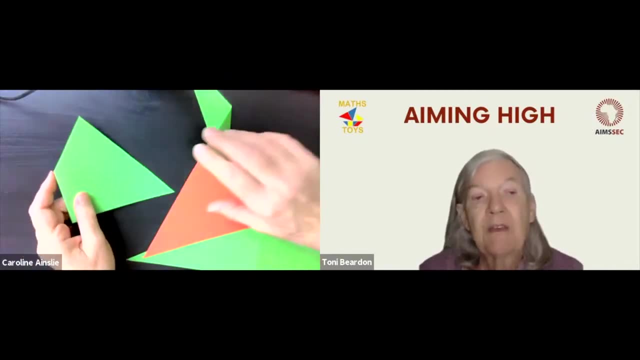 And only as long as they're interested, not continue. if they get bored and want to turn their attention to something else, Leave it. Maybe they'll come back to it another day. So what we like to do is to talk about learning at home. 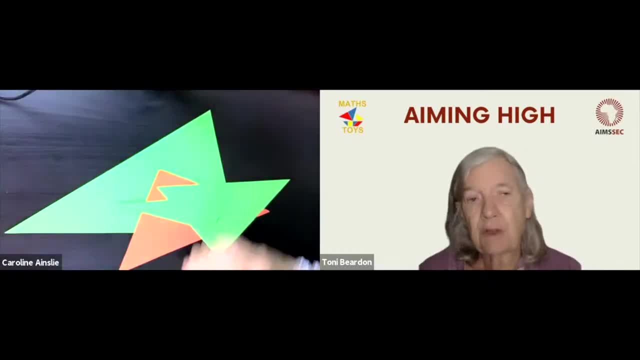 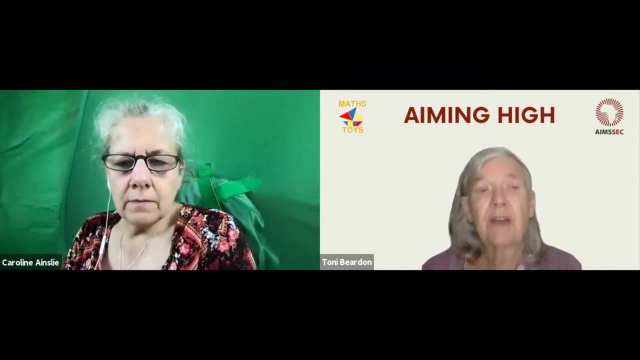 helping parents not just with very small children but especially with the lockdown and children not being in school, Children of different ages in the same household. So we introduce starter activities everybody can do together and then different activities for different age groups In a minute. 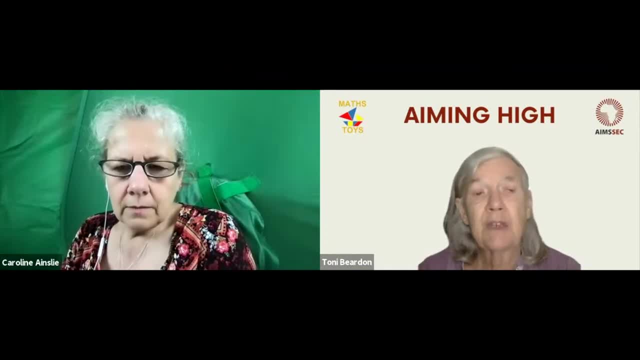 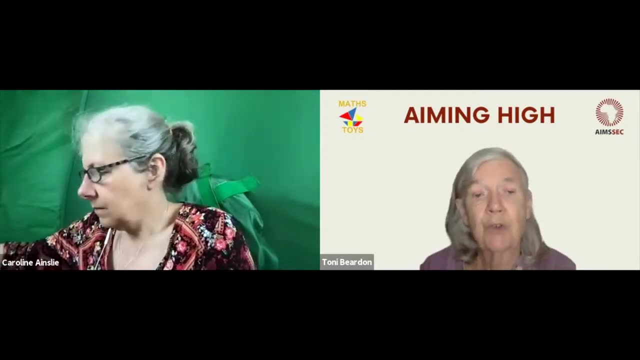 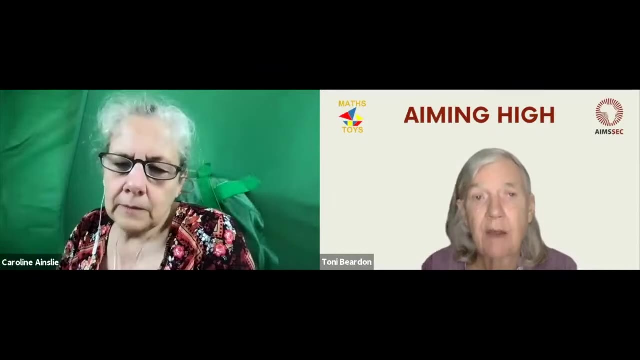 we're going to talk about the trifold activity and start with everybody doing something together, And then the very small children can do this, playing with triangles, and older children can get involved with more activities with trifold While the older learners are doing trifold. 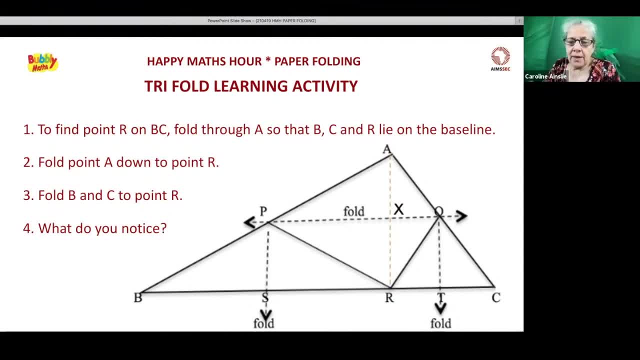 the younger learners can copy, They love to copy and they can do whatever version of trifold they come up with for themselves, And it's all good because it's all exploration. Now, here there's an enormous amount of maths, geometry, in this one activity. 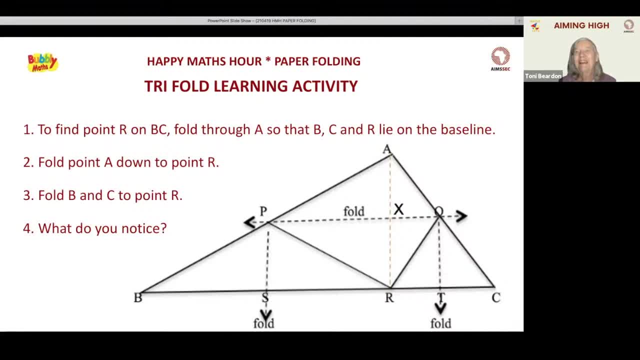 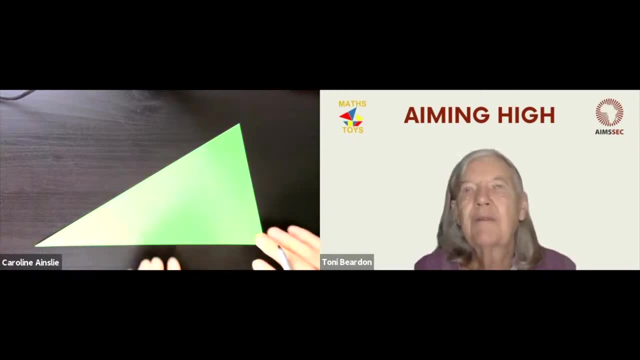 and all you need is a piece of paper. It's great, And I'm going to tell Caroline what to do, step by step, and she is going to follow this activity, Okay, So, first of all, Karen's got her triangle. Any triangle will do. 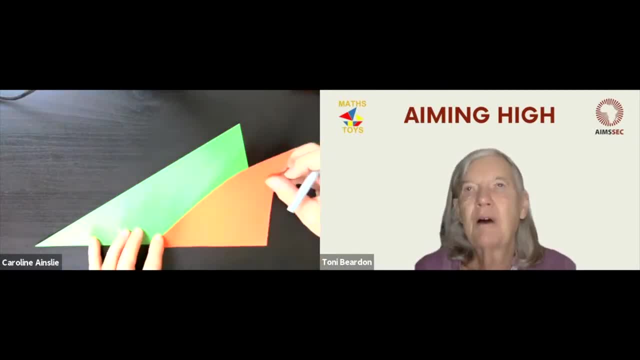 It doesn't matter what shape it is And she's going to. It's not. That's a right angle triangle. I just want to make absolutely clear. It's any old triangle, Well, it could be right angle, but the point is that it works. 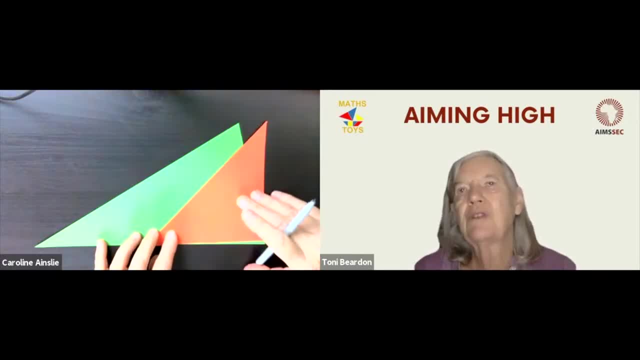 whatever the triangle is- And we're just showing you, with not a special triangle, but just any old triangle, And if your learners do it, let them all make their own triangles- I'm going to show you how to make a triangle, to start with. 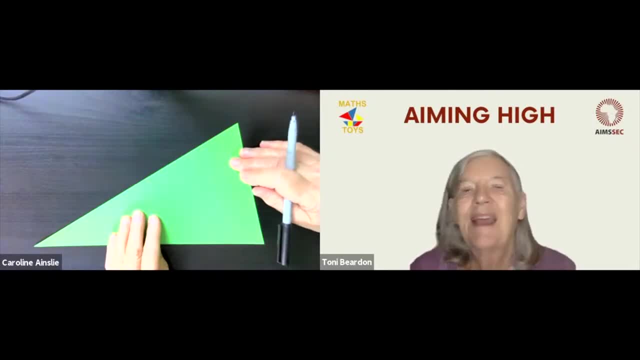 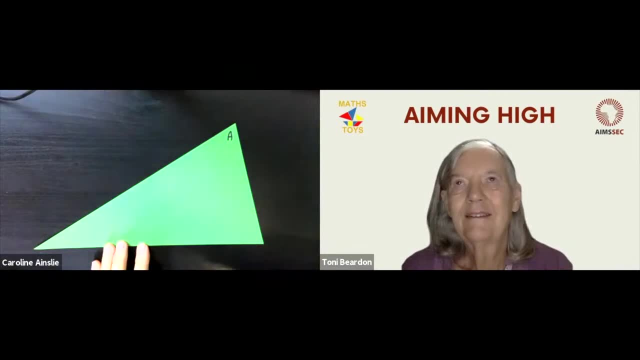 And so everybody in the class will have a triangle with different angles. Now Caroline's going to mark A, B and C at the three vertices: A, B and C. Are those big enough? Can you see them? That's beautiful, Caroline. 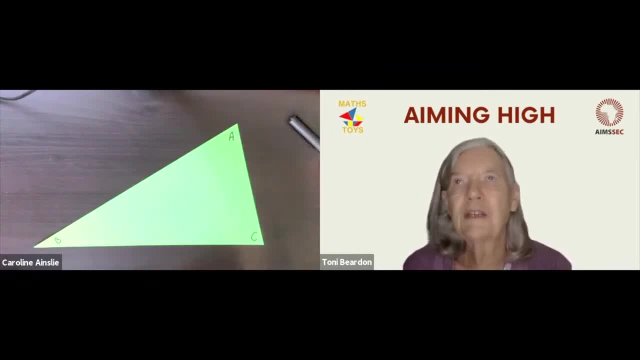 Now Caroline's going to make a fold through the top vertex A And the fold line is going to be down to the base and at right angles to the base. Now, to make sure it's a right angle, she's going to fold the point C across. 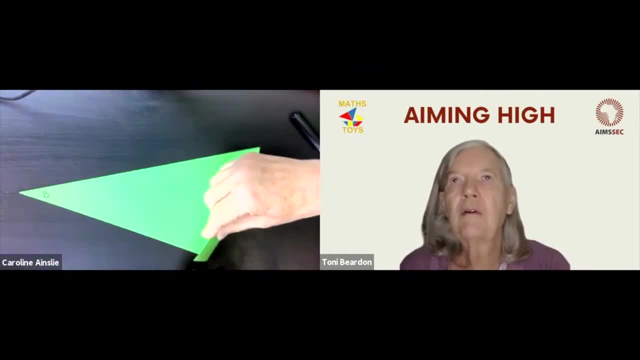 so that C will be on still on the baseline and the fold is going to go through A. So she makes that fold. This is the hardest fold to do because the A must remain a vertex. It's got The fold. has got to go right exactly. 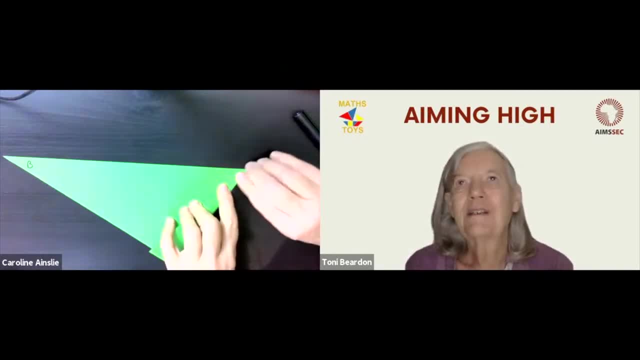 and precisely through the vertex there. Yes, And it is definitely the hardest one to do. I think I've got it. Actually, the more obtuse the angle, the easier that fold. OK, So brilliant. So now the line. 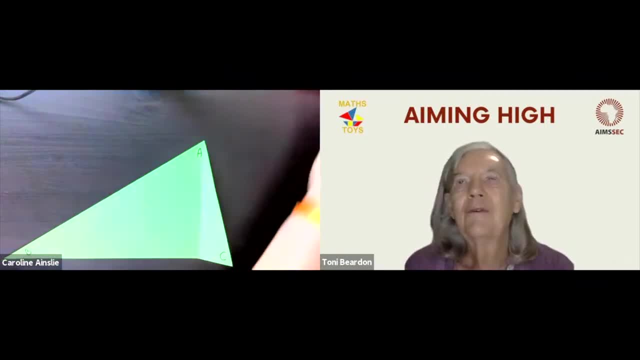 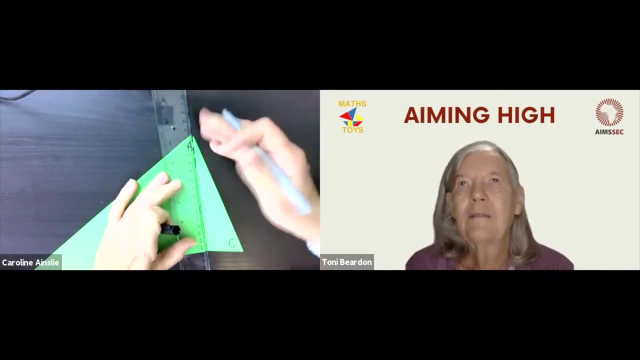 Caroline, if you dot it so that we can see it, The fold line is a line that's perpendicular. that means right angles to the baseline B, C. When Tony said the more obtuse it is, it means if that angle was more open. 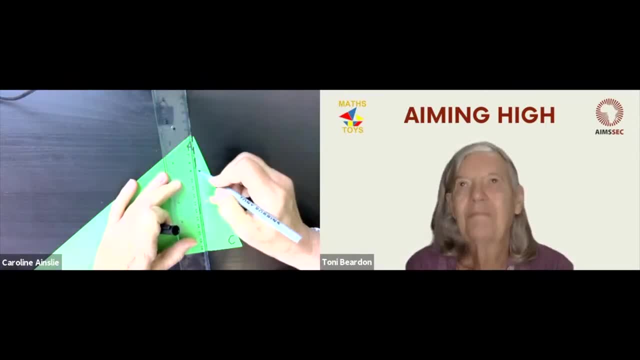 it would have been a much easier fold there. Bigger- yes, Bigger- angle. What did Yeah? So now the On the base there. that point is called R, So if you'd like to write R there to remind ourselves when we talk about R, 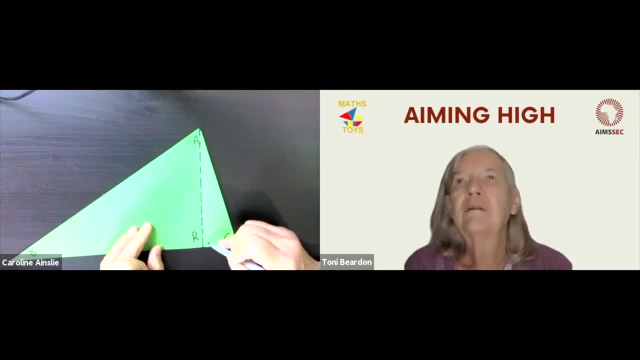 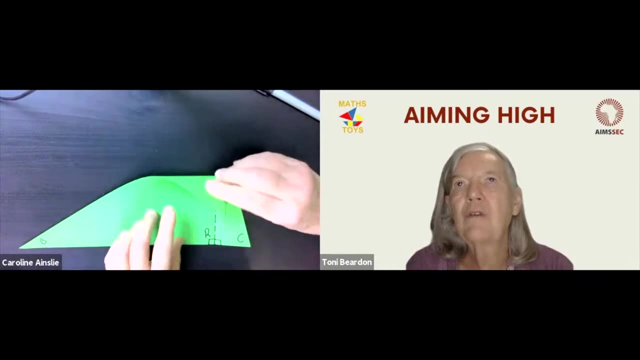 that's the point we mean. Can I mark that they are right angles? Yes, you can do. Yes, OK, So now fold the point A down to just the vertex, just on the point R, and make a crease there. 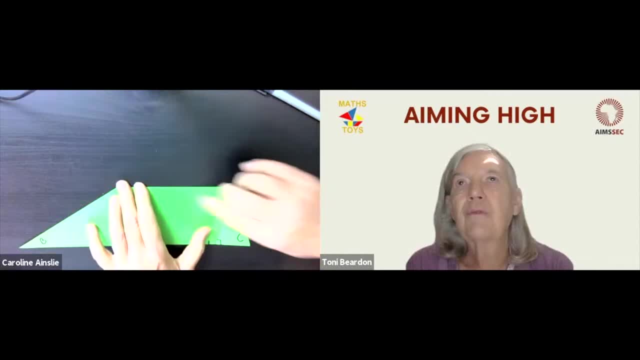 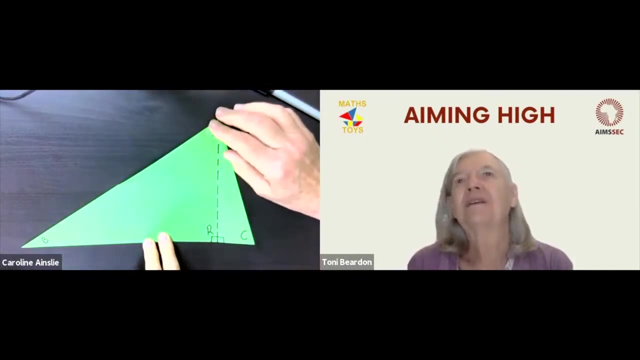 Now it looks as if the fold line that Caroline is making is actually parallel to the base. Now we can't assume anything, but in fact it is. It is parallel to the base and that's something that is quite easy to prove. 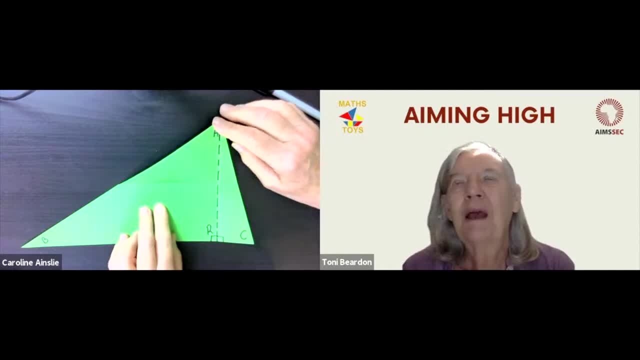 geometrically, you know, formally, in the geometry, It's only parallel to the base, because we started off with a line that is perpendicular to the base, which is why that positioning of point R is so important, Absolutely. Now. Caroline's now going to fold the point B. 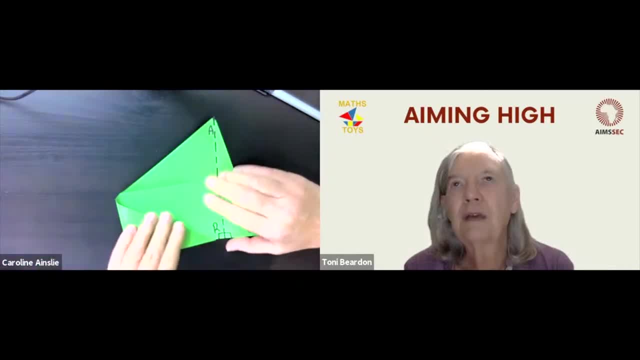 across to R, as she did with A, but this looks a little bit different. So there Again a little tip to help you. I'm using really thick markers. so that you can see what I'm doing, Use a nice thin pencil. 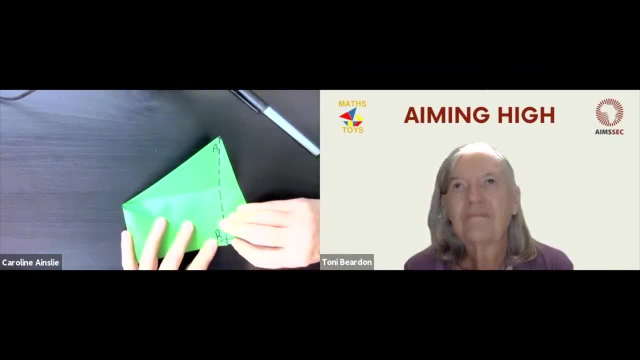 because right now I'm working out where exactly point R is and it's not very precise because I'm using a thick marker and that's not. Anyway, it'll do for the demonstration, but see if you can do Now. younger learners. 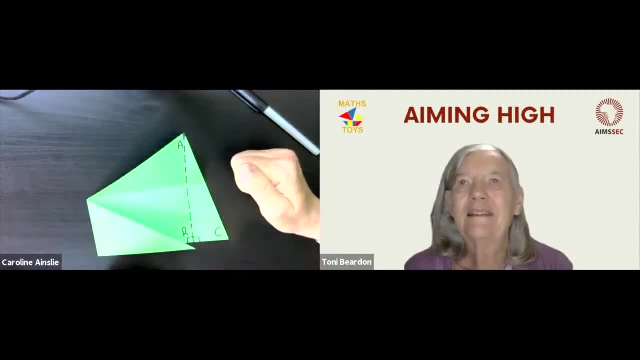 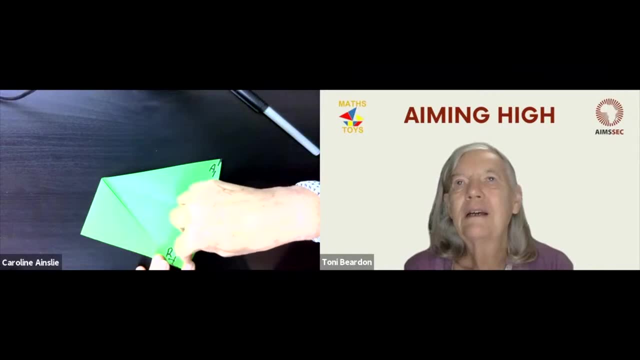 it'll make it quite higgledy-piggledy, but they'll still get the benefit from it. OK, Now do the same with C, Caroline, Bring C over to R as well, And So the vertex C has got to go. 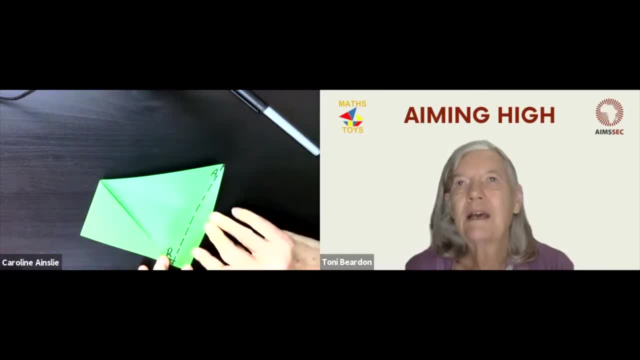 exactly onto point R, as you can make it, and crease that edge And bring the flap A down again. And Now, Wow, Wow. That's very neat and tidy, isn't it? And it appears that, Caroline, She's turned it over. 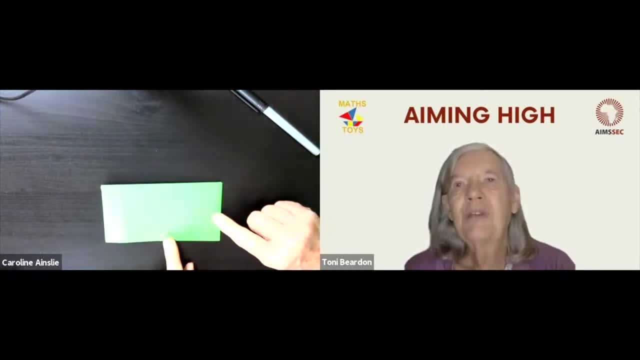 so that it holds in place. The shape that she's made by folding those three faces and the three flaps down is a rectangle, And Wow, There's a lot we can deduce from that. Now turn it over again, Caroline. 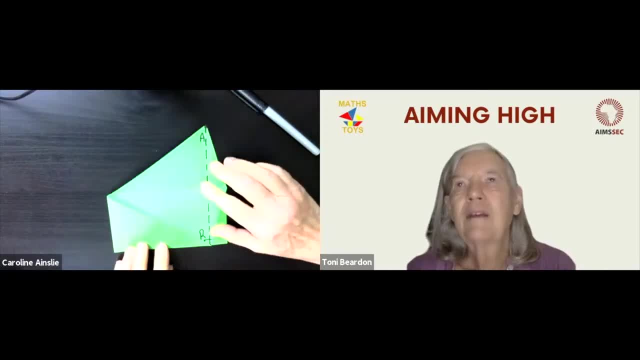 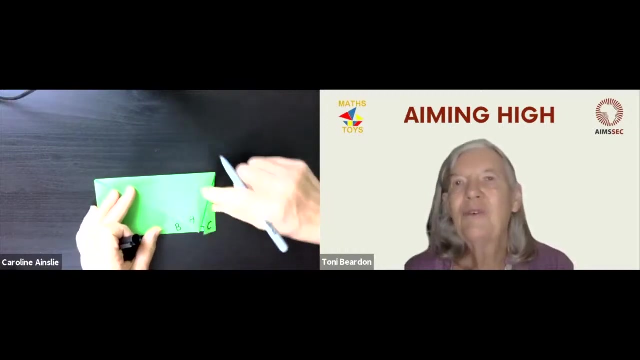 and see those three flaps coming together at that point at the bottom, Those angles A, B and C from the original triangle. Can I mark them on the back, A, B and C. And they fit so beautifully together. It looks as if. 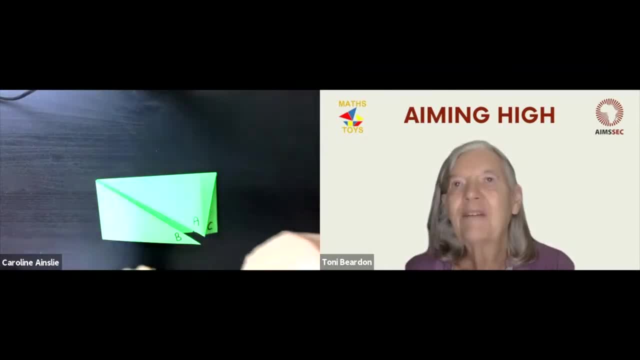 It's pretty convincing that the angles add up to 180 degrees. Now there you go. They've got a straight edge there, so you can see the angle on the straight edge is 180, and the three angles add up to 180.. 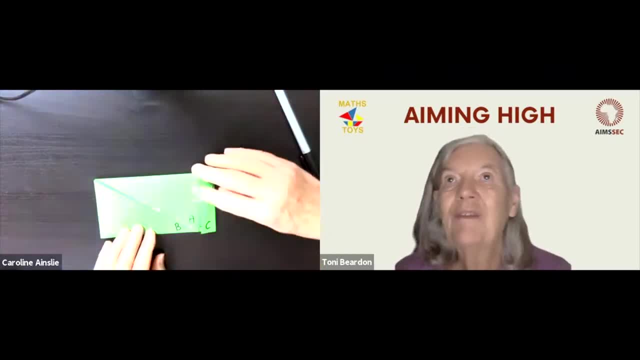 Now you can do that in primary school, And that's enough of a proof for younger children up to the age of 11, 12.. By the time they're 13,, 14, we want to begin to investigate the congruent triangles. 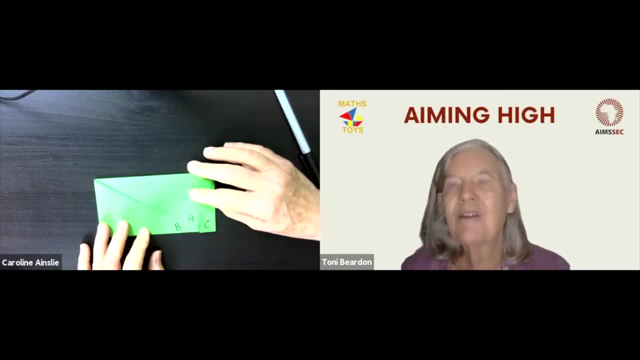 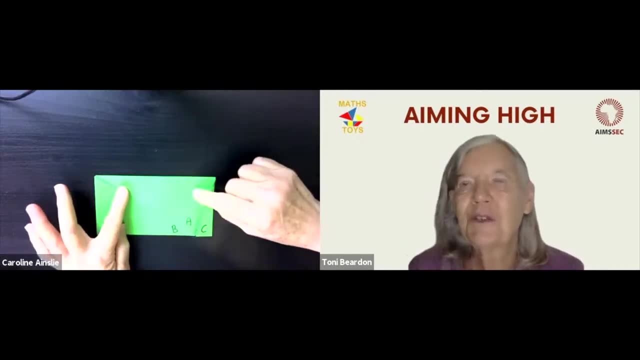 Congruent, meaning exactly the same. And they are the same if they fold on top of each other. Now, the little rectangle that Caroline's holding shows us that, the area of this rectangle, We can easily work that out. Now open it up, Caroline. 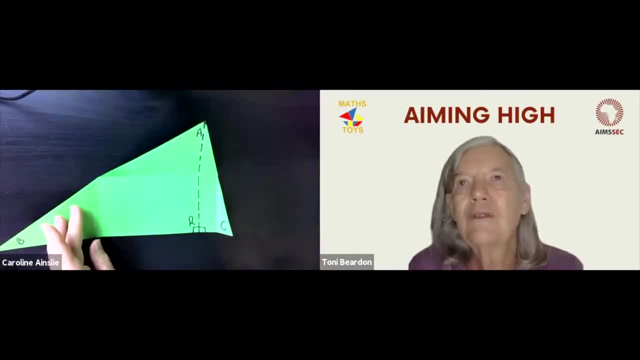 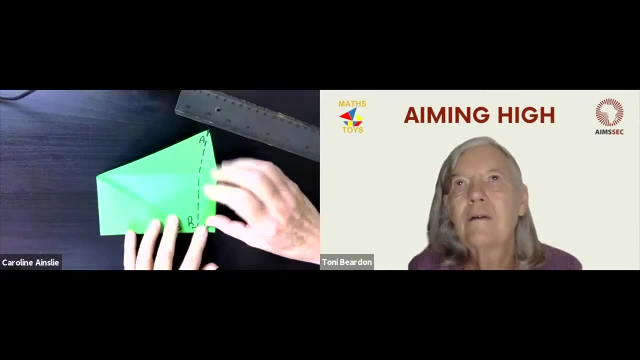 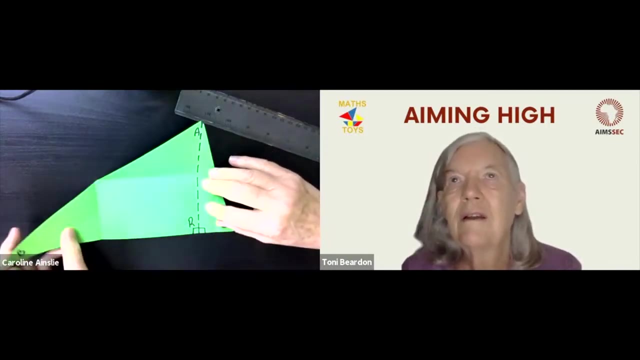 Now the triangle is covered twice when we fold the flaps in, So the area of the rectangle is half the area of the triangle. Oh, my goodness, So these three external triangles added together have the same area as the rectangle that they make. 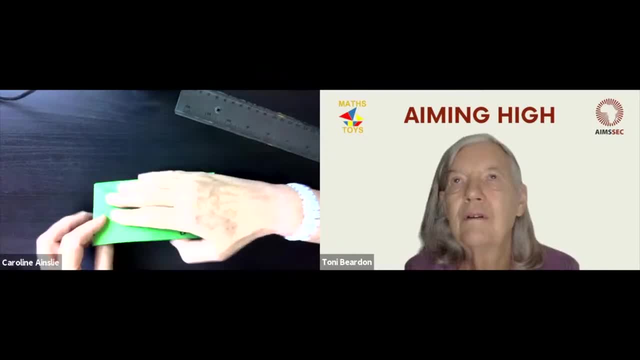 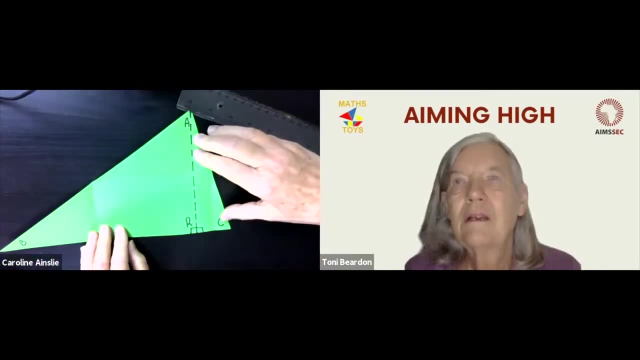 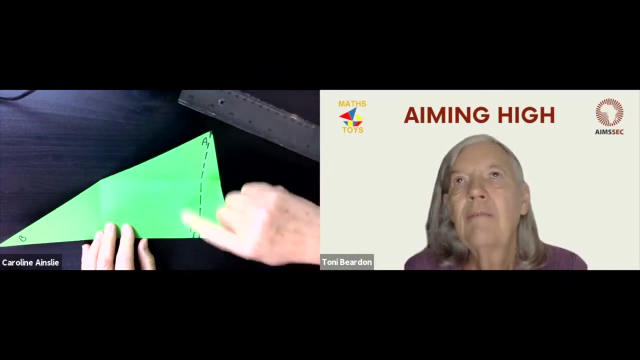 And there's a rectangle on top made out of triangles and a rectangle underneath. that's just the what's left of the original triangle. Yes, Now, because we can easily work out the area of the rectangle and because we've got these pairs of triangles. 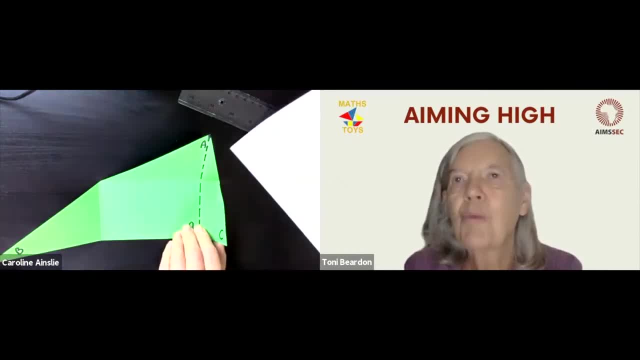 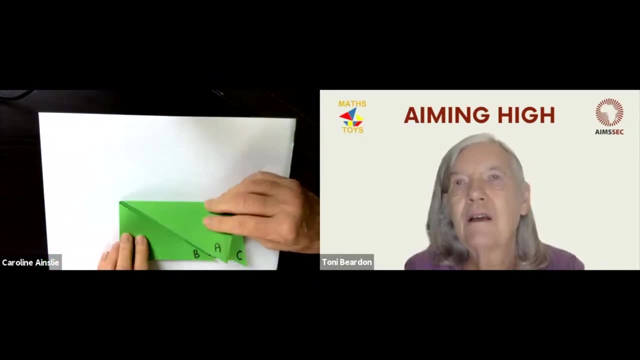 that are the same as each other because they fold on top of each other, and the mathematical word for that is that they're congruent triangles. we've got an easy way to prove that the area of the triangle is half the base times the height. 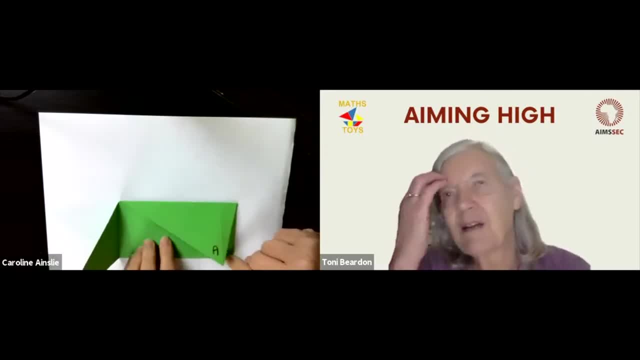 Now we won't go into that in detail now, but I think everybody can imagine that we can use that rectangle to prove that formula. So not only have we got a formula for the angles of the triangle that are 180, we've got a formula. 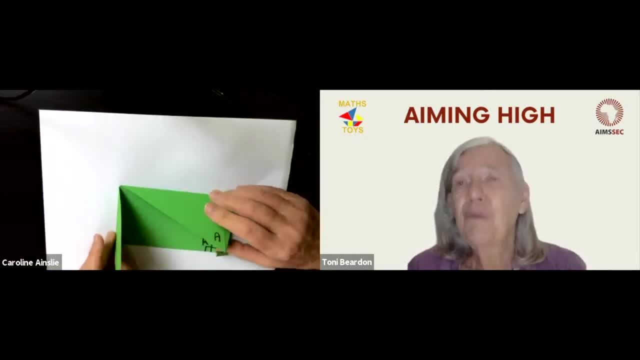 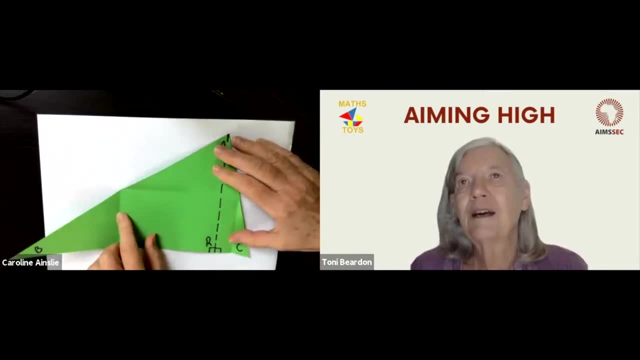 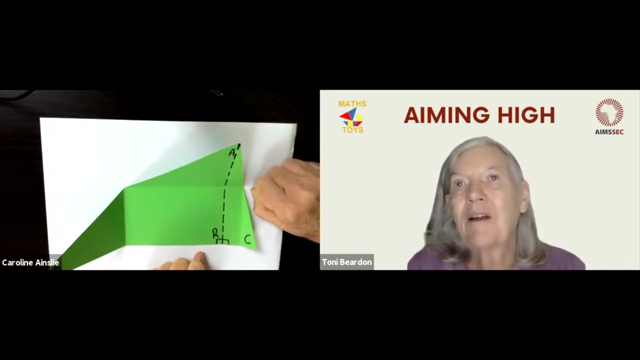 we've got a way for, we've got a proof of that, and we've got a way to prove the area of the triangle as half the base times the height. What we've also got is pairs of triangles that are the same and they. 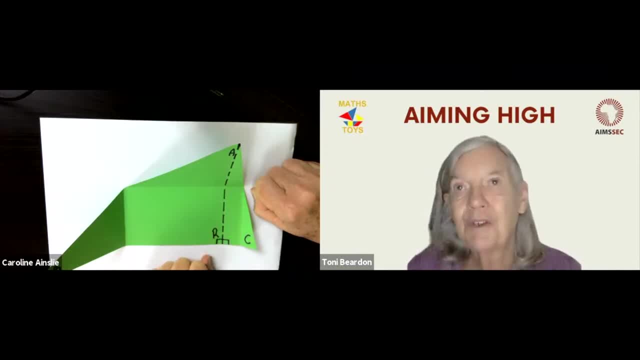 the same in the mathematical word is congruent. But we've also got- and we were just talking about it earlier- we've also got more symmetry here, so there's a lot that we can use this, just this simple paper folding exercise- for in talking about congruent triangles. 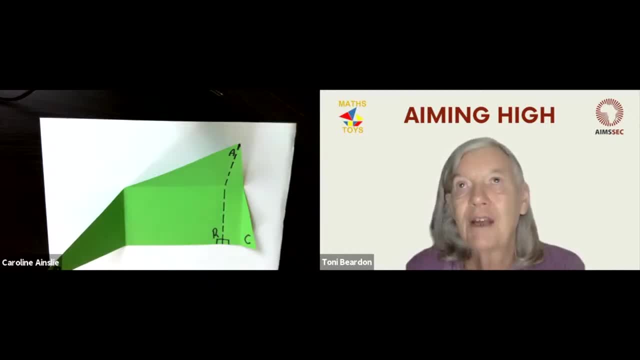 similar triangles and symmetry. I don't see any symmetry at all in this triangle. Well, Caroline, perhaps you would like to fold over one of those flaps with the say with the angle B on it. Now draw along that edge so that we can mark out that. 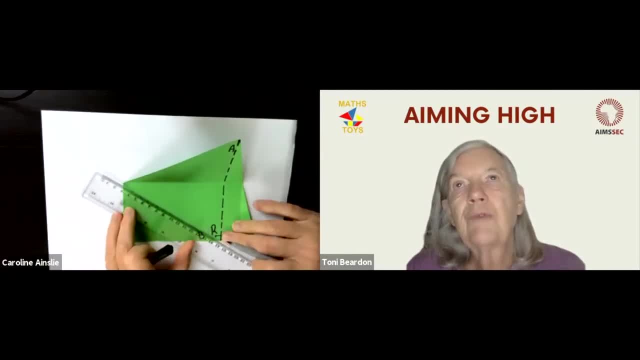 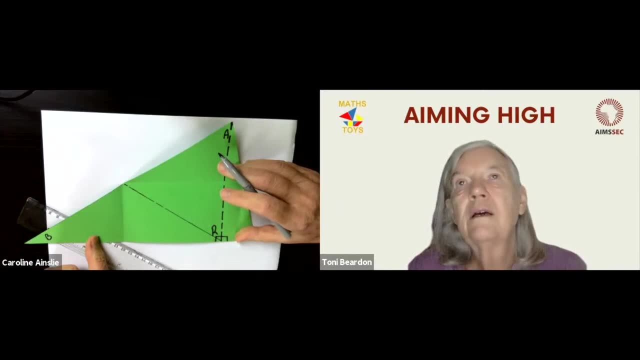 that's the edge. I meant, yes, Now bring the corner C. I've just seen something. OK, Now do the same thing from yes, then there. Is that what you're talking about with the congruent triangles? I am. 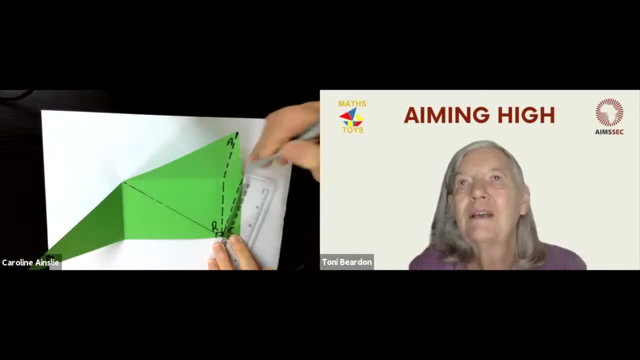 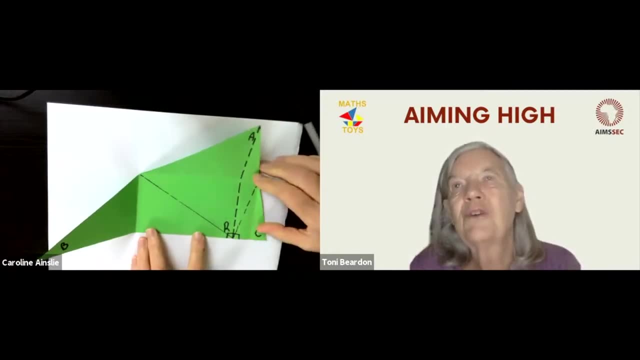 Ah, Right Now, what we like to do is to colour this as well. So each pair of congruent triangles is coloured with the same colour. So we've got three pairs of congruent triangles there. Wow, You could also draw in the vertical lines. 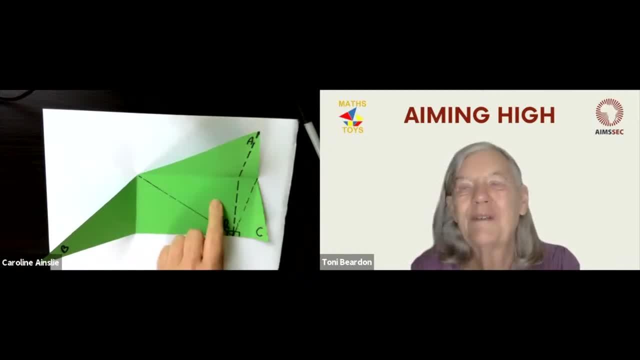 to show the lines of symmetry. on those. You've got lots of lines of symmetry, But of course this is a triangle. here That's a triangle. This is not a triangle, This is a quadrilateral, But the two congruent triangles 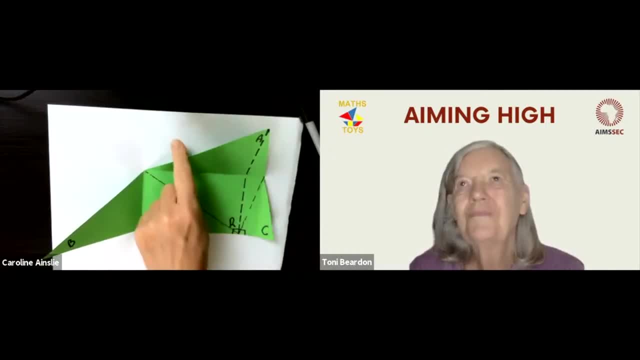 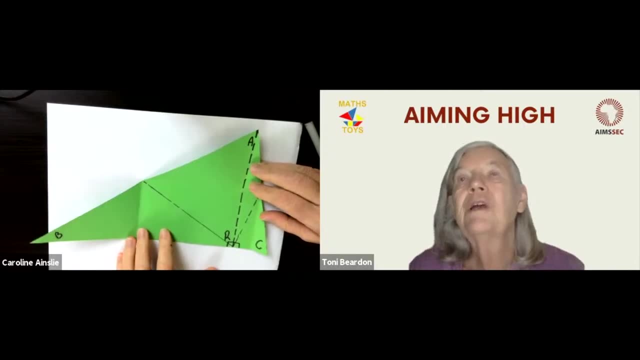 are symmetrical along that line of symmetry. So you've got a lot of symmetry there. You've got a lot you can do about congruent triangles. You've also got similar triangles. That's similar to the big triangle because the angles are all the same. 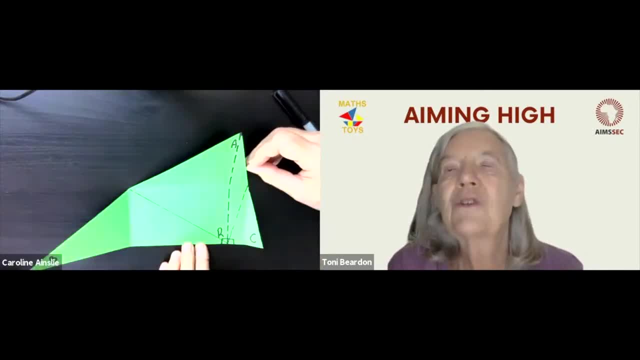 It's a smaller version of the big triangle, So there's a lot about similar triangles too. And that leads us into- for the older children, the 16 to 18-year-olds, into another theorem in geometry which they have to prove. 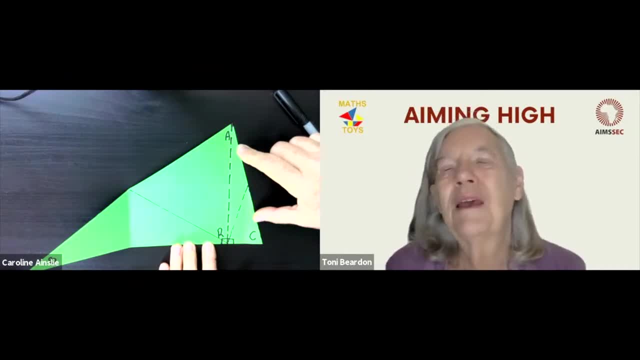 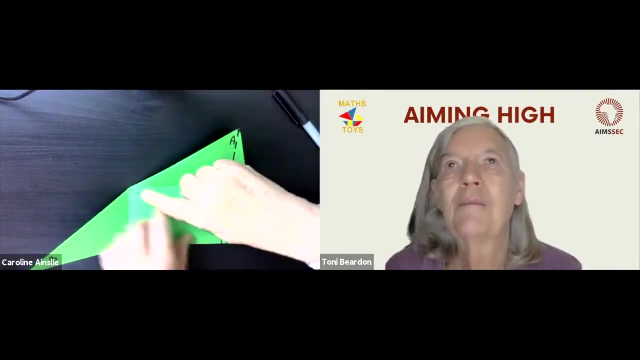 And the easiest proof of the theorem which is about a triangle, it's called the ratio theorem And the easiest proof is, using the similar triangles, that that top flap of the triangle with vertex A is similar to the bigger triangle. And OK, we'll leave it there. 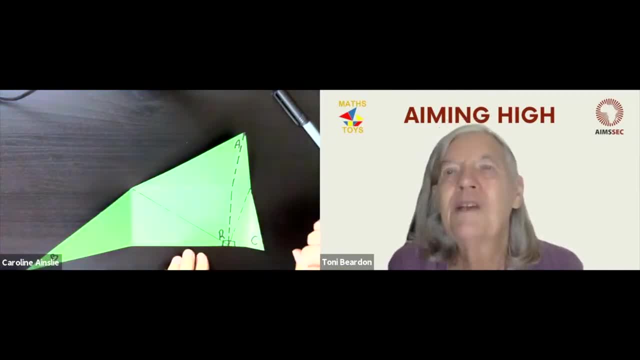 But there's a huge amount of geometry. So all the geometry is convincing when you have the paper folding exercise and you talk about it. But then you can easily, if you have to, turn it into a formal language of geometry and write a formal proof. 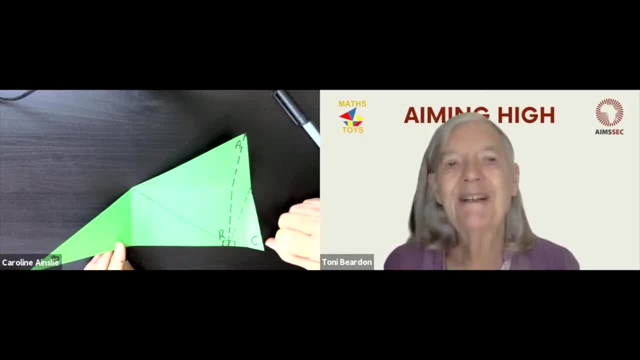 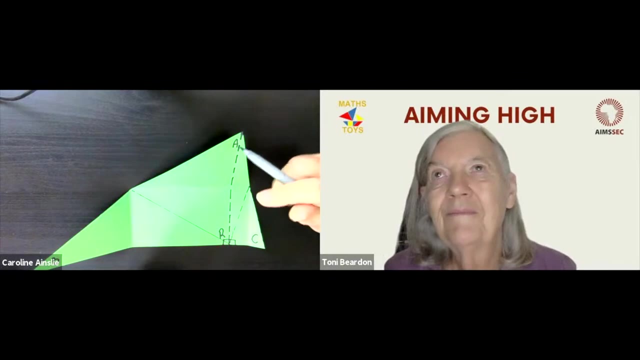 based on the paper folding. So it's a lovely, a lovely exercise which has ideas, and it relates to different geometry that's taught to different age groups in school. I'm completely blown away by how much there is in. All I've done is make three folds. 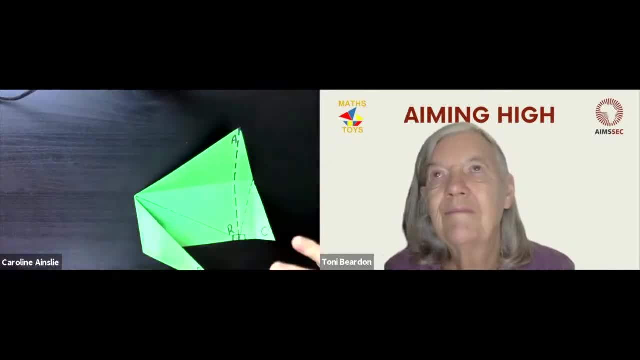 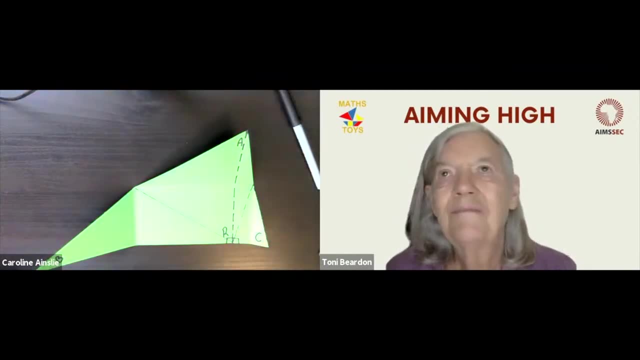 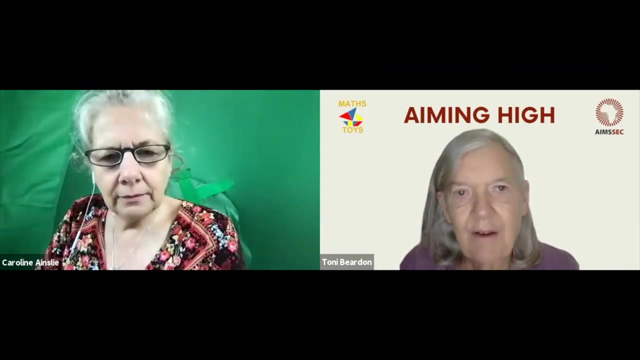 No, four folds, One there and three others, And there's so much in there. And then it's fantastic. What's next, Toni? Oh well, the next thing we're going to do and say goodbye to a trifold for now. 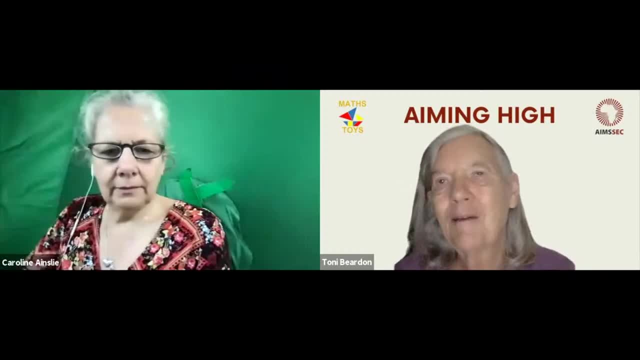 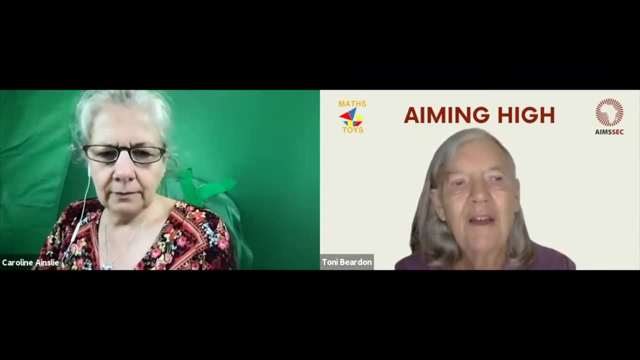 and go back to it please- is to have a look on the Aiming High website for our learning pack with lots and lots of ideas about trifold. And now we're going to move on to paper folding to get an angle of 60 degrees. 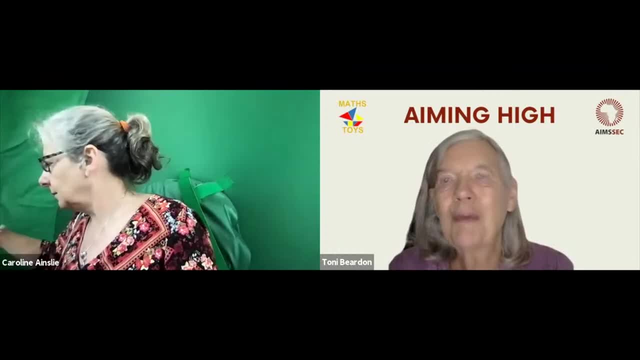 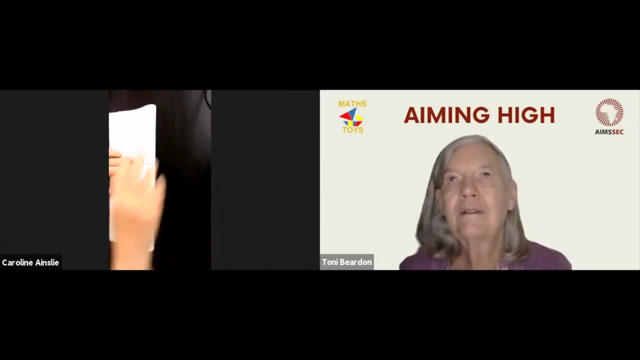 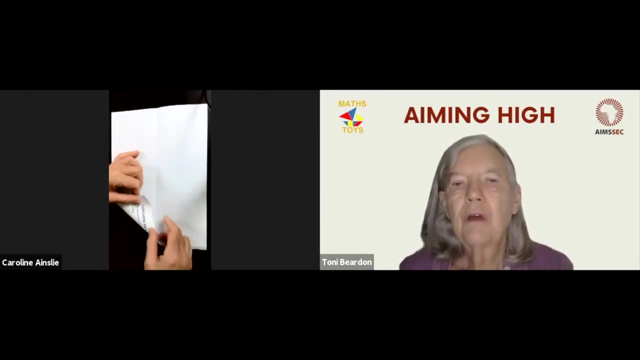 And all we need is an ordinary piece of A4 paper. Caroline is going to fold this lengthways in half And then make a crease And open it out. Then she's going to take the bottom left-hand corner and she's going to make a fold. 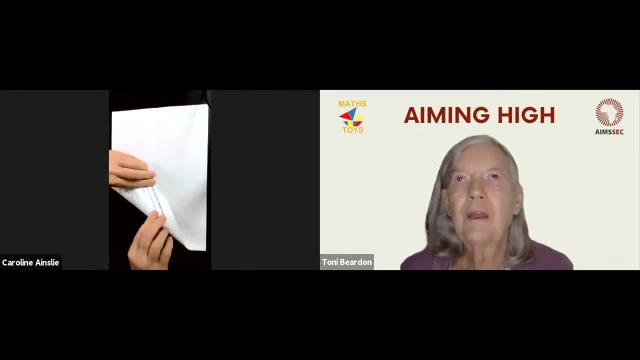 that goes through the bottom right-hand corner. So the corner that was at the bottom left-hand is going to go on the middle crease And again she's got to be quite careful to go exactly through that bottom right-hand corner. And when she's got it, 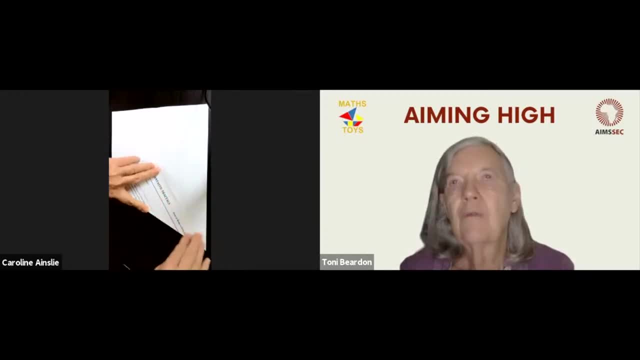 in the right position. she's going to make that crease And it's marvellous, but the angle that she's made is 60 degrees. Isn't that amazing? Seriously, 60 degrees, That's 60 degrees, yeah. 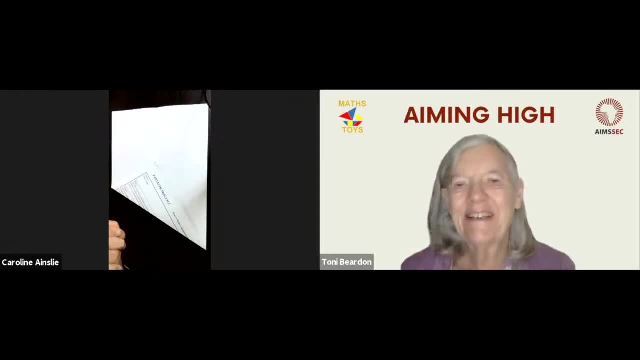 OK, Isn't that? It wasn't that easy Now. we'll Now make an equilateral triangle and then we'll talk about why it's 60 degrees. So now Caroline's going to take the top corner on the left and fold that down. 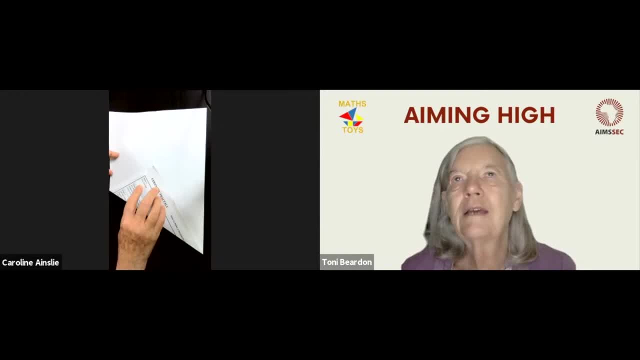 making the fold along the edge. Oh, yes, the edge. Show them, Caroline, It's where the paper was folded up along that edge. Fold this paper down And OK. And this edge wants to follow what is now the base of that triangle. 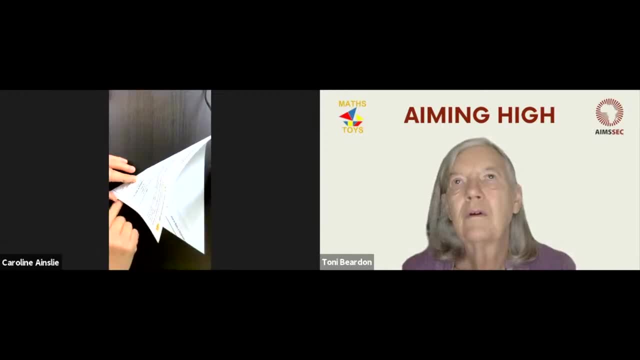 This edge wants to go on. the first fold that we made. Yes, And it's almost there. Turn it over, Caroline. You'll see that you've got an equilateral triangle with just a little flap which is going to just tuck in. 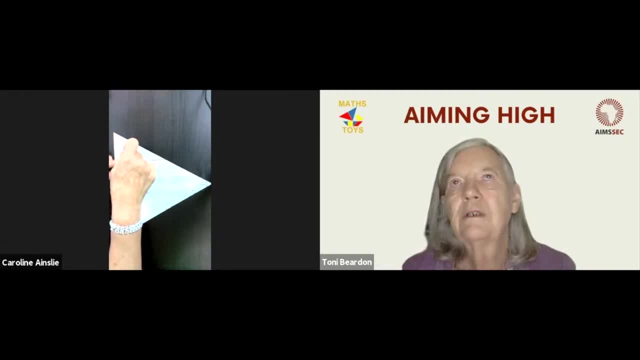 and get rid of. You can cut it off if you want, but there's no need. You can just tuck it in and it's gone, And that is now a perfect equilateral triangle. Yeah, OK, Yeah, and my mother's name is. 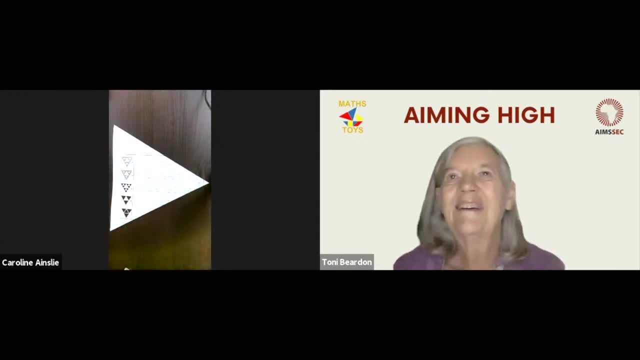 Seriously, Tony, a perfect equilateral triangle. All I've done is make two folds. It's amazing, isn't it? And even more amazing is that you can now easily fold each of those vertices to the opposite edge carefully, and then lift them up. 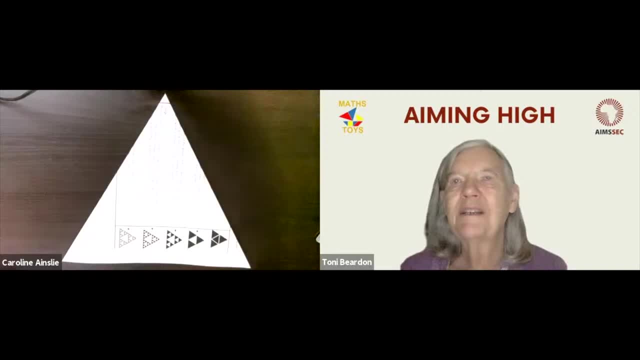 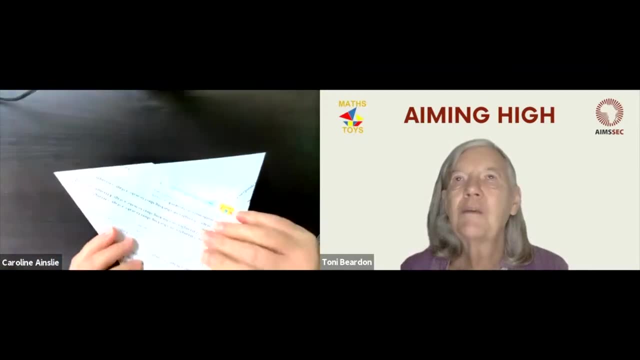 and make a tetrahedron from it, Right, OK, let's do that. then Each vertex goes to the opposite edge. Oh, I've got. Now I'll tell you what I've got. I've got a nice line here. 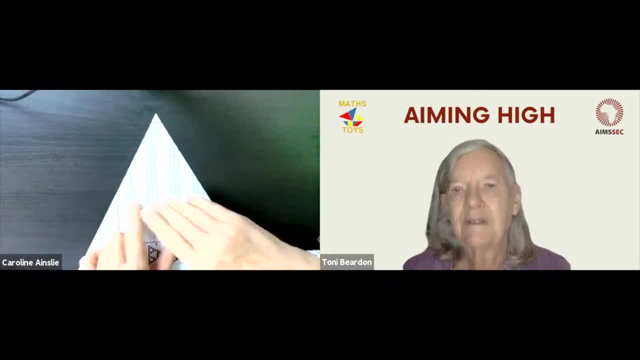 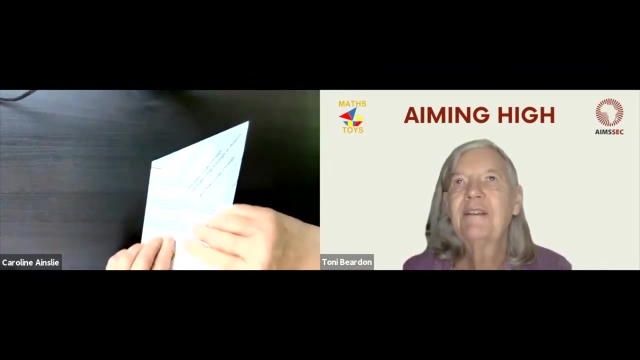 From the original fold where I folded the paper in half. I'm going to use that line and that's my fold line for the first one, so that I get it in the right place. So we're going to get four triangles folded on top of each other. 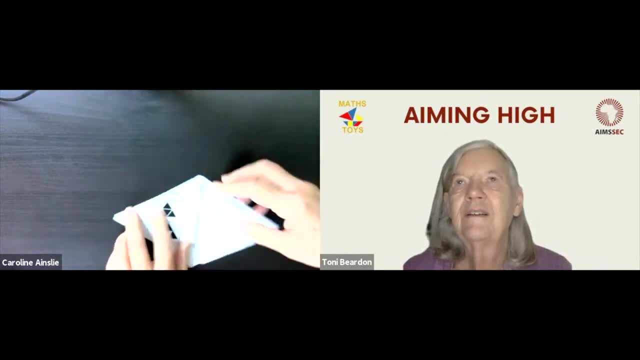 Again. such a simple activity. Look at this. They're all the same size. All four triangles are all the same size and they fold over onto each other beautifully. And you said that will make a tetrahedron. Yes, all you need is some sticky tape now. 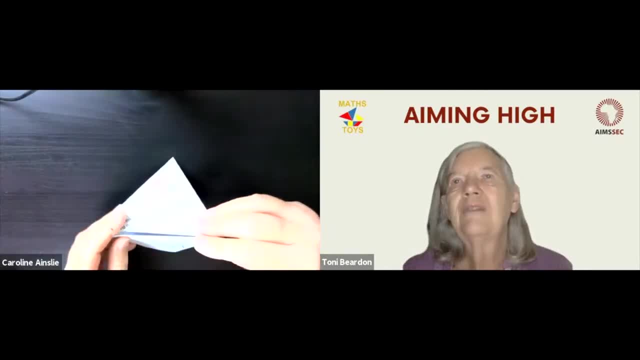 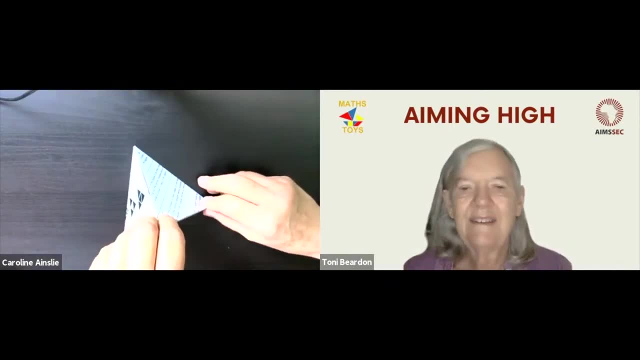 Woo-hoo, You've got your tetrahedron. Isn't that beautiful? It is beautiful And all the edges. This is a regular tetrahedron, All the edges. That's a tetrahedron- Four faces. 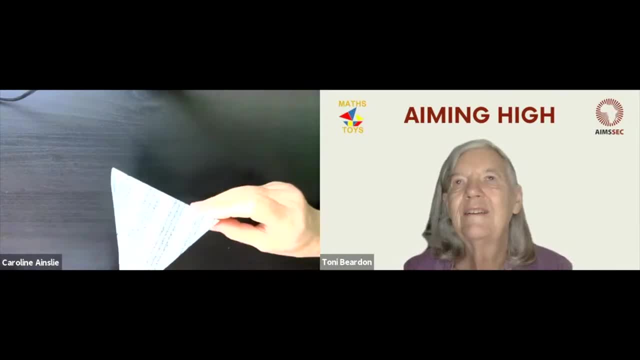 And all the edges are the same length, All the faces are the same size, Every vertex has the same number of of triangles, which means that it's a platonic solid. It's a regular polyhedron, And the beauty of this is 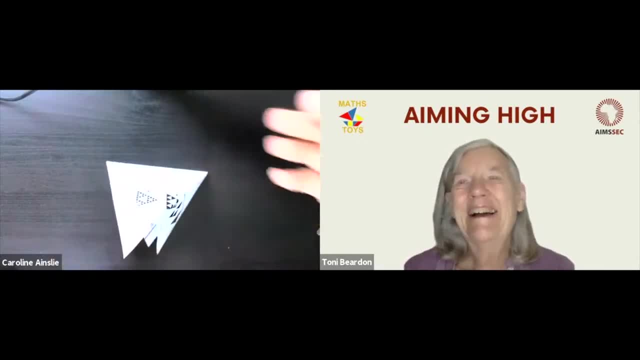 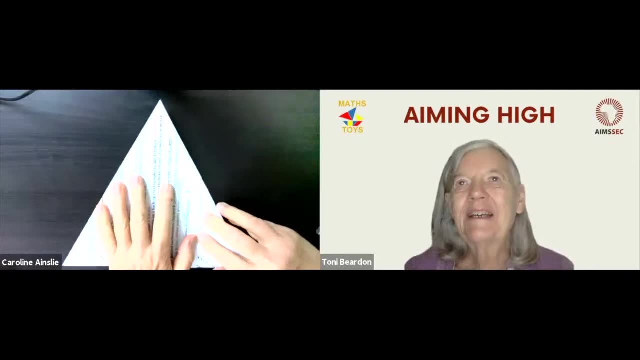 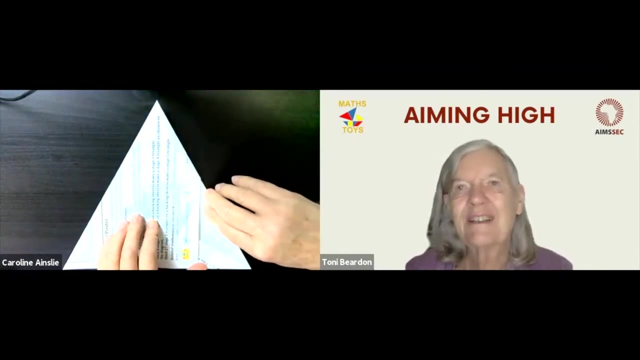 it's so easy to do, It's really easy. So unfold it, Caroline, because now we've really got to look at it a bit more critically. I think we're all convinced that it's angles of 60 and they're equilateral triangles. 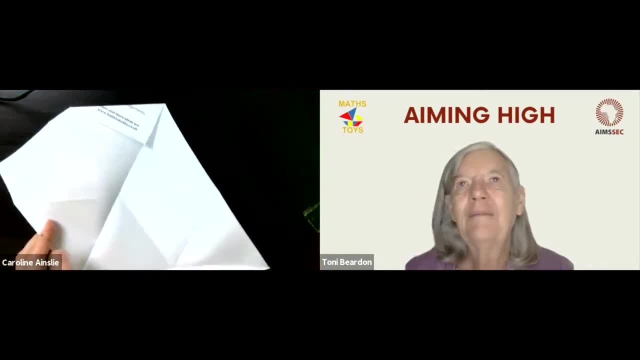 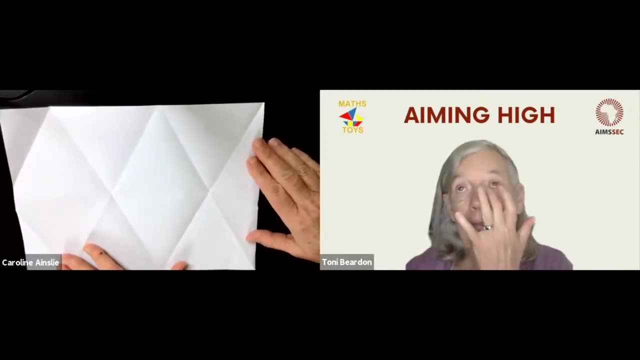 But let's open it right out, OK? Oh, it makes a pretty pattern. Yes, OK, Now just make that first fold. That's the fold. I mean, I'm going to fold it the other way, so that now we've got plain paper. 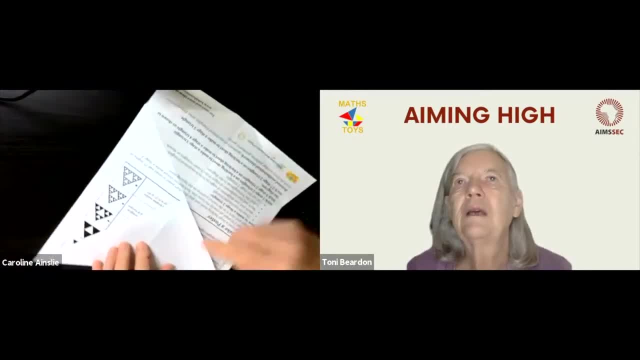 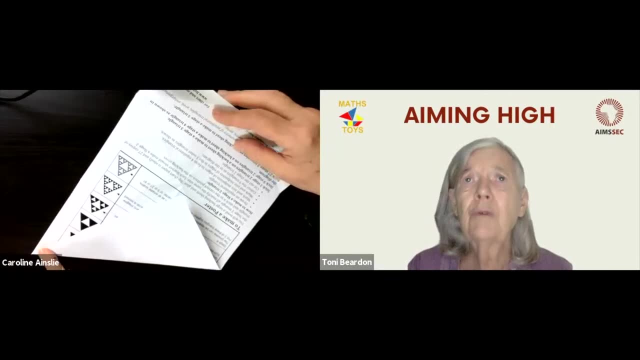 It might help if I have to write something on it. OK, Go ahead, Watch. It's now on the bottom left-hand corner. You have got obviously three angles there Now two of them are on top of each other. 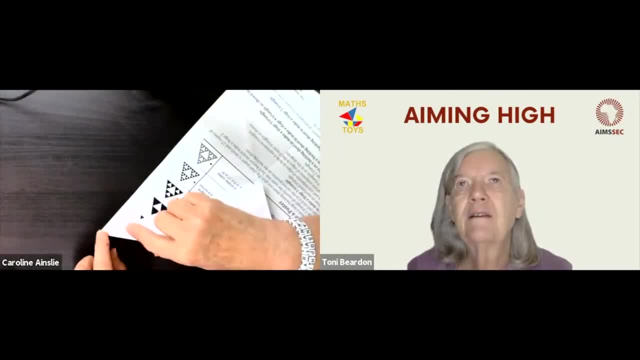 Aren't they? Yes, So we know that, whatever that angle is, the one underneath is identical, because we've got that, We've got. Is it a similar triangle? No, What was it? One of these identical, congruent triangles? 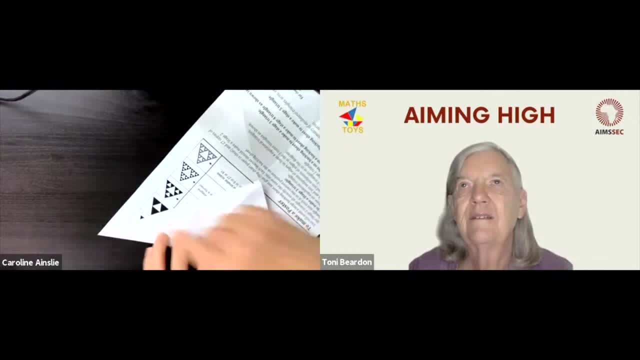 So I'm making a congruent triangle by placing this triangle on top, and whatever is underneath is identical. obviously, Yes. Now Caroline, make another fold that goes through that That corner, So that you have got three triangles on top of each other. 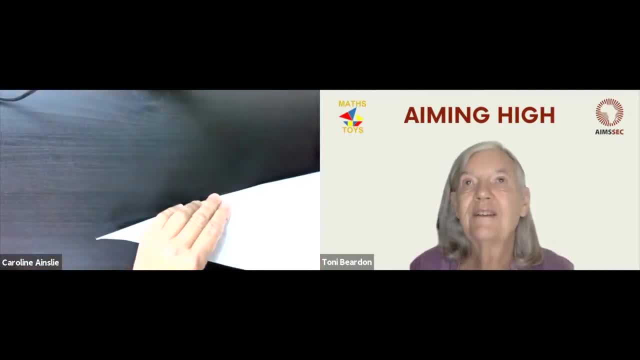 Oh, OK, Like I did with the tetrahedron, Here we go. Yes, Now those The corner there that Caroline's showing us. we have got three angles on top of each other and they're all the same OK. 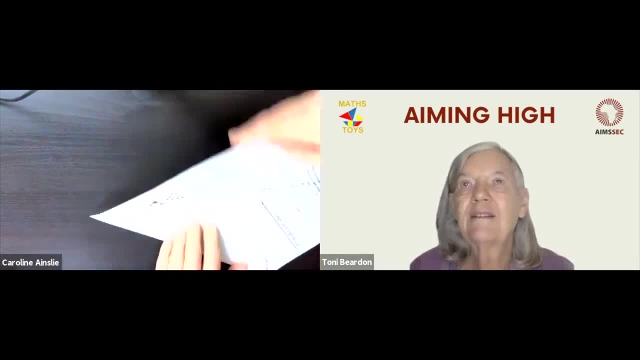 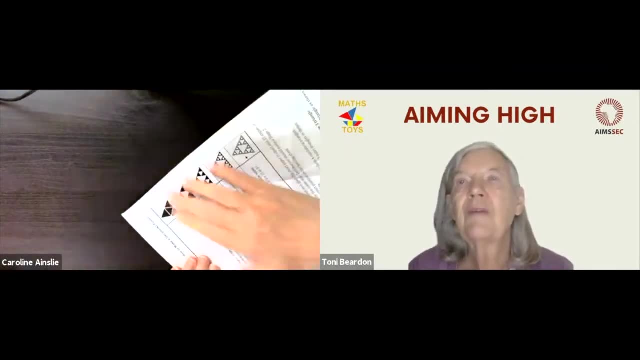 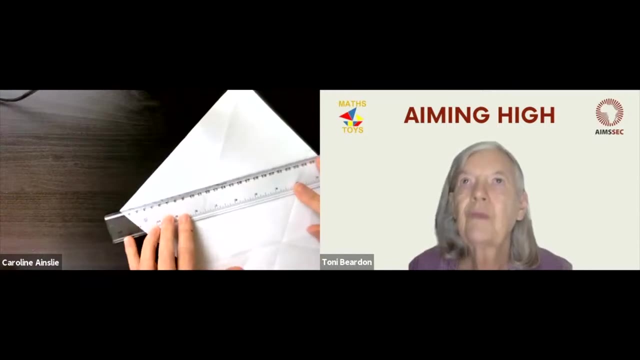 Now open it out, Caroline, And So each of the angles, And, in fact, Caroline, could you draw the? Could you draw the dotted line on the paper to show us? Yes, I'm going, I'm just turning it over. 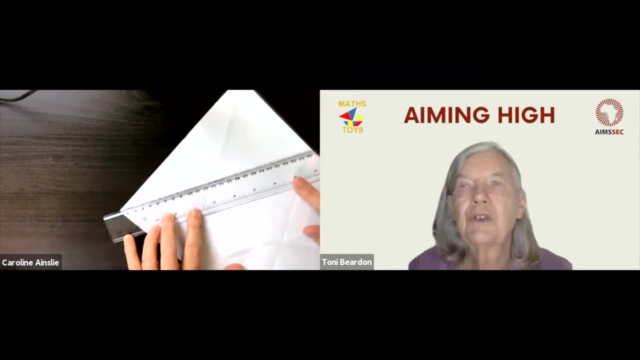 so we can see it a bit better. Yes, Just a dotted line. Remember what I said, that this pen is a thick pen, so use a pencil yourselves. It's, It's more, It's much more precise, It's hard to see. 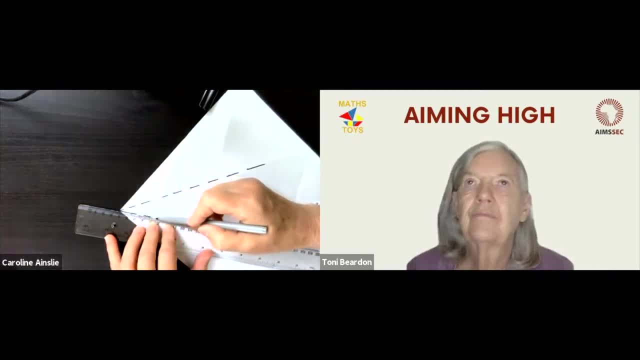 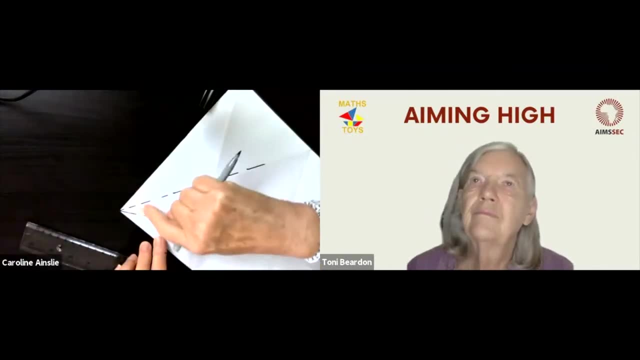 Here we go, Whoops, OK, You're telling me that. Well, we knew that two of those angles were the same, because they, Well they are. They must all be the same, because we folded them over onto each other and they were all. 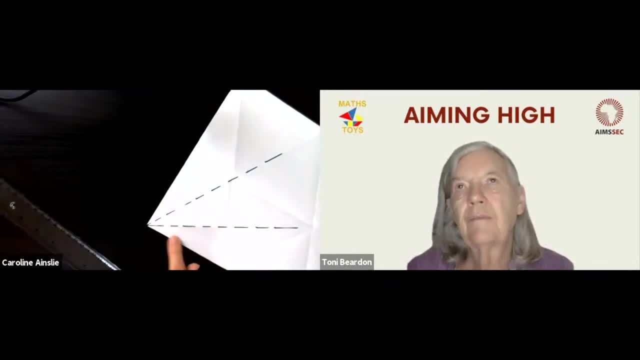 They were just sitting on top of each other. Yes, and they add up to: Well, we know that's 90 degrees. Yes, It's a standard piece of paper, So, And they're all the same. so it's 90 divided by 3.. 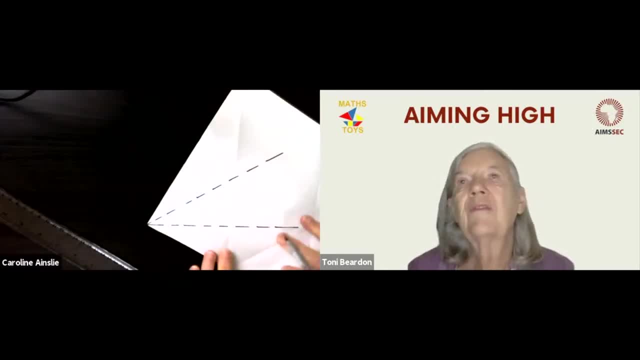 30 degrees, 30 degrees each, And then the two of them make the 60,, which is what we were claiming, Which was what our original claim, which is- Make sure I get the right one here, That one. So it's. 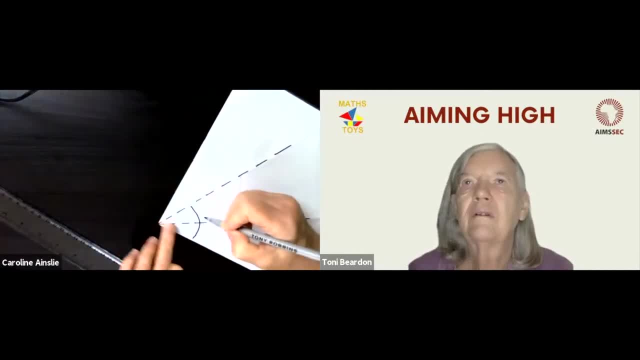 This here is 60 degrees. That was our original 60 degrees, which is what you said it was. Yes, This is 30.. Yes, And of course, this is as we said, it's not a lesson, so we're not going to go on about this any longer, but 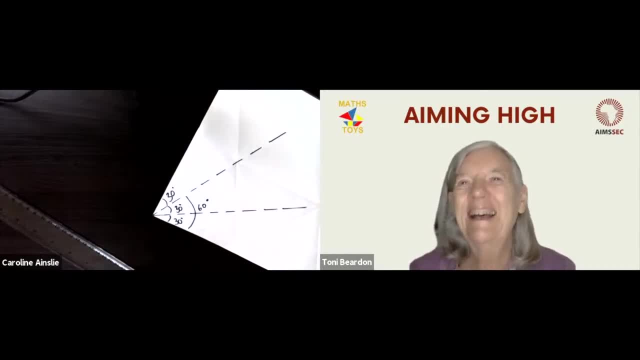 No, but it's super exciting that all you're doing is folding paper and, hey presto, you just have to have a few basic things like know that a right angle is 90 degrees, and things like that. Yes, yes, Lovely. 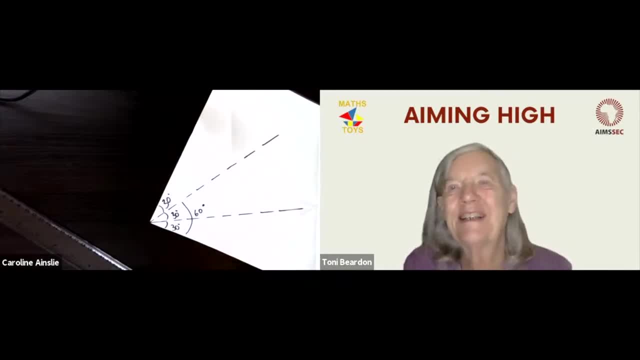 And you can. Obviously you can- get into ideas like congruent triangles and prove that you have got the condition for congruency, which is one of the things they teach about in school and you've got to. Children have got to be able to write it down in the right way. 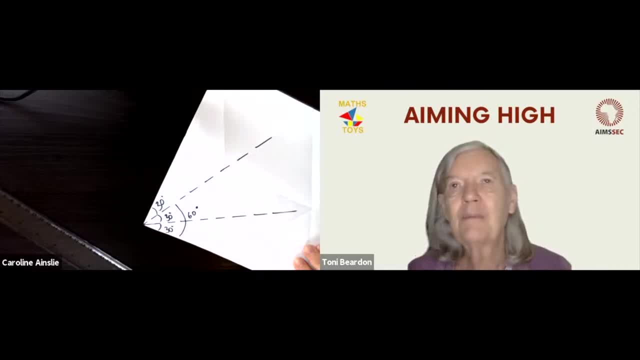 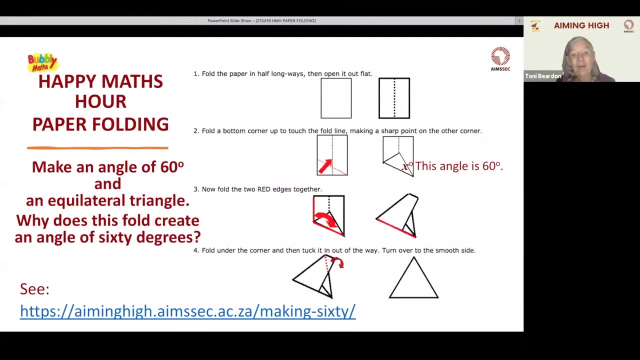 But it's so easy with the paper that it'll be clear to anybody who does it this way what is happening, and this proof is a nice easy proof. So that's a very Another, very rich activity. Now go to the Aiming High website. 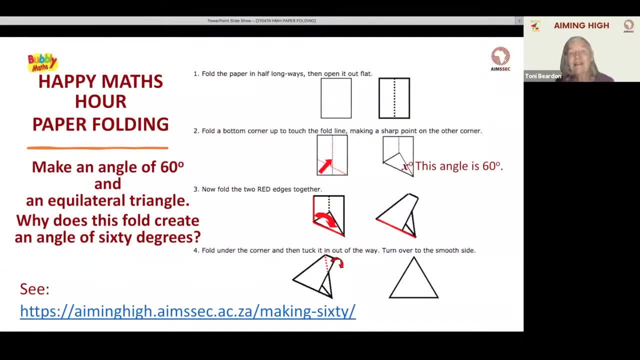 and you'll find the Making 60 activity will give lots of suggestions for teachers using this activity. It's a simple activity. It makes maths fun, It makes geometry easy. So you see there the illustrations of what Caroline did with just an ordinary sheet of paper. 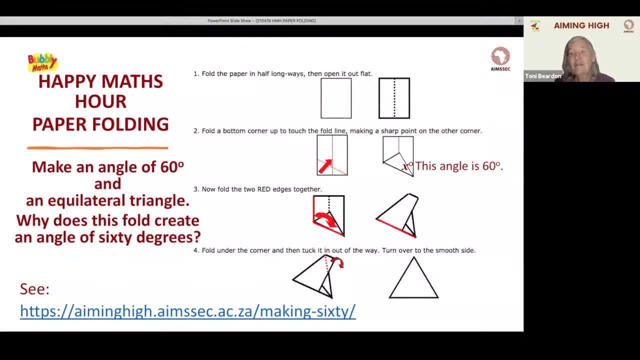 and making an equilateral triangle, then making a tetrahedron and then proving some geometry, Some geometry facts, Just using paper folding, and reasoning about showing congruent triangles and reasoning about the angles in the triangles. I would agree, Very enjoyable. 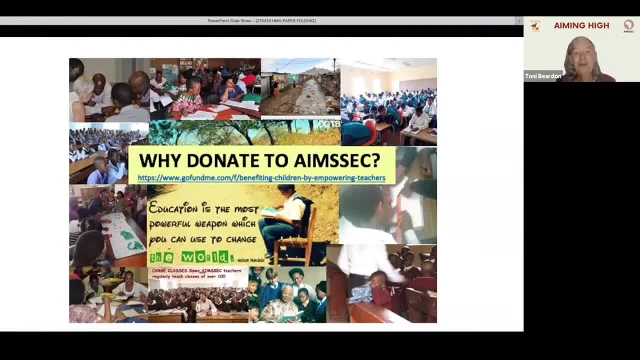 I love that, Thank you. Now this picture shows you a little bit about AIMSEC and why I am involved, and have been for a while- with working in South Africa, another African country, because I think that education is the most powerful weapon which you can use to change the world. 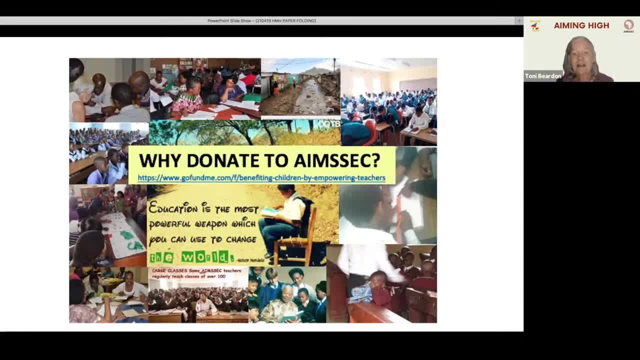 That's what Mandela. Nelson Mandela said, And there you'll see at the bottom a picture of him reading with some children. And I want to change children's lives, but they can't do it. I started work with hundreds of teachers and they are the important people. 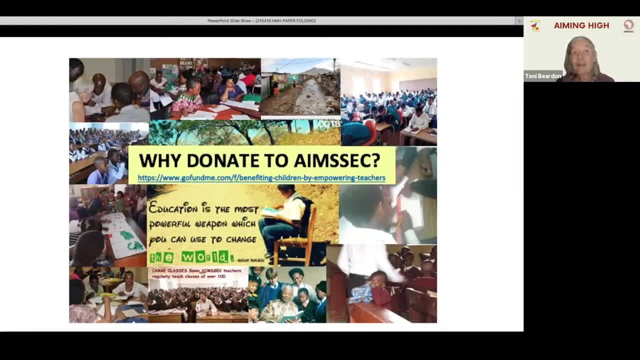 They're changing the lives of those children who, with a better education, should have better life chances and opportunities for a better life. And you see some of the classes there, The top right hand, you see that enormous class. That's very common that teachers are working. 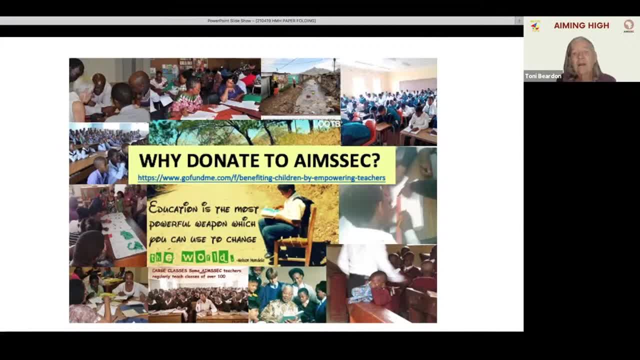 with huge classes there, And just on the top, just to the right of centre, you'll see a village street there. Now, that's where I live and where Caroline's father lives in Fishook- Fishook on the Cape Peninsula. When I say it's where we live, 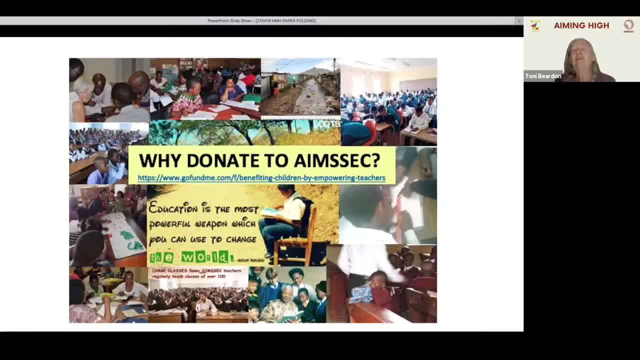 it's part of Fishook. Actually I don't live on that street, but where I live is only about 20, 25 minutes, maybe half an hour at most, to walk from my part of Fishook to that part of Fishook.